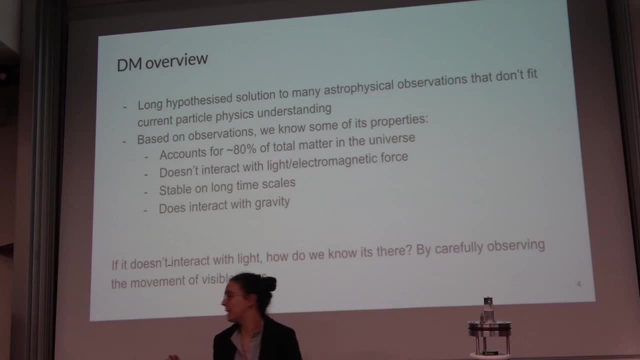 ratio of empty seats to people would probably be about the same as matter to dark matter. It doesn't interact with light or the electromagnetic force, depending on how technical you want to get. It's stable on long timescales so it doesn't decay away like radioactive material. 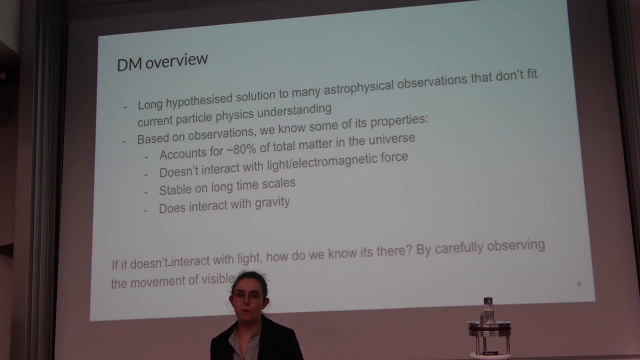 But it does interact with gravity, which is key to how we know that it's actually there. However, the big question is: if it doesn't interact with light, which is why it's very creatively called dark matter, then how do we actually know that it's there? I'll go. 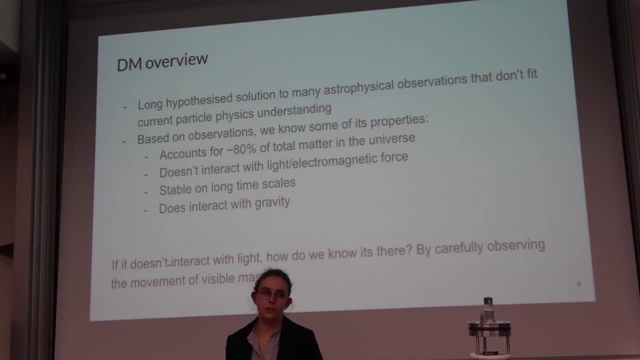 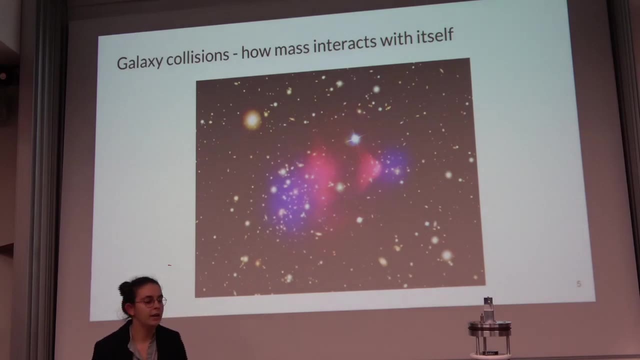 through kind of the three main ways that we know that it's there, by looking at how it can interact with mass. All right, So the first thing is galactic collision, So how mass interacts with itself. This is a very famous picture and if you go on to keep studying, 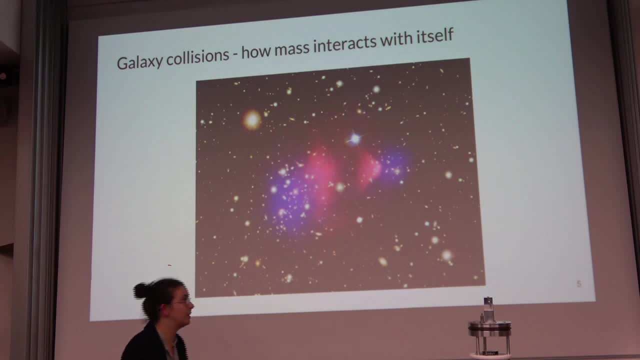 physics, in particular particle physics. I promise you this is not the last time you'll see it. This is called the bullet cluster And essentially what's happened is you've had one galaxy come through here and collide with another. So in pink we have the distribution. 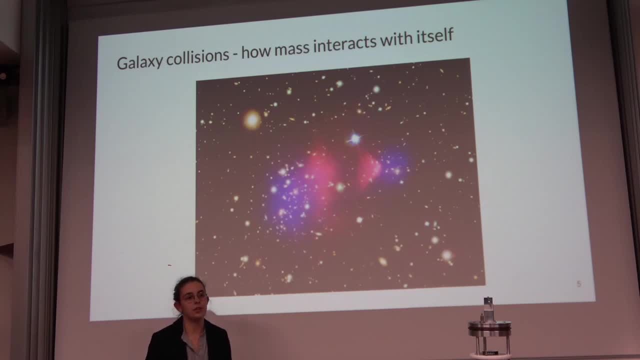 of mass of gas, So most of the galaxy is actually made up of hot hydrogen and helium gases. These are mapped in red here And this is how we know there's been a collision, because you can see that something's shot through here like a bullet In purple. however, we've 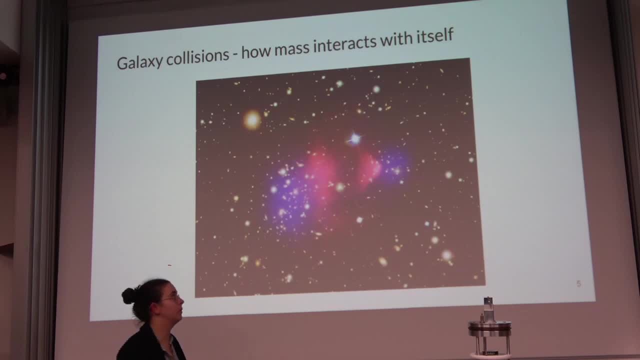 mapped the center of the mass of the galaxies, which we can tell based on how the visible stars and things, And the fact that the gas which actually makes up most of the galaxies doesn't overlap with where we know the mass is, tells us that there's a whole bunch of extra matter there. 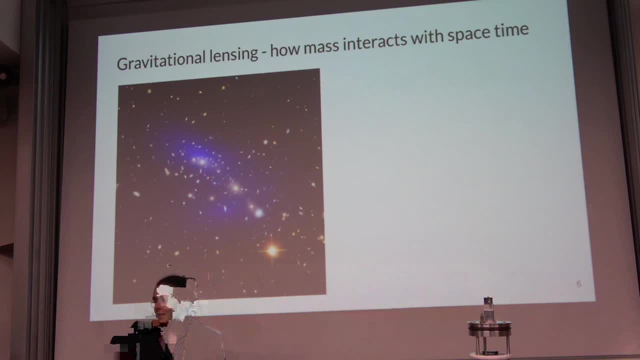 that we can't see. The next thing is gravitational lensing, which is about how mass interacts with something called space-time. So if you've done any kind of special relativity, you'll know that our universe is made out of a space-time fabric that, I like to say, is a little bit like a. 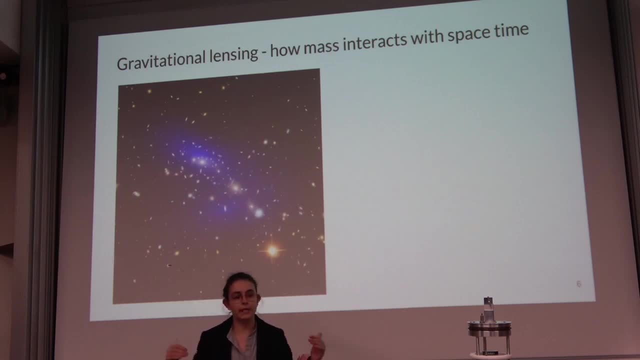 trampoline. And when you put a heavy mass on a trampoline, it's going to bend it. And in the same way, if we have masses like stars and galaxies in space-time, they're going to bend it too. So you can see. 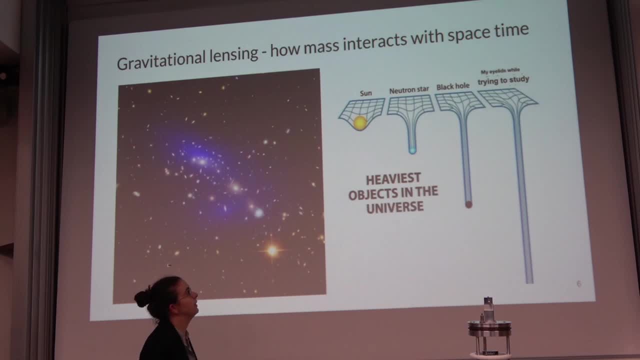 here is a plot of some of the heaviest objects in the universe that are bending space-time: The sun, a neutron star, a black hole, my eyes when I'm trying to write my thesis, And each of these guys are going to be bending our space-time trampoline more than others. 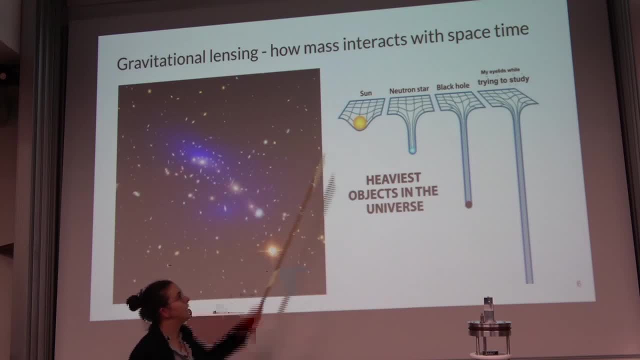 And as they do this, when light comes in and it moves around it, it essentially is getting smeared. So you can see this in this picture here. So you can- I don't know if you guys can see from where you are, but there's basically a whole bunch of stars that are kind of being 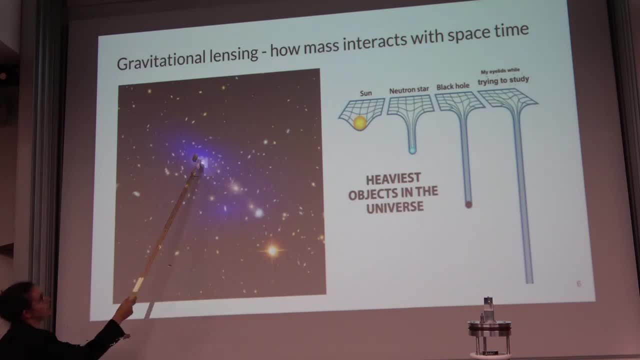 and galaxies- sorry- that are being smeared out like this, And that's happening because there's this really big galaxy in the middle that's smearing them in this lensing way, And even though there's a galaxy in the center. here we also see this happening when there's. 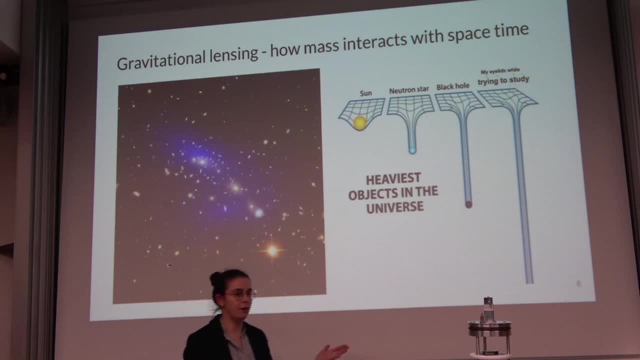 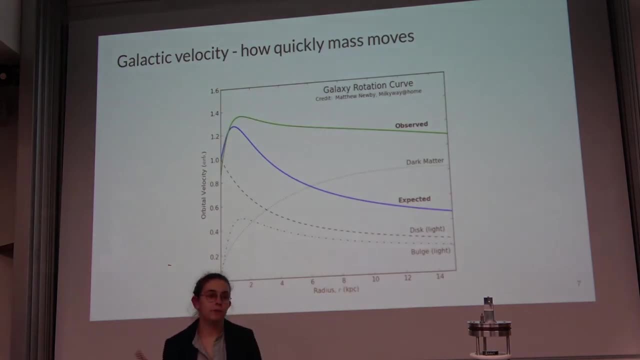 nothing in the middle, So it looks like there's no mass, but all the stars around it are behaving as if there is, So again, mass that we can't see- Finally, we come to the galactic velocity. So in the same way- I don't know if you guys. 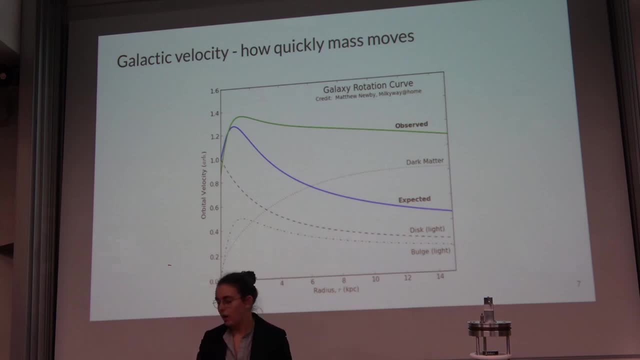 have ever spun a yo-yo or a mass on a string, but basically, the closer it is to your hand, the faster you have to bend it, And so you can see that there's a whole bunch of stars that are being smeared out, but all the stars around it are behaving as if there's nothing. 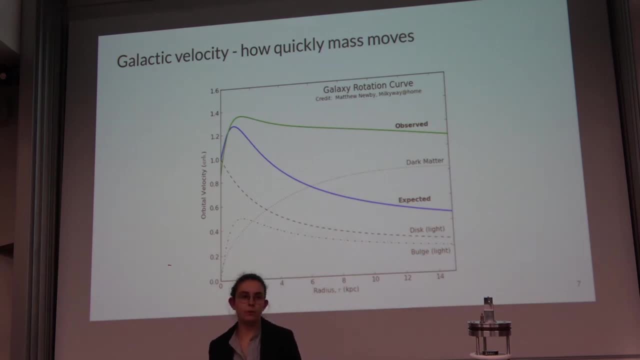 in the middle. So again, mass that we can't see. So again mass that we can't see. So exactly the same principle applies to stars within a galaxy. The further out they are from the galaxy, the slower they should move. So we expect them to follow this kind of curve. 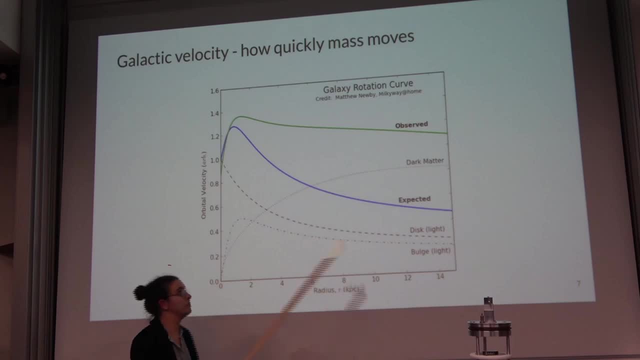 So as they get further out, they get slower. However, what we've actually observed is they stay pretty much the same speed, no matter where they are, which means that there's not some kind of big clump of mass at the center of the galaxy. Instead, it's being evenly. 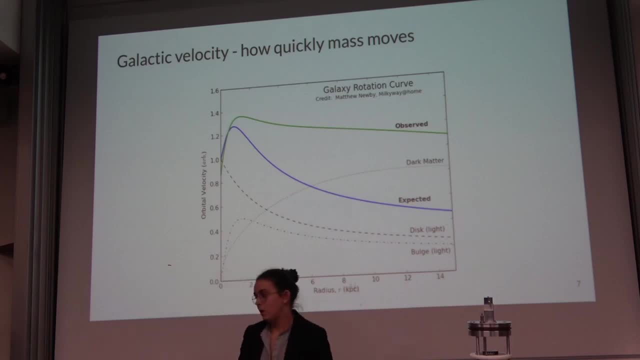 distributed, which is not what we see when we look at the stars. So, basically, these three pieces of evidence are being smeared out and they're being smeared out, and they're being smeared out and they're being smeared out. So these three pieces of evidence tell: 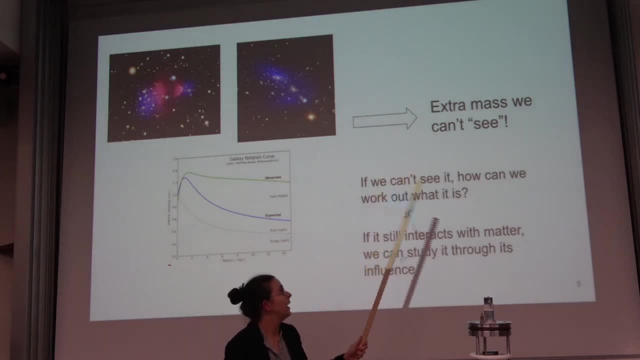 us that there has to be extra mass that we can't see within the universe. And again, as I said before, if we can't see it, how can we work out what it is? So, if it interacts with matter, we study it through its influence. We knew that it was there based on looking. 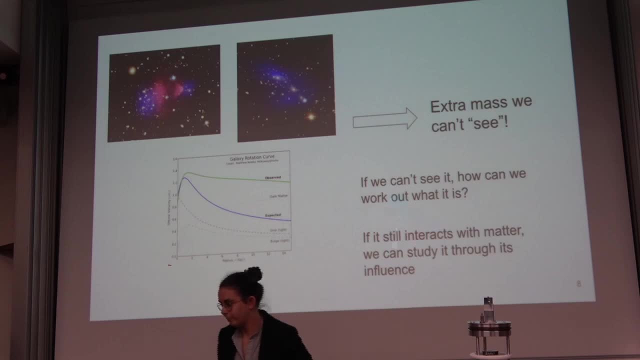 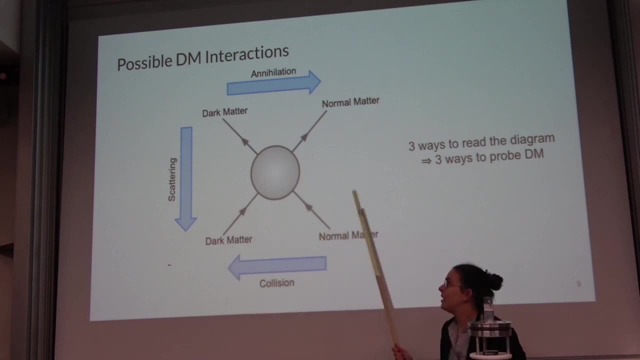 at how it influenced other things and we're going to study it in exactly the same way. So this is kind of a standard – spin it around – this is kind of a standard drawing of how we write interactions where we don't know what's happening. We're going to have a dark matter particle coming in, a normal matter particle coming out, and then we're going to have a dark matter particle coming in, and then we're going to have a normal matter particle coming out, and then we're going to have a normal matter particle coming. 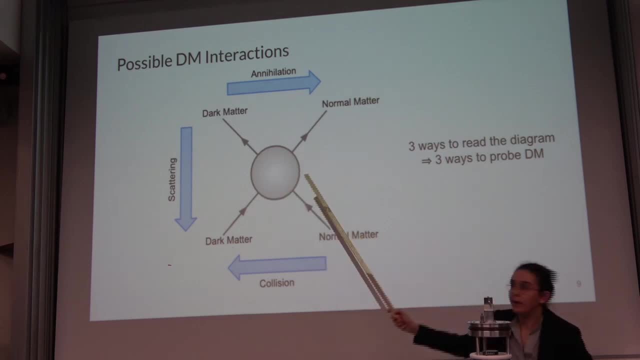 in and then we're going to have a normal matter particle coming in. we don't know what happens. we just put a giant blob and then we're going to say, okay, we've got normal matter and dark matter coming out. There's basically three ways that you can. 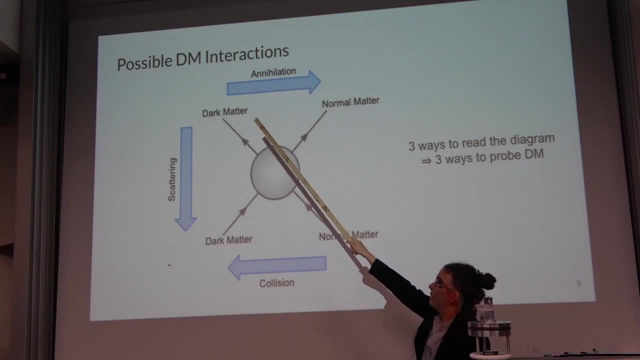 read this diagram. You can start from this side and say, okay, I'm going to start with two dark matter particles. they meet up, something happens and they turn into two normal matter particles. I can read it up and down where I say that, okay, I've got a dark matter. 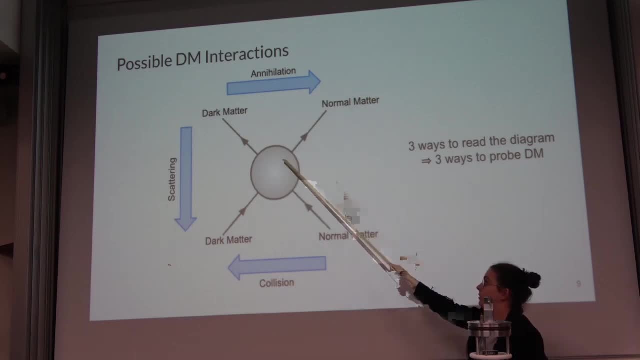 particle coming in, it does something with a normal matter particle and then they both go off their separate ways. Or I can read it this way and say: okay, I've got two normal particles coming in And it out-spits two dark matter particles. So these are three different ways to read. 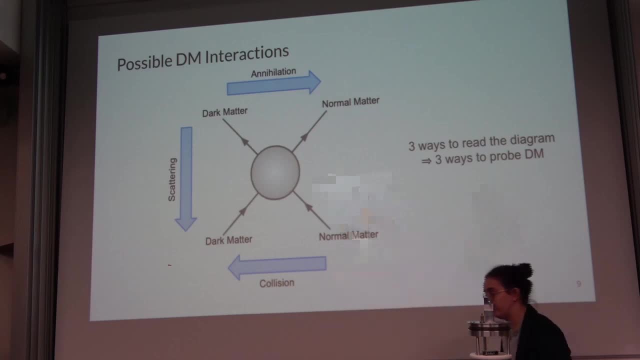 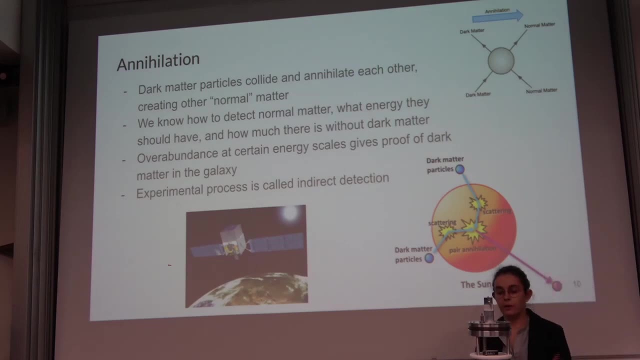 the diagram, which means that there's three different ways that you can probe dark matter. I'll go through each of those quickly now. So the first one is annihilation, where you have two dark matter particles destroying each other and out-spits, something that we 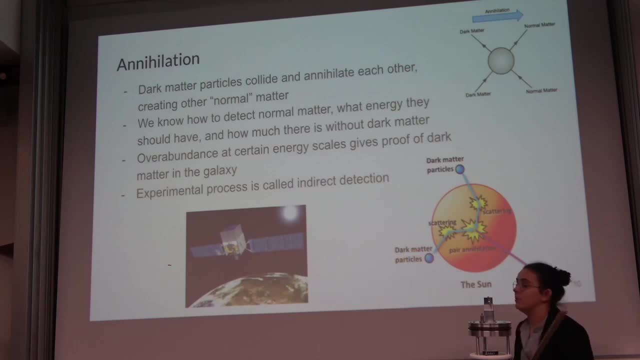 know how to detect. This is particularly powerful because, obviously, if it's regular matter, we have already designed a whole bunch of experiments on Earth that can see this. Because it's regular matter, we also know very well how much there should be if there was no. 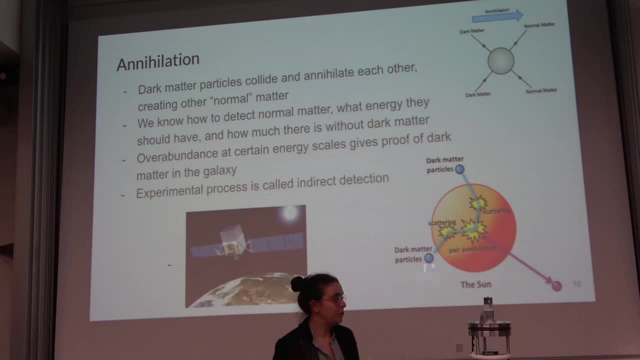 dark matter and we know how much energy they should have. So what we do is we put a whole bunch of telescopes like this guy out here called Fermilat, which is pointing towards the sun, And we look very carefully at what's coming from the sun and see if we 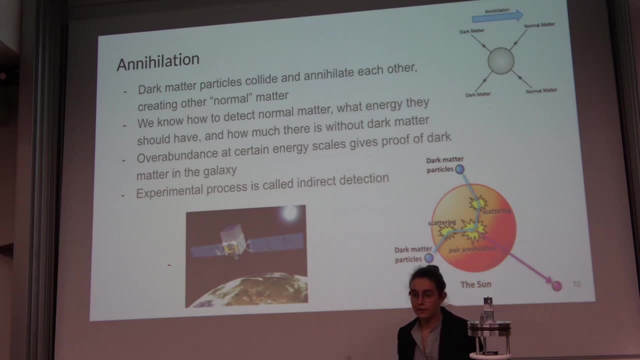 can spot any overabundances at certain energies. If we see some, then we know that this must be attributed to dark matter within our galaxy. So this experimental process is called indirect detection, because you're not actually observing any dark matter, you're observing its annihilation. 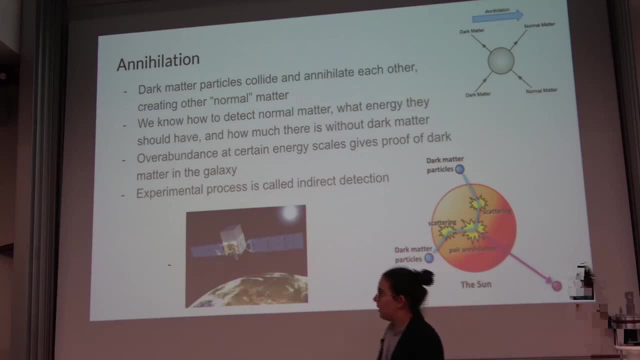 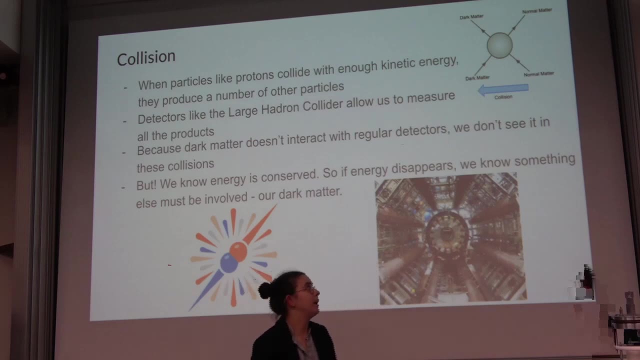 Sorry, I'll just move that so it's a bit easier for people to see, All right. next We have collision, which is exactly the opposite process of annihilation. Instead of dark matter, annihilating it's our regular matter. So this is a picture of 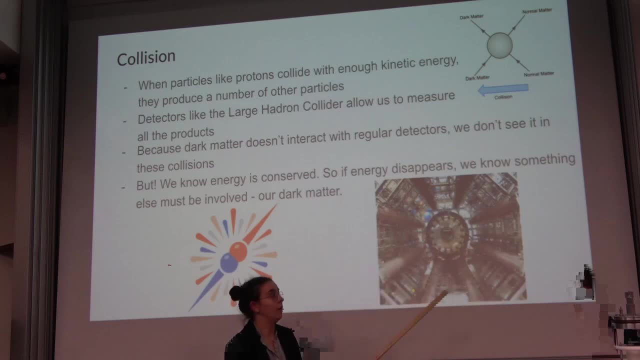 probably one of the most famous physics experiments in the world, called the Large Hadron Collider. This guy basically collides these regular particles at massive speeds with huge amounts of energy to produce a whole bunch of other particles. So you can kind of imagine it. 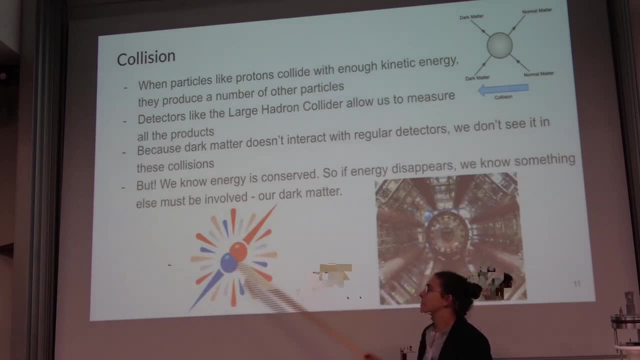 obviously a very simplistic diagram here, But we have our blue and orange particles colliding and then producing a whole bunch of other different colored ones where you can kind of imagine that maybe these dark gray ones are dark matter. So there's a possibility. 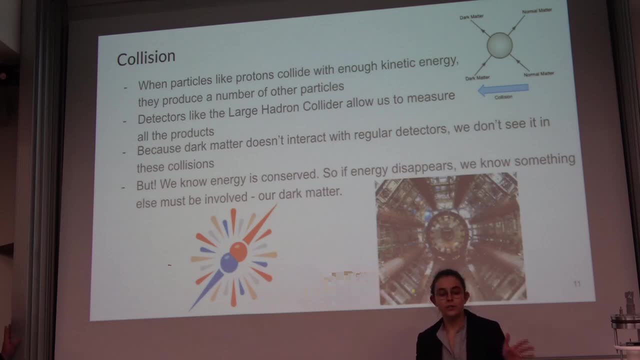 that dark matter can be produced in these interactions. However, as I just said before, dark matter doesn't interact with any of our detectors, because our detectors all use electromagnetic forces in order to observe things. However, we also know that energy is conserved, So 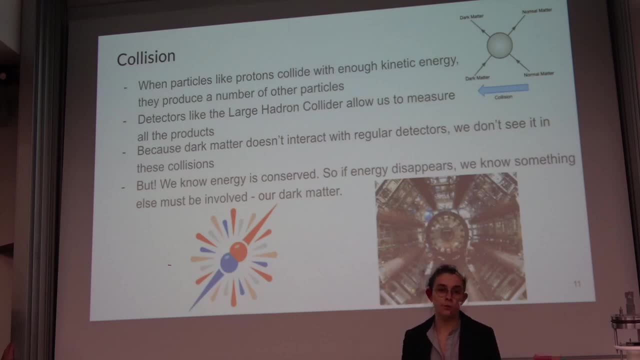 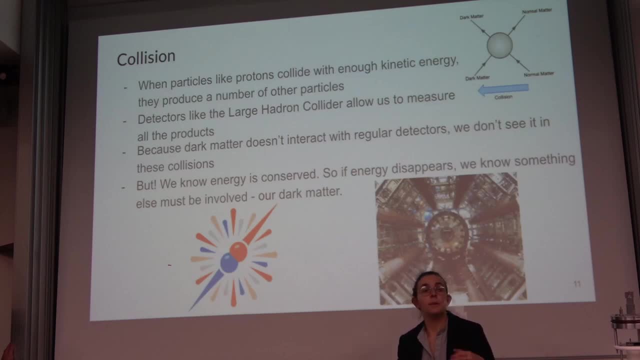 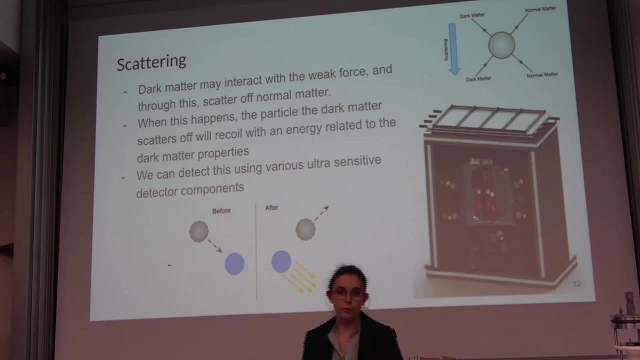 Next up, we have scattering, which is what the SABR experiment that Bill and I both work on does In this case. we're assuming that dark matter and normal matter can interact with each other by kind of bouncing off each other in the same way that you might have. 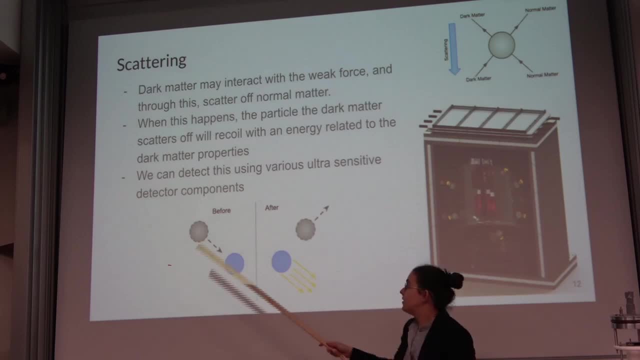 a regular collision. So in this case you have dark matter coming in hitting our target matter particle and then this guy's going to have some energy transferred to it. but because of the dark matter, We can detect the energy of this target particle by 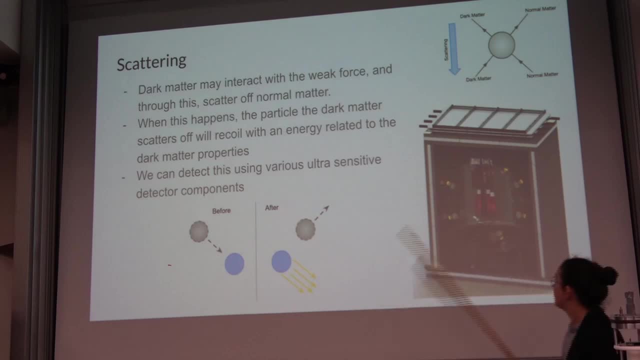 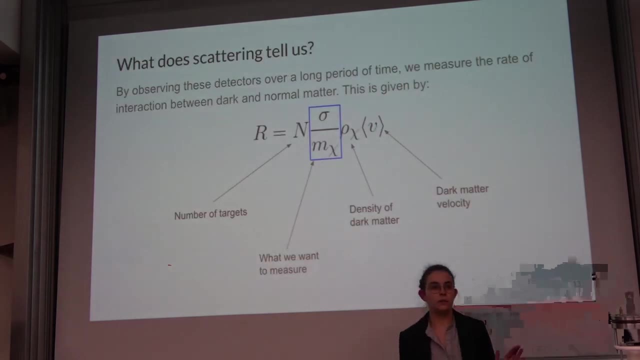 using various ultra-sensitive detector components. So this is a picture of the SABR experiment, and we'll explain this in a lot more detail later. What I'm going to talk about now is what detector scattering actually tells us. So when we go through the physics and all of our understanding of how dark matter could, 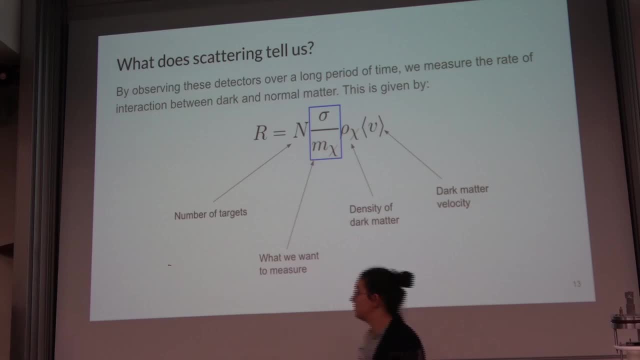 interact. what do we expect to happen inside these detectors? So this expression here basically just gives you the rate of a collision. This one is for dark matter, but you can apply the same kind of principles to work out the rate of collision of anything Like: if I'm walking out into the rain, you can use a 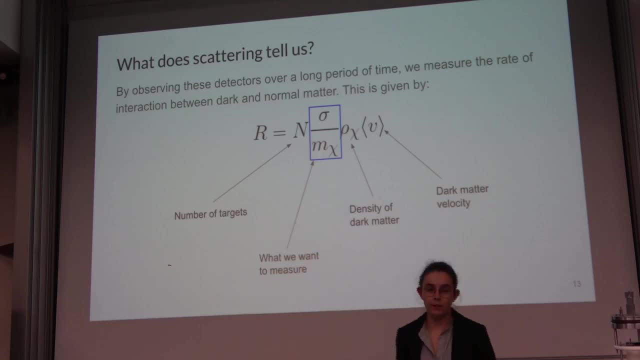 similar thing here. to work out how many rain drops are going to hit me. It depends on the number of targets that you have Some particular properties of dark matter that I'll talk about in a second called the cross-section and the mass. These are what we want to measure The density of 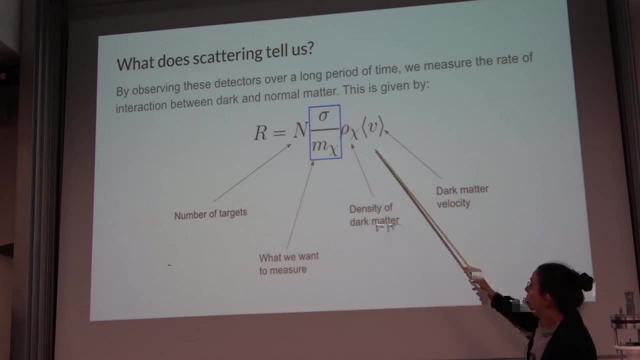 dark matter. so how many dark matter particles are hitting me, and then how quickly the dark matter is moving. These two things we can pull from astrophysical observations. This one we set up ourselves. so then all we have to do is put our detector. 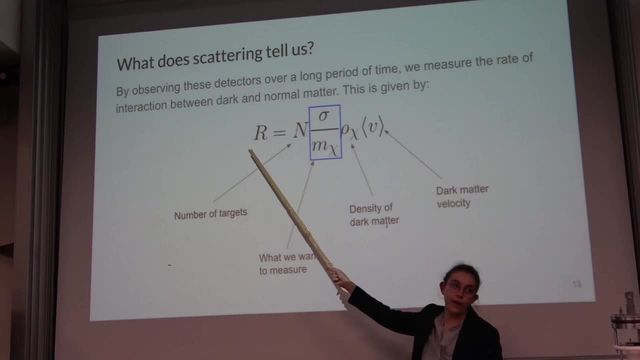 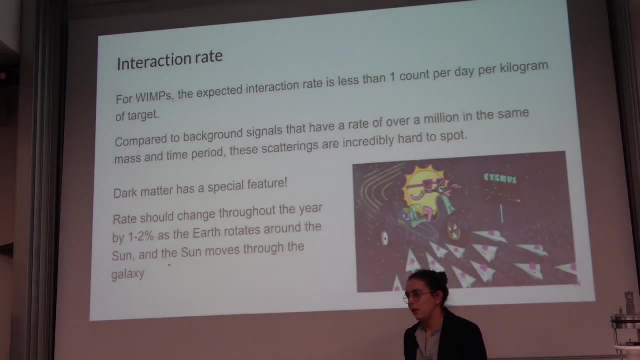 underground wait, observe some interaction rate, so some number of interactions that occur, and then we can calculate this value just here. So what do we expect this interaction rate to be? There's a whole bunch of different kinds of theories for what dark matter could be, but one of the most popular ones is: 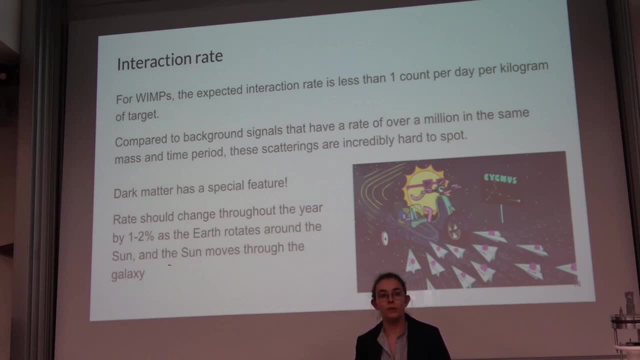 called a WIMP, because physicists are excellent at naming things. It stands for weakly interacting massive particle, because it's a particle that interacts weakly and it has mass. In this case, we expect that they have a particular value of mass and cross-section that is going to give it an 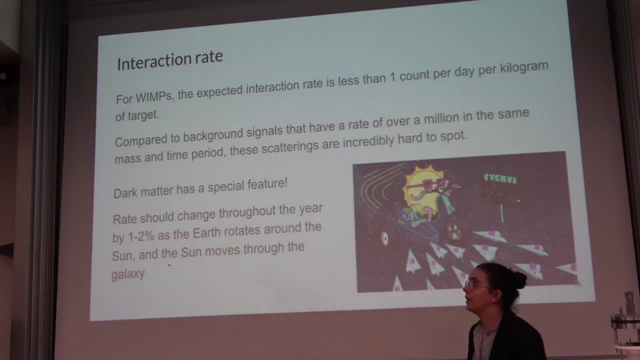 interaction rate that is less than one count per day per kilogram of target. So think about that for a second. If you have like a kilo of flour and this guy could interact with dark matter, you'd only see one count per day. Now I don't. 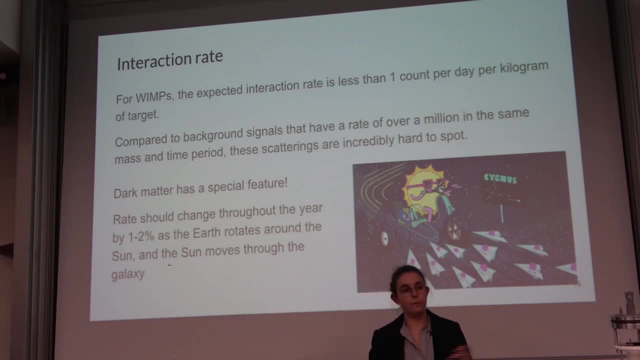 know how much you guys have studied about. you know general radiation or particles that come from the Sun, but we have background signals that have a rate of over a million in the same mass and time period. So you're trying to pick out, quite literally, a needle in a haystack here. a single event over a day compared. 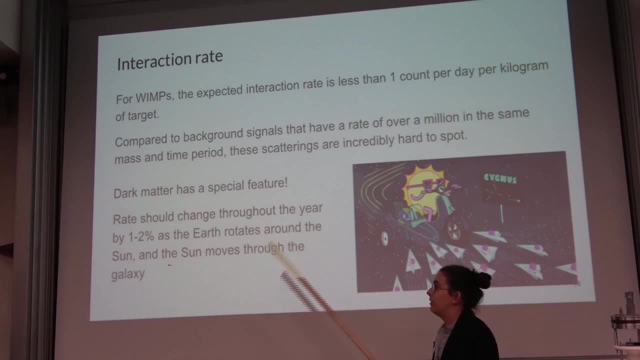 to a million. What we do have a bit of luck with, though, is the fact that dark matter has a really special feature: We expect it to have a modulating rate. Now, this happens because we've got kind of a cartoon version of the Earth in a side. 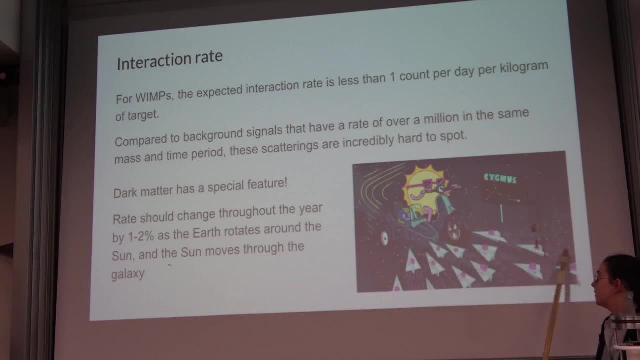 car as the Sun moves through the galaxy and it hits kind of our WIMP flux here Now I hope you all know this could be groundbreaking science here. but the Earth rotates around the Sun. So as the Sun is moving through all these dark matter, 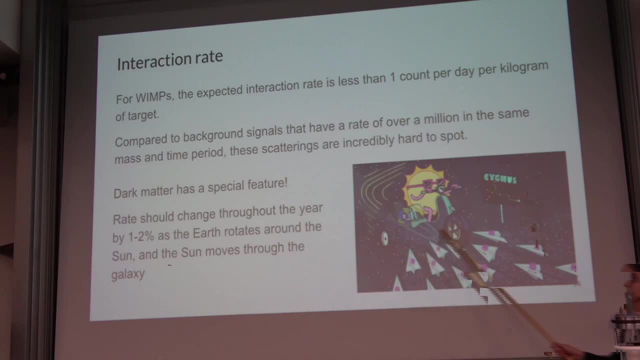 particles. half the time the Earth is traveling with it in this direction and the other half of the time it loops back like that. So that means that the rate is going to change throughout the year by about one to two percent, and we expect to see more events in June than we do in December. So it's a bit of a gift that. 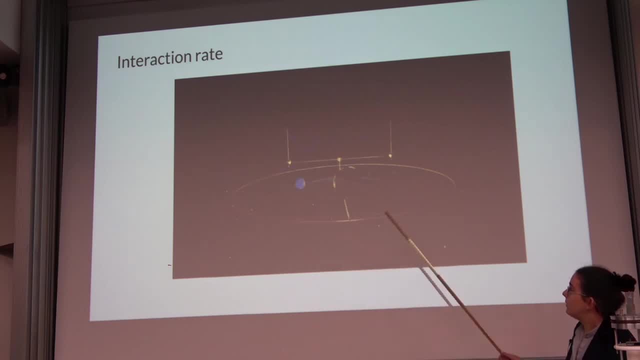 demonstrates us a little bit better. So you can see, here we've got the Sun and the Earth, and as the Earth is traveling kind of on the outer side of the Sun, they're traveling parallel to each other, and when it's on the inside, they're. 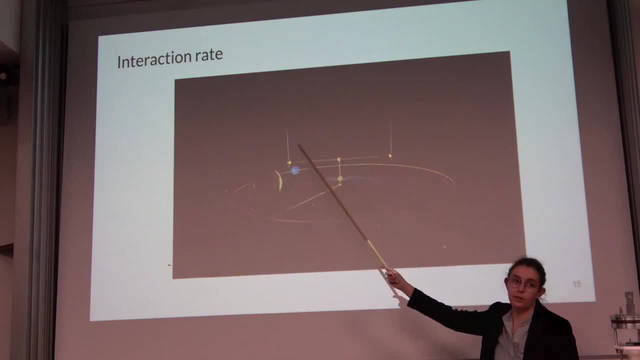 traveling anti-parallel, which is when you get the minimum just here. So you can think about this as the same thing as when you're walking through, walking on the street on a rainy day, If it's really windy and the wind is blowing the rain. 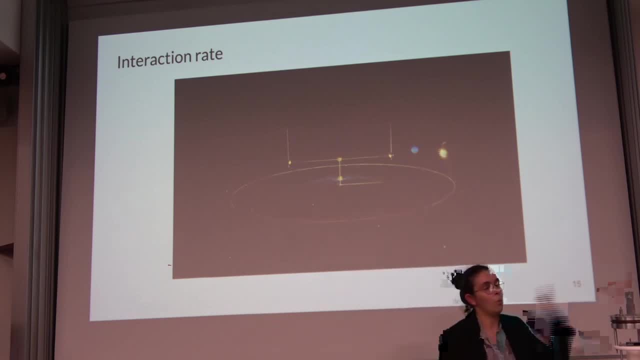 into your face as you're walking, it feels like you're getting a lot more wet because more rain is hitting you. However, if you're walking with your wind, the wind to your back and the rain is coming back on you like this, you're almost out. 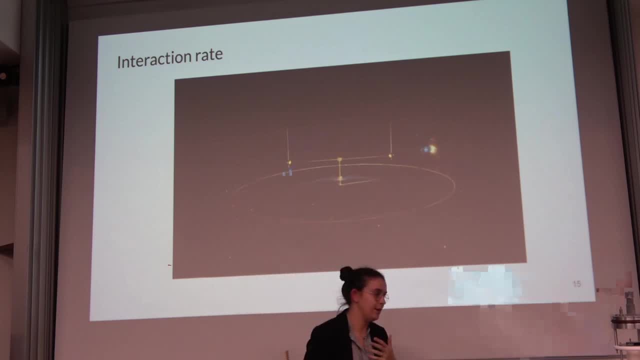 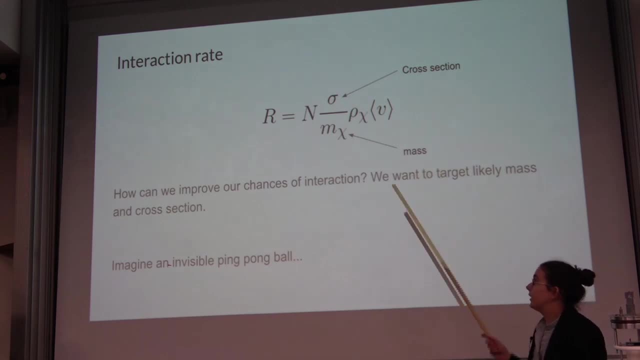 running some of the raindrops, You're not getting as wet and the interaction rate in this case is lower. Alright, so I said I'd explain the cross-section and the mass. These are important because, as I said, the interaction rate is very, very low. but we 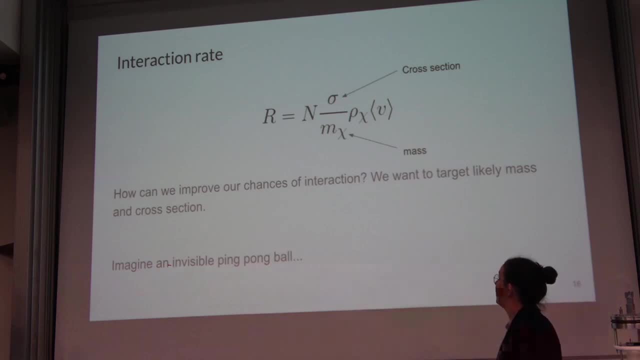 can apply a couple of tricks to increase our chances of seeing an interaction, and we want to target what we think is most likely to be the cross-section and the mass number. So I'm going to talk through a bunch of detector concepts and, in the back of your mind, I want you to imagine that what I'm trying to see is the 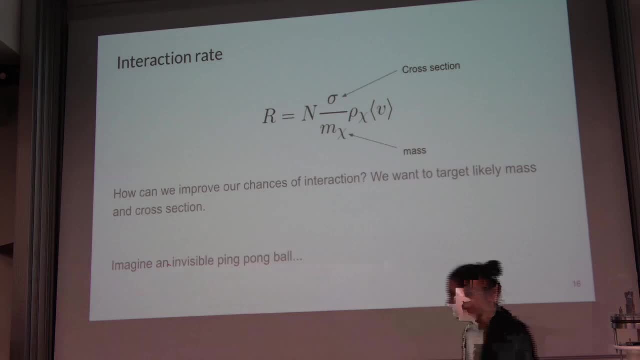 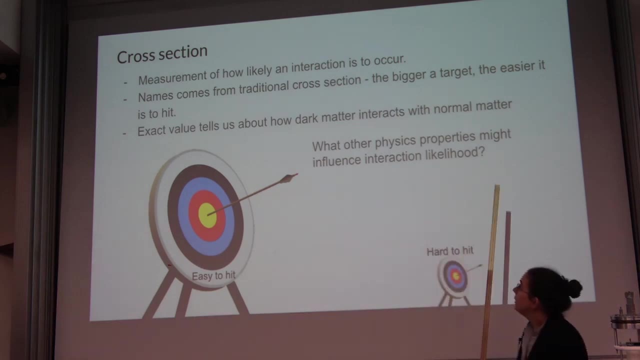 interaction from an invisible ping-pong ball hitting something. Alright. so the cross-section. Finally, after mentioning it like three times, I'm giving you a proper definition. The cross-section is a measurement of how likely an interaction is to occur. The actual name itself is a bit of a hangover from when we were actually trying. 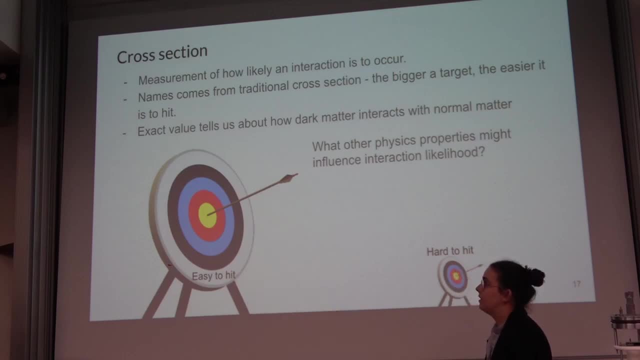 to hit physical targets like a bow and arrow kind of thing, where the physical cross-section and how big it is was a measurement of how easy it is to hit. However, when we think about physics and, in particular, how dark matter might interact with normal matter, there's 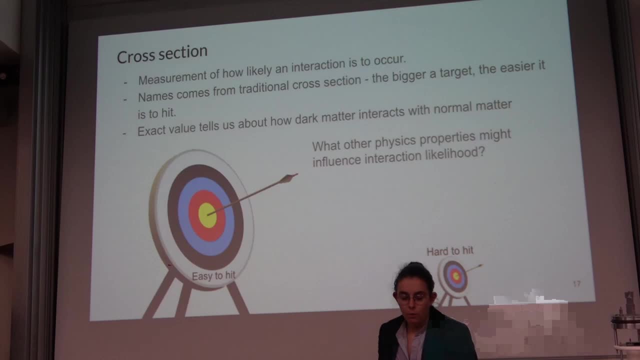 a whole bunch of other things that might come into play. So I mean, there's not a lot of use, so I won't actually throw this out to as a question, but there are some physics processes you've kind of probably come across that might influence. 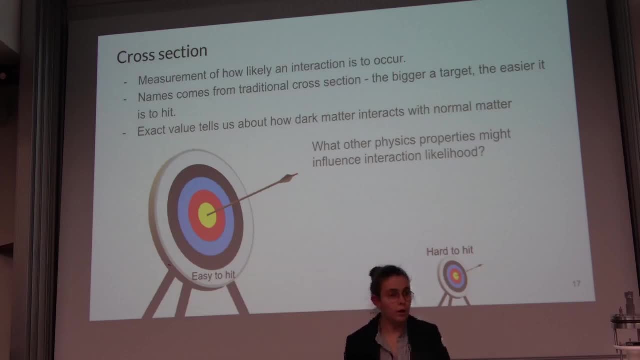 how things interact. So things like if they have an electric charge, if there's any magnetism at play. Another thing that could influence it is how visible the target is. So if I'm standing at the back of the room and I'm trying to throw a ping-pong ball, 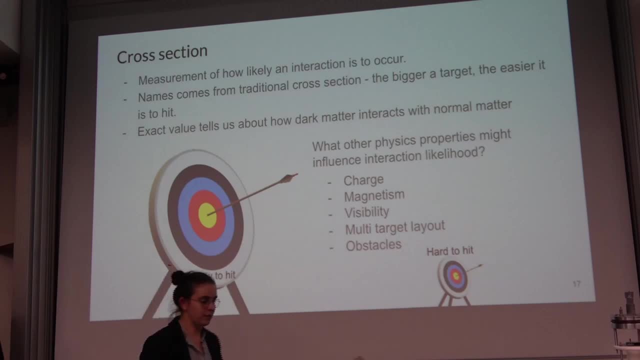 against a whiteboard if I know that my target is a big circle, but the circle is white and it's stuck onto the whiteboard. it's going to be hard to see If there's a big black circle that I'm trying to hit with my ping-pong ball. it's going to be a lot easier You. 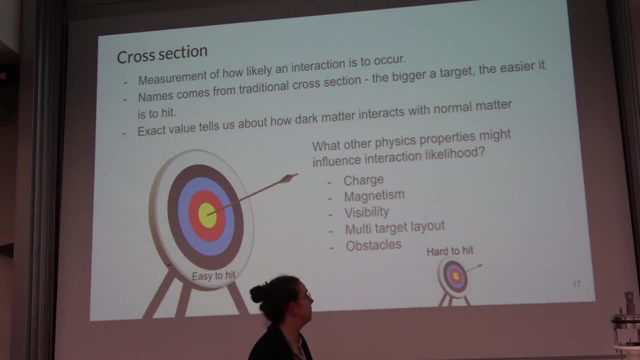 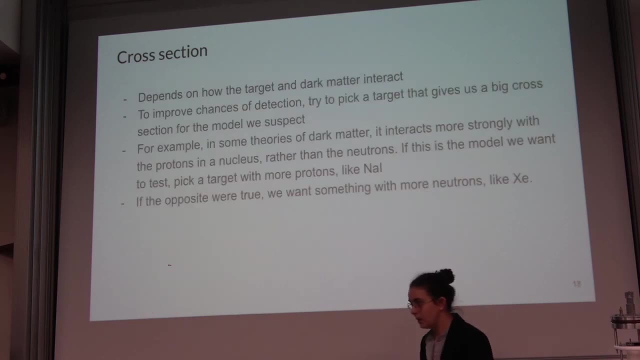 know how many targets are there. If there's more targets, it's going to be easier for me to hit something. Are there any obstacles between me and my target? These are all things that influence the value of a cross-section for an interaction. 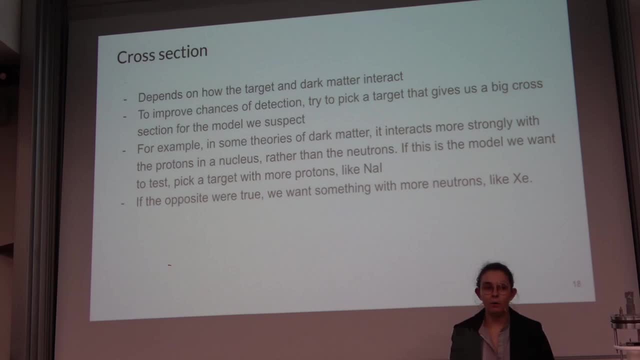 So the cross-section in particular is going to depend on how exactly the target and the dark matter are interacting with each other. This is where it gets very mathsy and physics-y, So I'm just going to try and leave it at that. But basically, to improve the chances of your interaction, you want to build a detector. 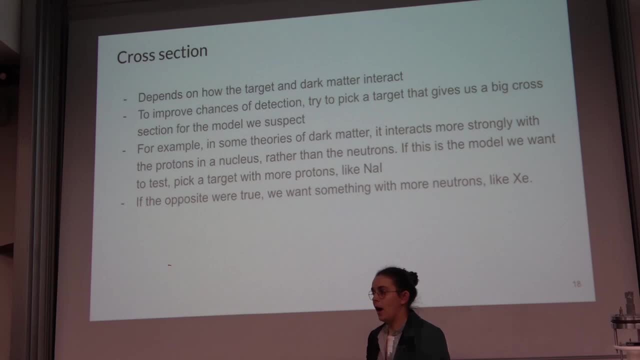 that's likely to have a very high cross-section And by targeting the model that you think is causing the interaction to occur. So, for example, I'm sure you guys have heard about protons and neutrons making up a nucleus. Some models of dark matter tell us that dark 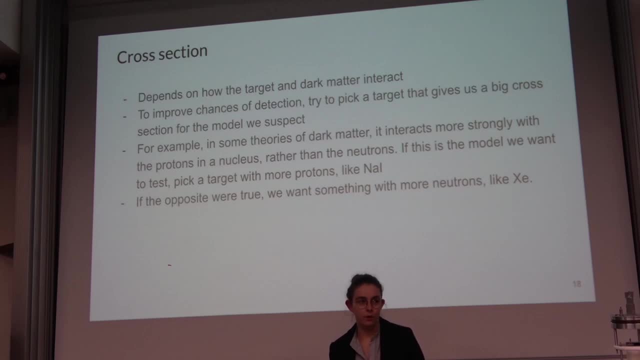 matter is more likely to interact with a neutron than it is with a proton. If that was the case, we would want to pick a target that has a lot more neutrons, like xenon. Conversely, you might have a dark matter model that interacts more with protons than neutrons. so we pick. 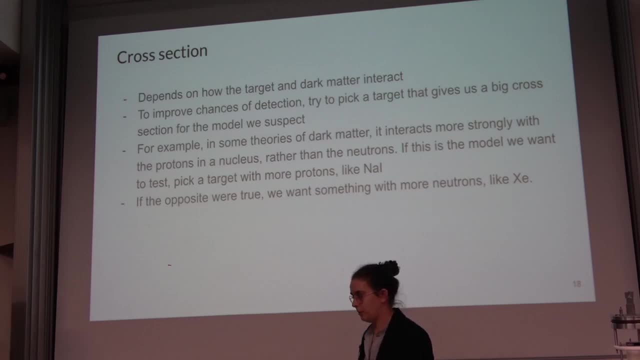 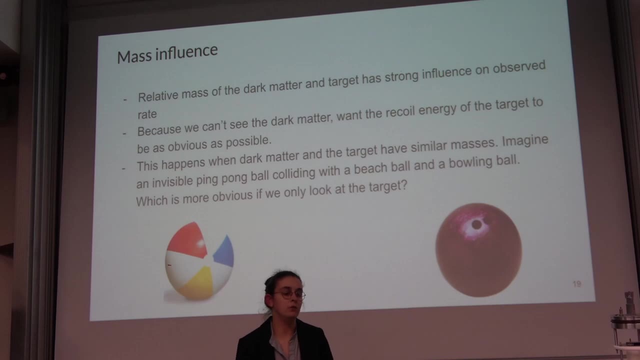 a target that has more neutrons. The second thing that we can kind of manipulate is the influence of the mass. So the relative mass of our target and our dark matter is going to have a really big influence on what we actually see. So imagine if I'm trying to hit a bowling ball and a beach ball with my invisible ping. 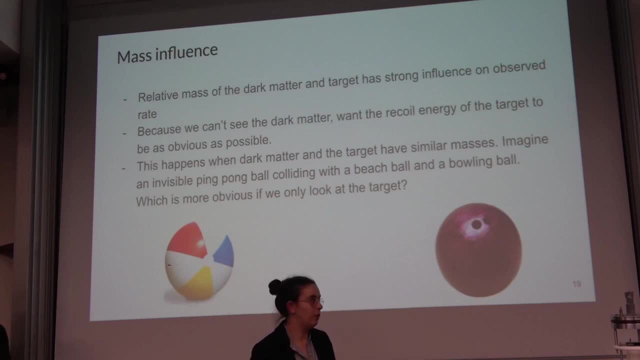 pong ball. They've both got the same size, so they've got the same physical cross-section. But if you can only see what the target is, if I throw a ping pong ball at a bowling ball, is the bowling ball going to move? No, If I pick a bowling ball, it's going to move. 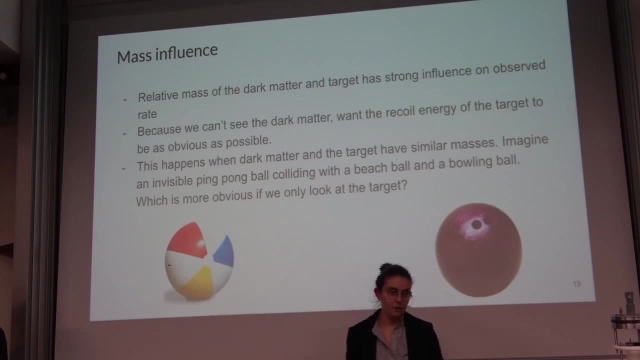 If I peg it at a beach ball, is the beach ball going to move? Yeah, So if the only thing you can see is a target, an interaction with a beach ball is way easier to observe than an interaction with a bowling ball. So we try and pick targets that have a similar mass. 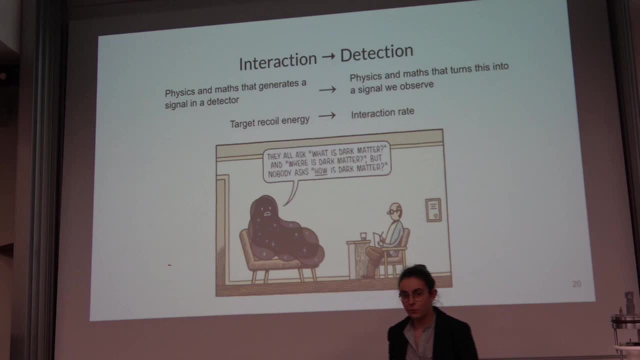 to what we think dark matter should be. So this is where I'm handing you over to Bill. I've talked about the interactions, so the physics and maths that's going to generate a signal within a detector which gives you a target recoil energy spectrum, And Bill is going to talk about the detection, so the 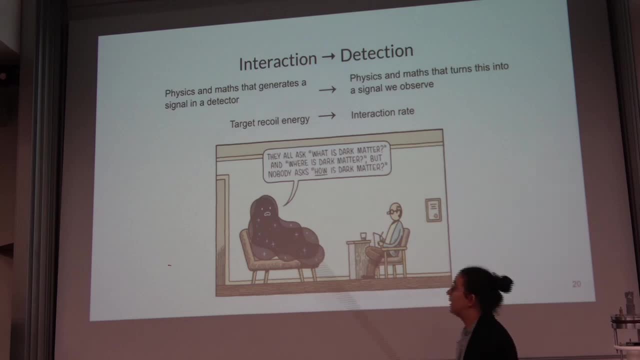 physics and maths that turns this into a signal we can observe, which I have probably talked about a lot in the past. So I'm going to talk about the physics and maths that turns this into a signal we can observe, which I have probably confusingly named an interaction rate, but it's more the interaction rate that we 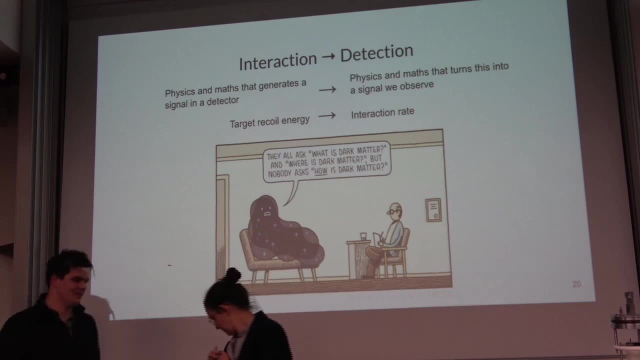 actually observe While they're swapping over. just go ahead and comment if you'd like to ask a question. Actually, put your hand up if you have the time. Were there any questions to Bailey before she moves off, And Bill, if any questions come up from the chat, I'll just try to let you know. 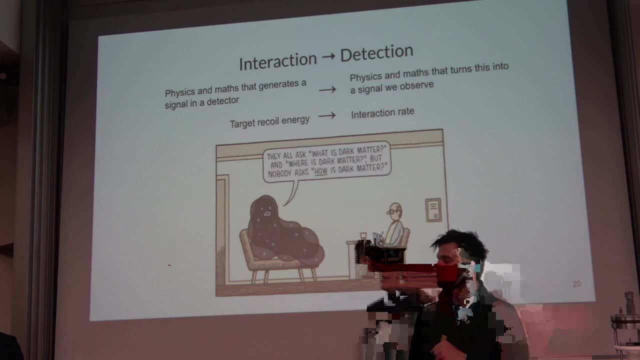 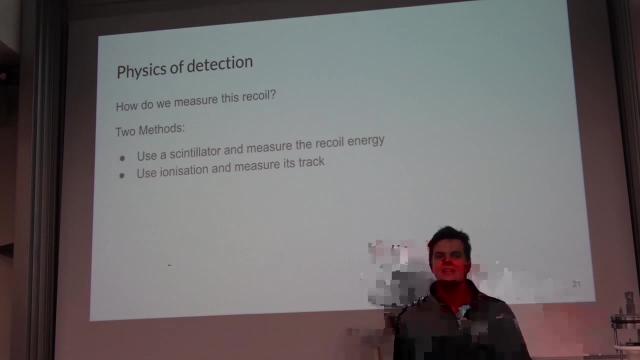 Perfect, Okay. So yeah, I now get to talk to you about how we actually see these processes. So, whilst I'm talking about this, in how we look at the dark matter, it's exactly the same thing you'd use if you wanted to study other particles. So, whether that's at a particle collider, 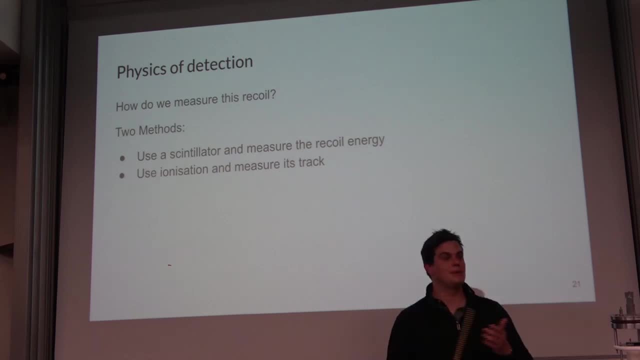 or even if you're using it in like medical technology, like PET scanners that use particles to observe like areas of interest in the brain and things like that. So this idea is kind of quite universal whenever you want to observe a particle interacting. So there's two main measures to measure a particle recoil for dark matter. So one of 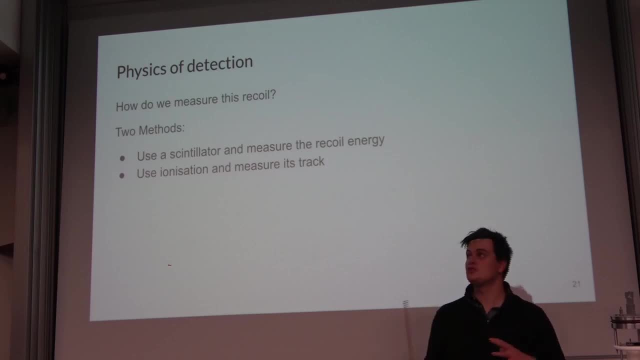 the approaches is to use a scintillator where we measure the energy of the recoil, and the other is where we use ionization. that gives us a nice track we can measure for the recoiling particle. So I'm going to start off with what a scintillator is. A scintillator is just any material that. 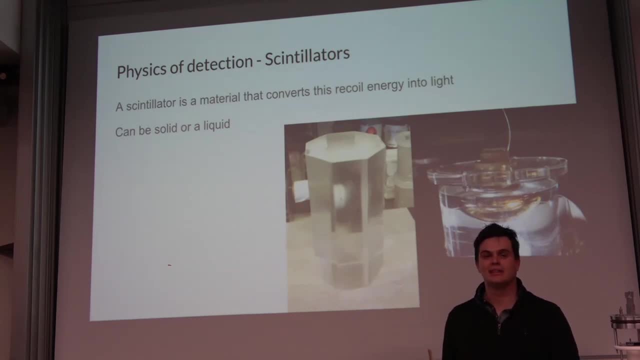 when there's a particle recoil inside it, it gives off light, So it can be a solid or a liquid. This somewhat blurry photo here is a sodium iodide crystal. We keep talking about that because that's what Saber uses and we'll talk about that later. It can also be a liquid. 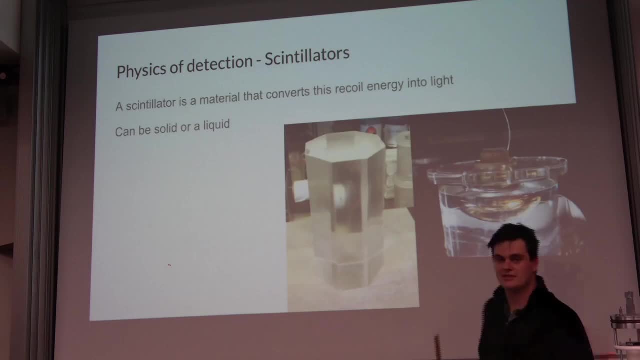 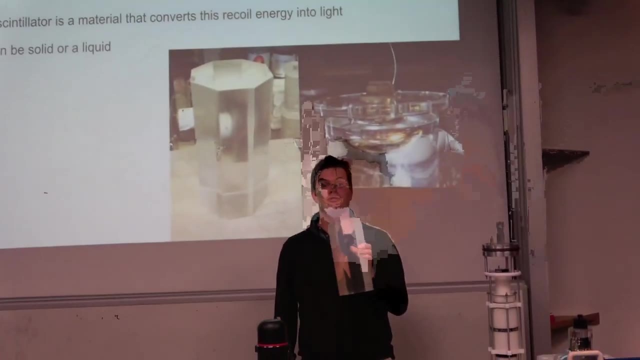 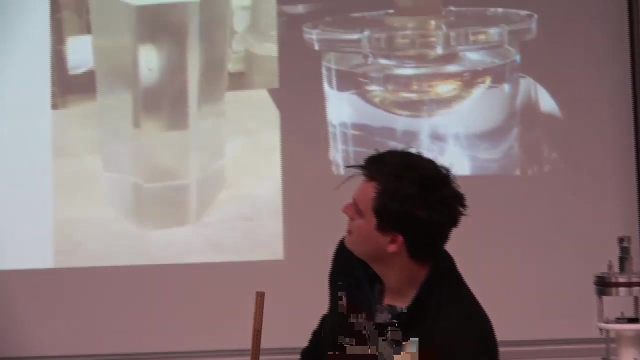 So this again picture is a tank of a liquid scintillator with a PMT inside it. I even have a somewhat boring clump of it here. Unfortunately, the amount of light it produces when a particle interacts is really small, so we can't see it here. Yeah, so that's the scintillator. 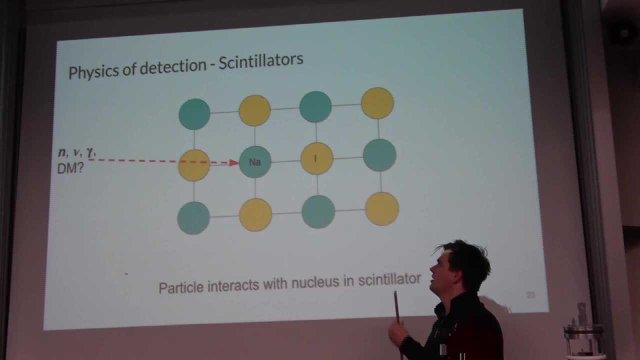 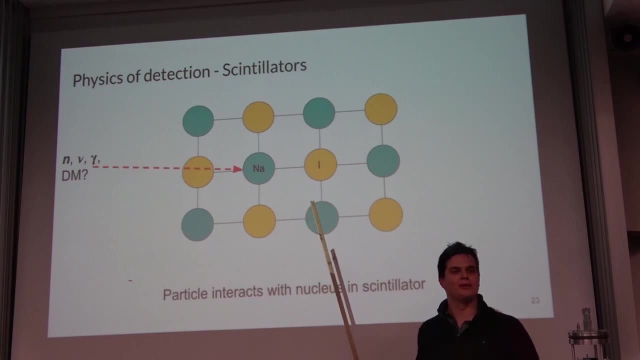 So how a scintillator actually produces light. So this is a crystal, So we're going to have a solid dark matter. Sorry for these low like low quality animations. This is my own handiwork and I'm not very good at. 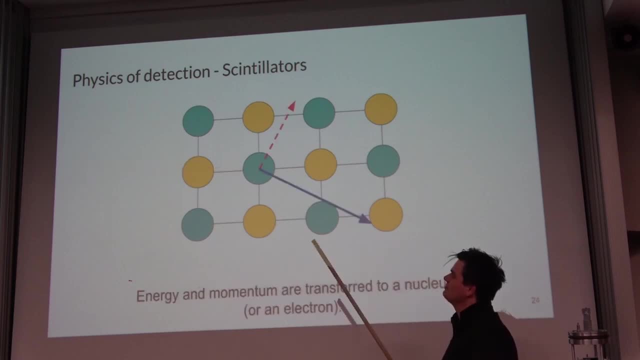 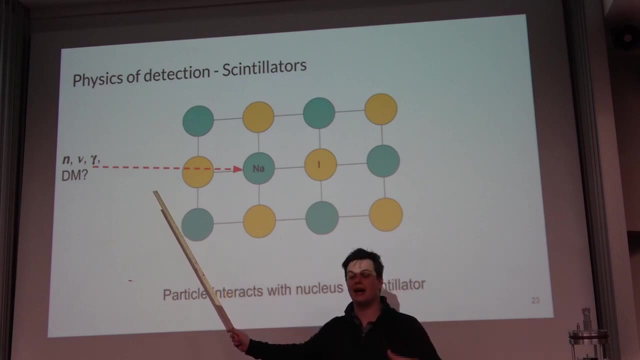 drawing things, Yeah, So it's Sorry. So if we start with some, in this case we'll say a neutral particle, So it could be something we know like a neutron, a gamma ray or even a neutrino. 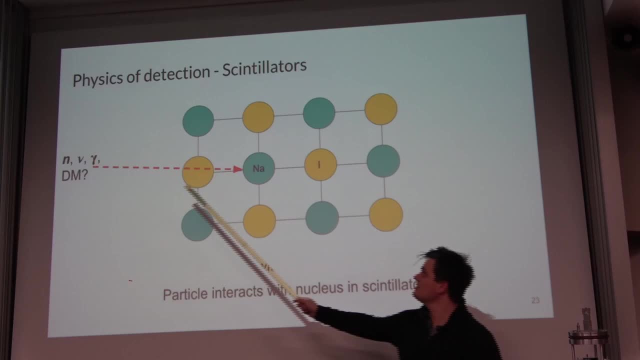 It could also be dark matter for some theories. So this comes in and it will interact with one atom in our scintillator. So because of this is a collision. it's like any other collision: it'll impart some energy and some momentum to our particle. Next slide: 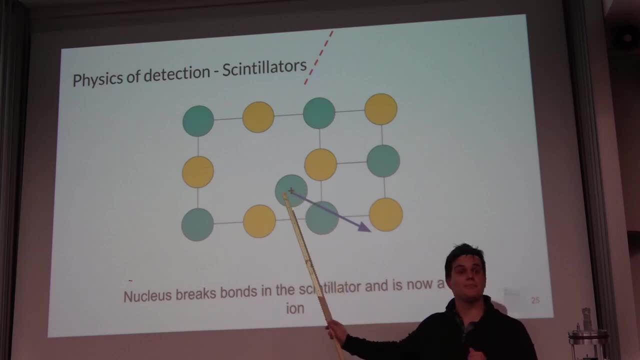 So this, in our case, might be enough for the particle to break the bonds in the lattice and start traveling through the scintillator. and when that happens- because this is now an ion- it's broken its bonds and I'll either be missing some electrons or carrying some extra ones as it travels through it's going to. 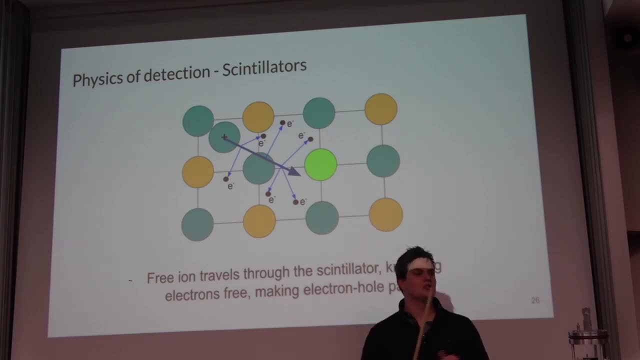 knock other electrons loose, creating an electron and an electron whole pair. This is kind of what you'll see in, sometimes in silicon as well, and the point is, as these go out, next slide- sorry- our particles now gone and we're left with these electrons and the space is where electrons should be, and what happens is: 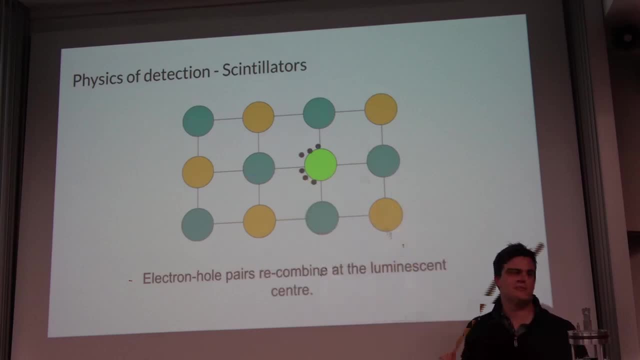 these are going to travel to something that's called the lumenscent center- that's not how you pronounce it, but I'm just going to go through- and they recombine here. so now you've got the electron and the space where an electron should be. when they recombine, they give off energy and that. 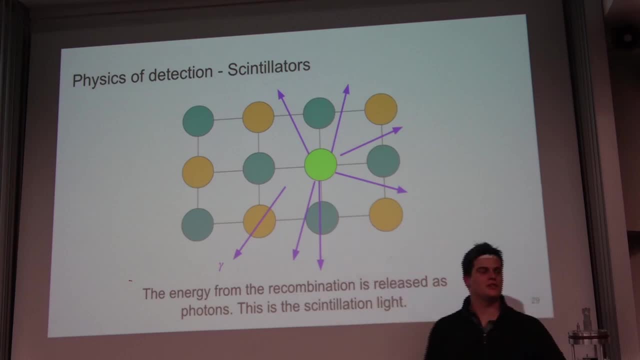 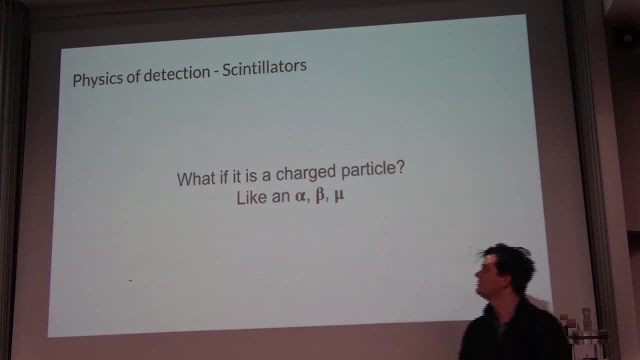 gives off light. So suddenly we've turned a particle, bumping another one, into a light signal in our scintillator, and that's something that we can measure. So what would happen if we had a charged particle? right? you all know about alphas and betas, right. and then this here is a muon. it's just like an electron, but a. 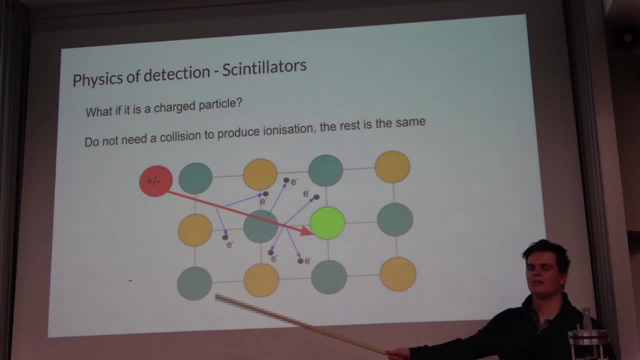 bit heavier. So what happens if it's one of those? Well, we just get to skip a bunch of steps at the start. right, because this is charged when it travels through the scintillator. it's just going to knock those electrons off by itself. They'll then recombine and give us our light as 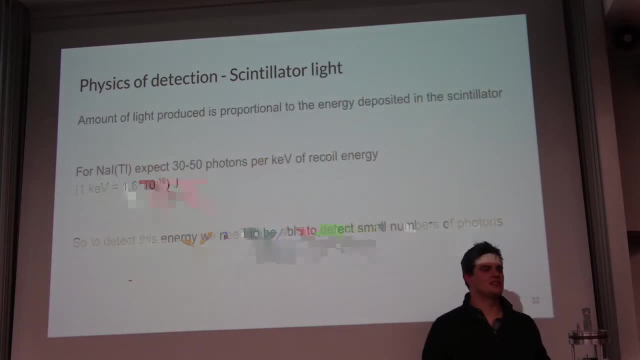 normal. So what does this scintillation light look like? So the amount of light is proportional to the amount of energy deposited, but to give you an idea of just how much light we get for a dark matter like event again, the scintillator. 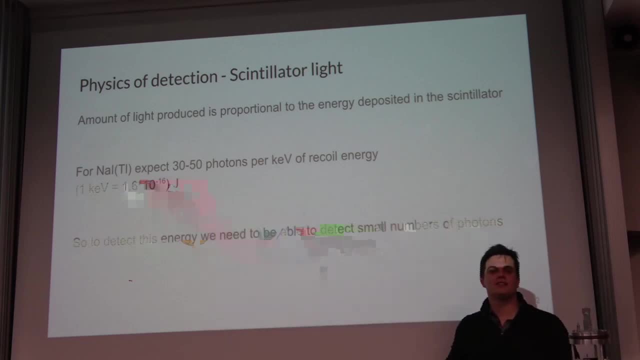 that we use produces about thirty to fifty photons per keV of recoil energy, So that's a very small amount of energy. that's helpfully done here. that one kV is 1.6 times 10 to the minus 16 joules. right, that's tiny, but for a particle it's a reasonable amount of. 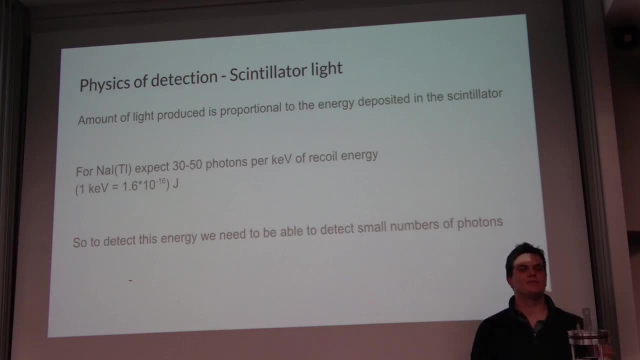 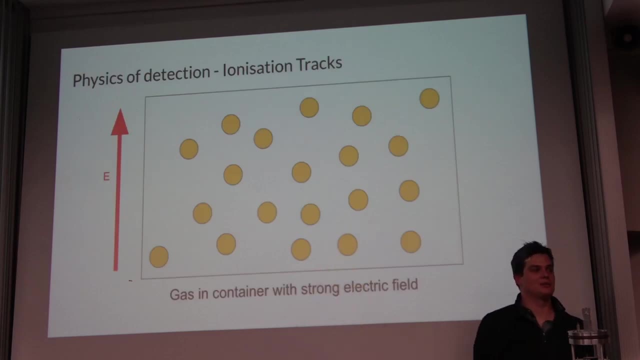 energy. So to detect this energy, we need something that's very, very sensitive to measure this light, and I'll talk about that in a little bit. So on to the other way. we can detect a particle, which is ionization. So in this case we have some. 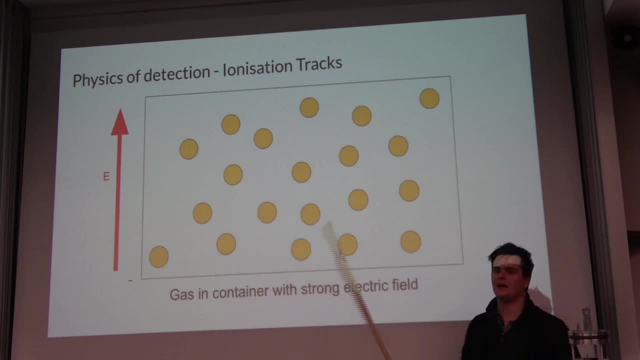 particles in a volume and we apply a strong electric field to our gas. So now our particle comes in- next slide again, it interacts with one of our gas atoms. we have a collision. so this atom now has energy and momentum and it will be. 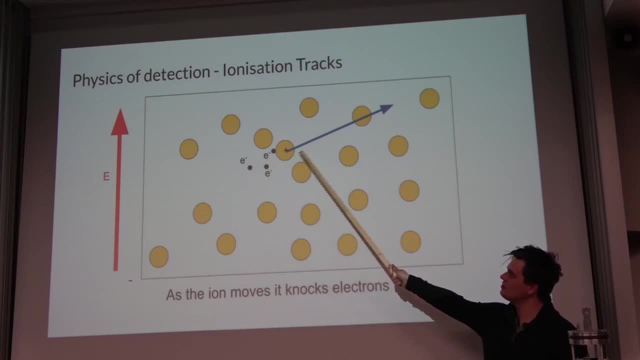 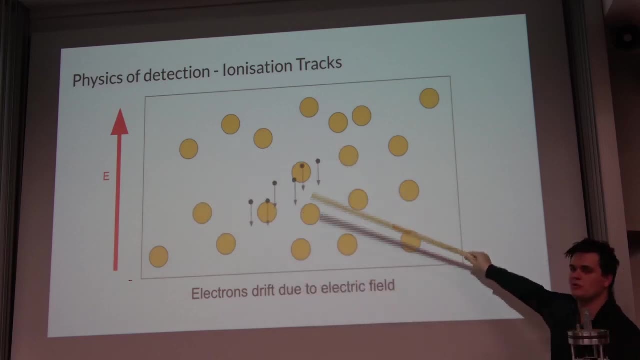 ionized sometimes, and as this travels, now again it knocks electrons loose and then it goes away. But because of our strong electric field, now our electrons are going to drift through the gas and as they drift, eventually they reach the gas. So we can detect them. and not only do we detect them, we can detect their. 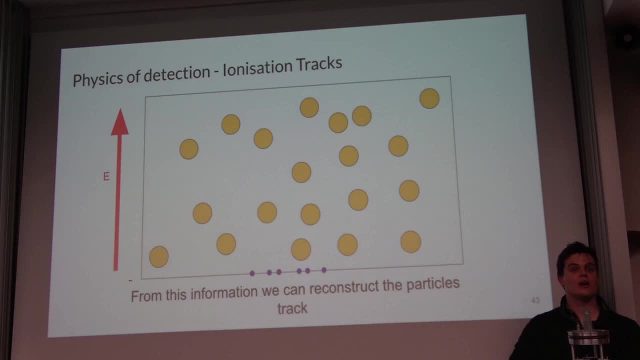 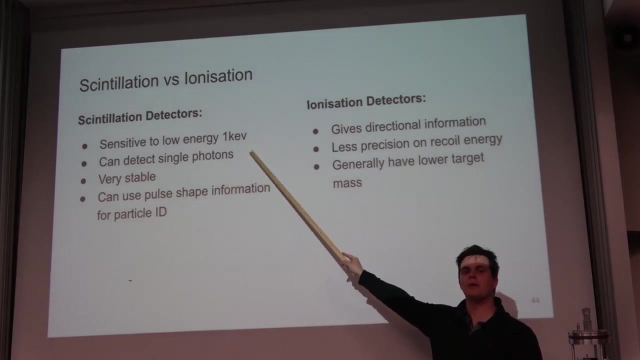 actual position and the time and from that we can reconstruct the path of our recoiling particle through the tank. So this technique actually lets us measure the direction of a particle. So as a very quick recap, when we've got scintillators, these are really good for looking at low energy processes like dark matter. We can. 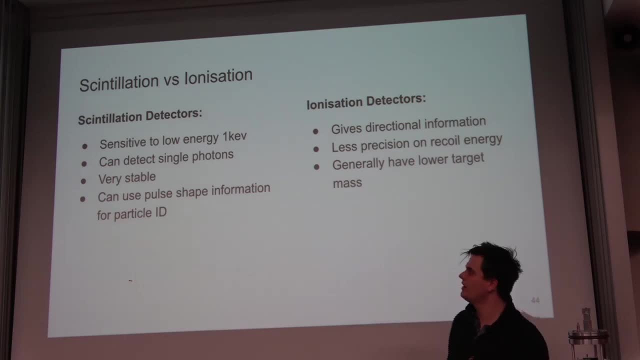 even use them to detect energies that would only produce a single photon. So that's very important: Very, very low. Importantly, they can be very stable. Obviously, this is a chunk of plastic. it's not going to change much over time and you can. 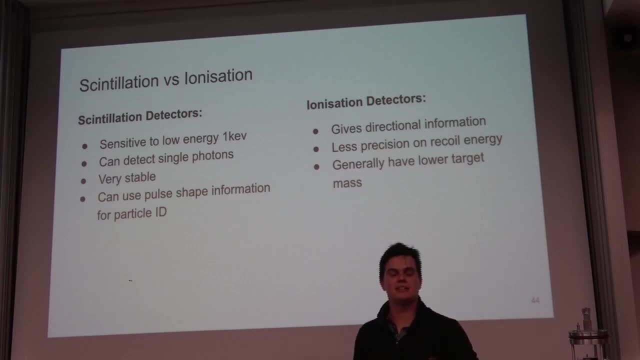 potentially tell what kind of particle it is by how it interacts in the scintillator If we compare it to ionization detectors. these are really good because they can give us directional information. They can tell us that a particle came in. well, the thing that recoiled off, the particle came in. 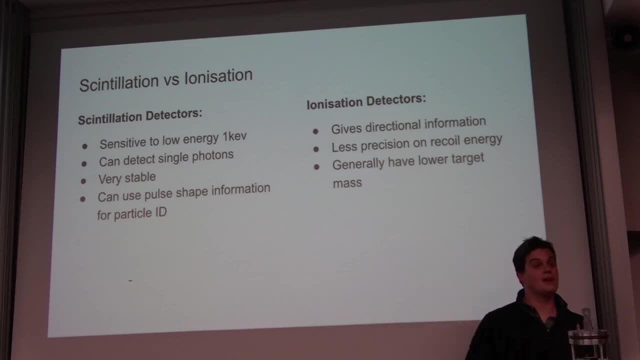 this direction. The problem is it doesn't give us as much precision on the recoil energy and you generally have less target mass because- remember Maddy was talking about it's- the number of particles affects your rate. Obviously, a gas has a lot less atoms than a big solid chunk of something, So I think we 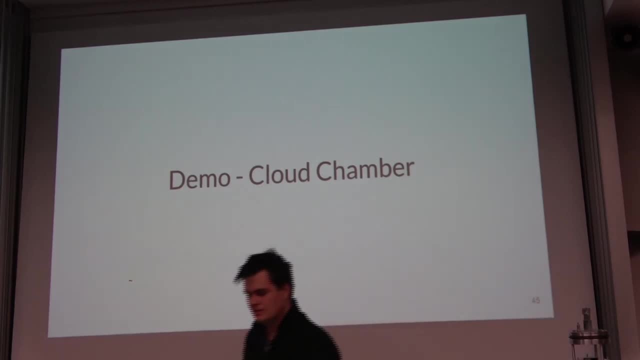 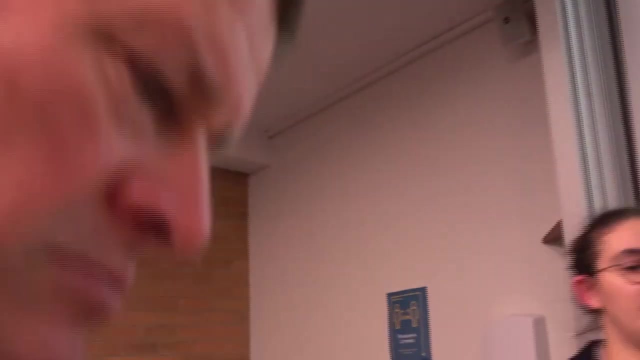 have a demo now, which is our cloud chamber. We might do. we have it. is it working? Yeah, So we might bring. we'll bring the camera up and have a look. So the cloud chamber is an ionization type detector. You can probably come up to the front and have a. 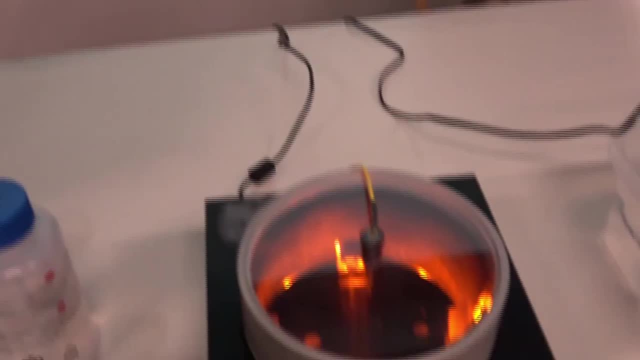 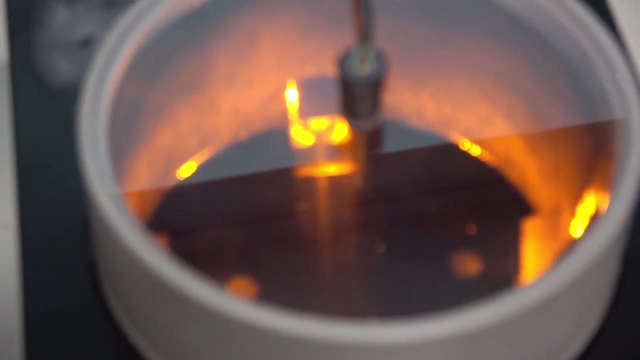 look as well, So I'm not sure if you'll be able to see it, but what you can see here, if you look, is you can see these little like pulses. So these are the tracks of particles coming in. You might have to like lean over the top to have a look. 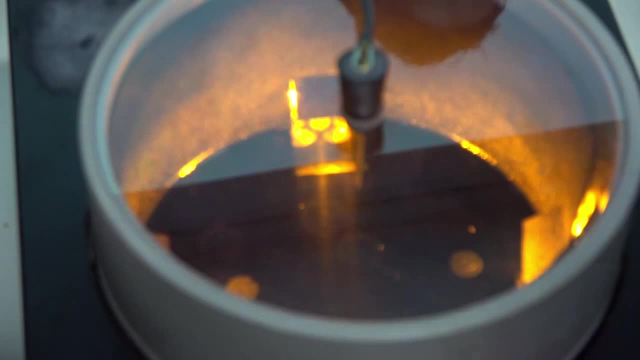 Those are actually tracks being caused by particles, So they only last two or three seconds. Yeah, We've got some good ones now. So in a real experiment we would use something to record where these tracks hit the ground. Yeah, We can. 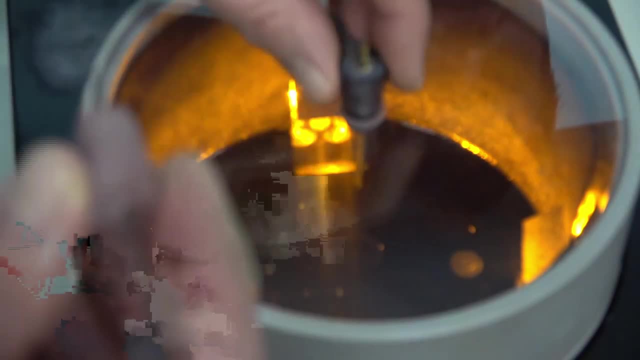 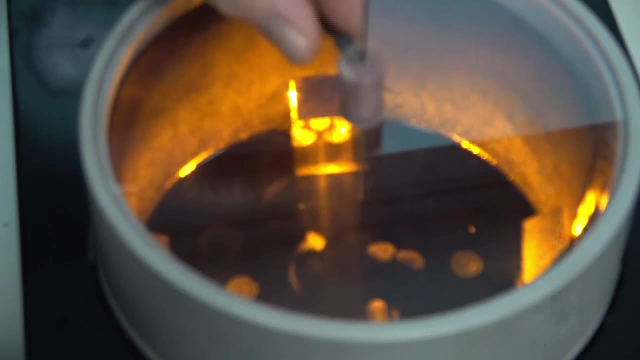 swap sources. This is an Alpha Source. This is throwing coating on it So we can put these here. There you go. So, if you remember, Alpha particles are a lot larger, So you can take out the particles and then put them away from the ground, Because 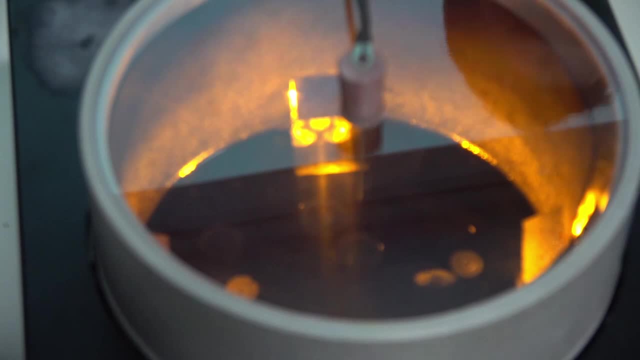 So you can see that they give off some bigger tracks in the tank. I could watch these for like days. it's so cool. Yeah, so this is exactly that process that Bill was just talking about, the ionization, except in this case you can see the tracks occurring. 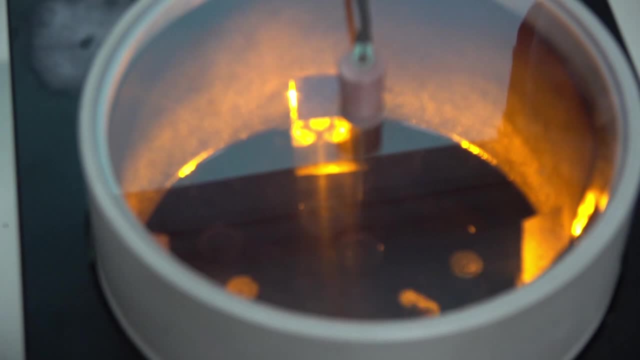 Yeah, So I guess are there any questions about this, since we've got this all here, I'm just watching. there's none coming out, so these guys can answer. Do you have any questions? No, No, That's all right. 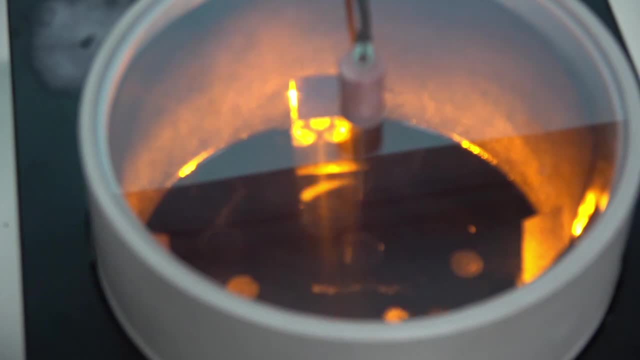 Okay, Carry on our merry way, then I think we'll keep going. This will probably still be here and running afterwards. if you'd like to come back, have another look and ask any questions about it as well. Thank you for that, Steve. 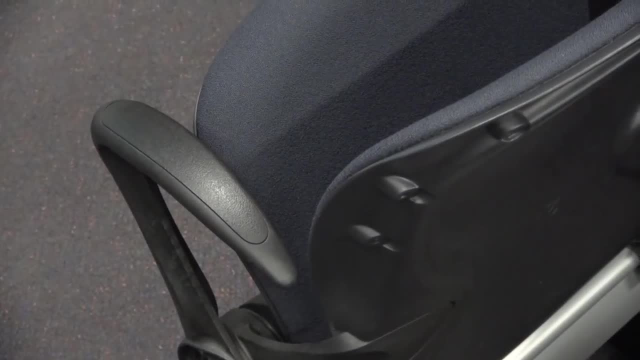 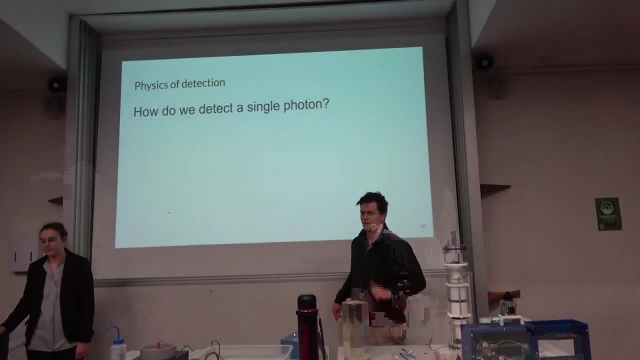 Quite a bit of setup just for 30 seconds. I know it's been two minutes. yeah, I was just watching here. I'm not sure if it's fine, Perfect, okay. So now to go back to how we detect a scintillator event. 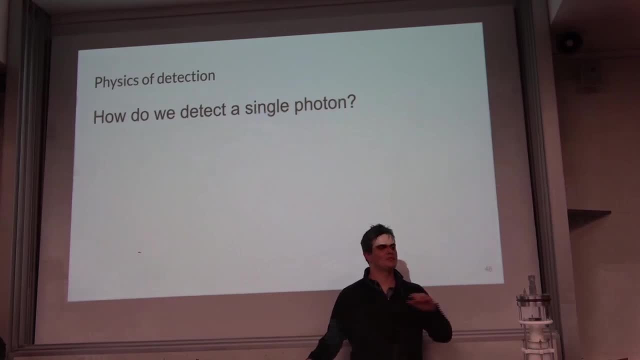 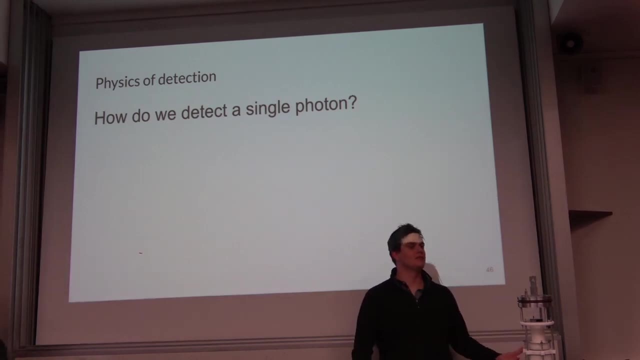 So detecting these? we just have a little sensor that reads out when an electron comes, But how we detect this scintillation event is going to be different, because how do you find a single photon? How do we turn a single photon into something that we can measure? 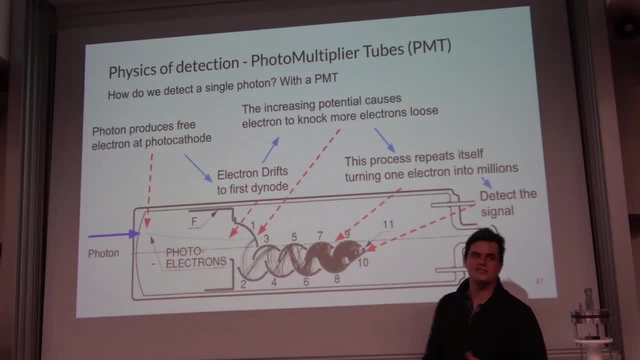 And the answer is it's with something called a PMT. So this is what I've basically been working on for the last three years. So I could quite easily bore you. so I could quite easily bore you. so I could quite easily bore you here. 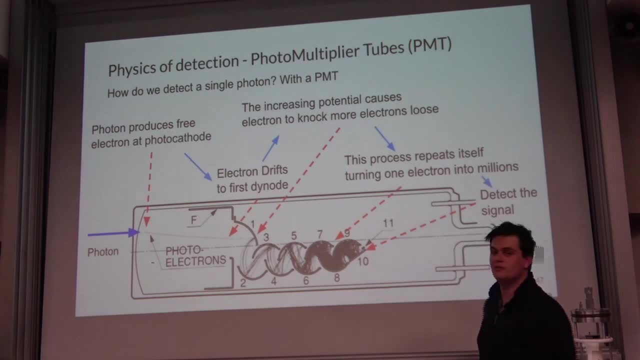 I'm trying not to, but if I stray too far, either please ask me a question or you can give me, like some sort of hurry up sign. So this is a very complicated diagram, but it's all about how we detect a single photon. 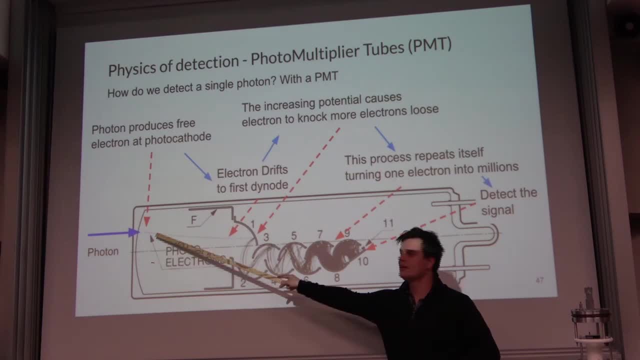 So the first thing is our photon comes into the PMT and it knocks an electron off at the photocathode. So this is the photoelectric effect. I know it's something you study quite a lot when we talk about the nature of light. 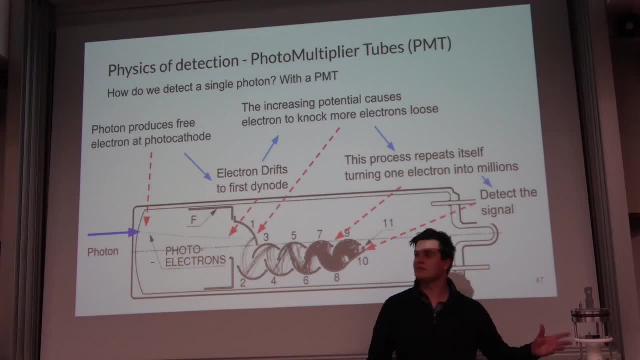 PMTs wouldn't work if light at least wasn't a particle sometimes. So this will then knock an electron off, and this entire thing has a very high voltage applied to it, So this can be something like 1500 volts or even 2000 volts. 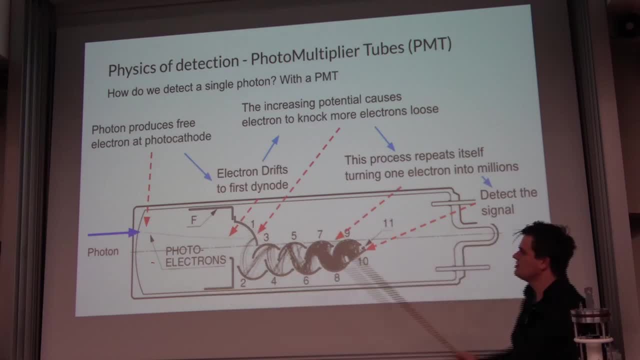 And it increases as we go from this end to this end. So because we have a really strong potential, our electron is going to be drawn to this first metal stage. It's called a dyno. It's just a nice piece of metal that attracts the electrons. 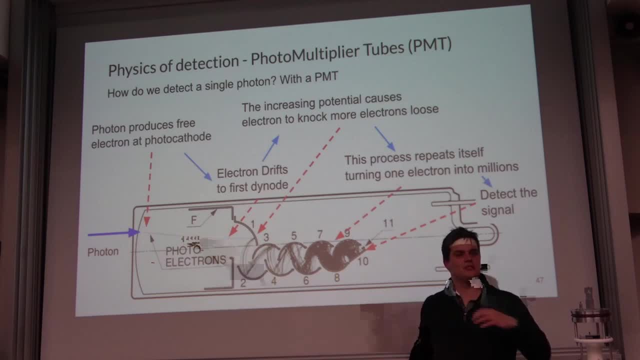 So as the electron comes, it's going to increase its energy, right, Because it's basically going, it's being drawn in And when it gets here it has quite a bit of energy. So when it collides it suddenly knocks off a few more electrons. 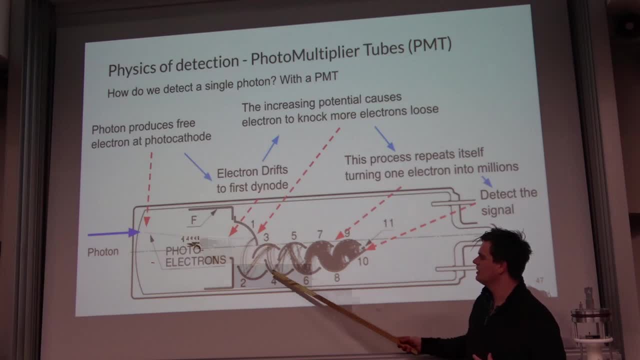 And then the same thing happens, as it goes to the next one and the next one, And eventually, in a process that's basically like an avalanche, one electron will turn into millions of electrons And suddenly that gives us a signal that we can measure. 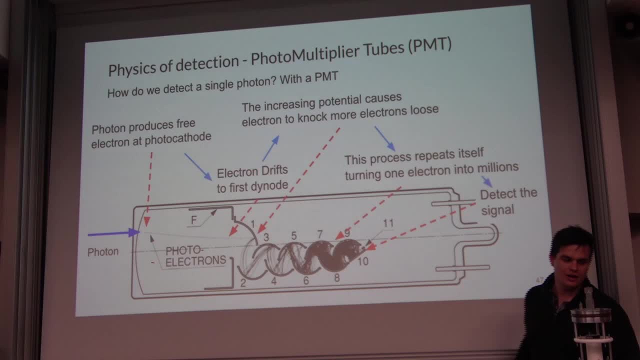 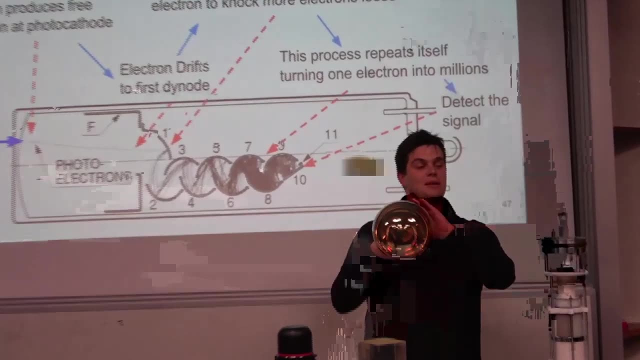 So next slide. Oh yeah, I have a lot of examples Of this, since this is something I work with, So this is one of the ones that we'll use here, And it's just the same thing, but much, much bigger. 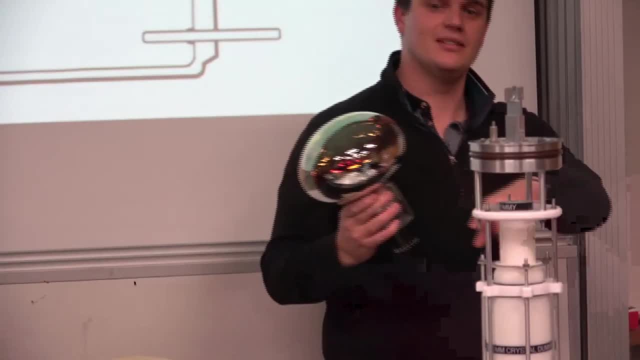 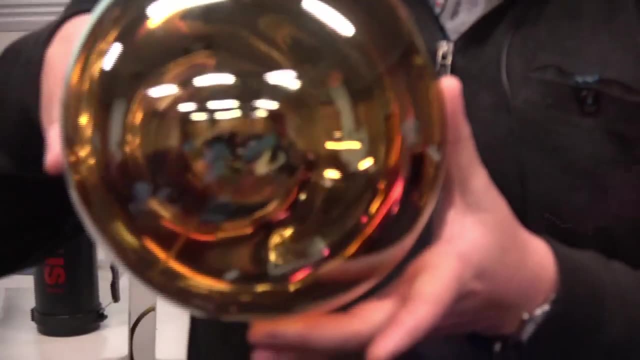 So I'm not sure if you can really see. I can come in front if that's easier. So there's a faint gold glow on the front. This is because of the photocathode, And then if you look inside, you might just see a flat piece of metal. 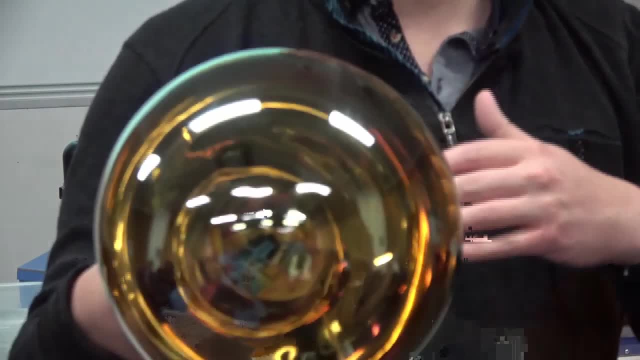 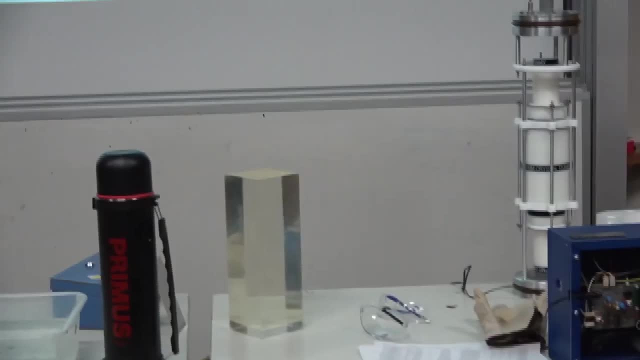 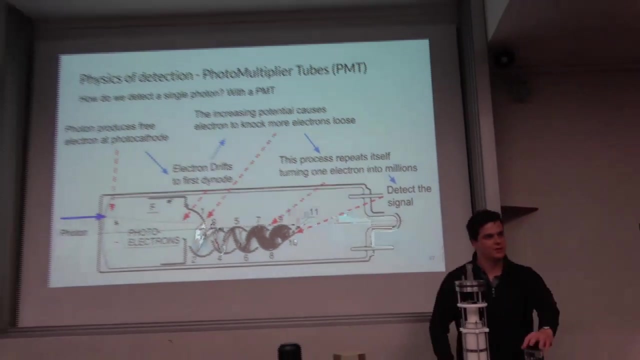 And that is the first of these many metallic stages, And then eventually we get a signal out from one of these pins at the back here. So I have quite a lot of these, And I'll talk about these ones specifically a little bit later, because these are actually part of the SABER experiment. 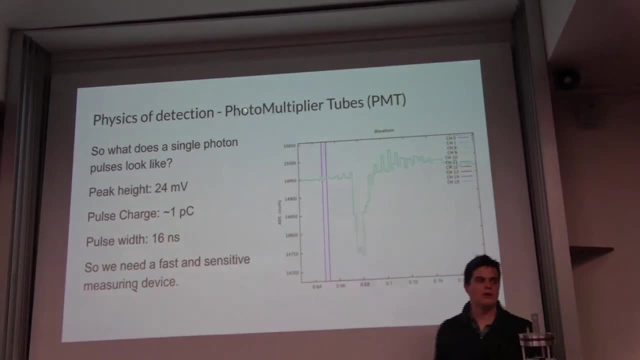 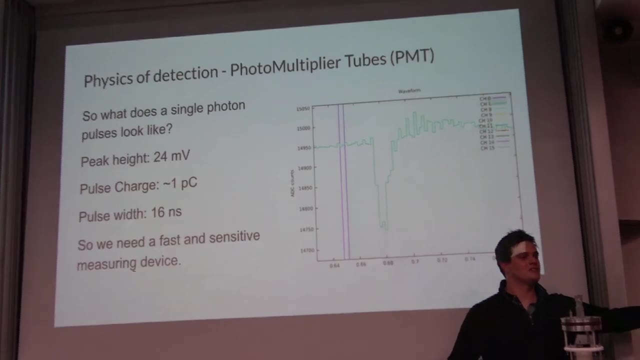 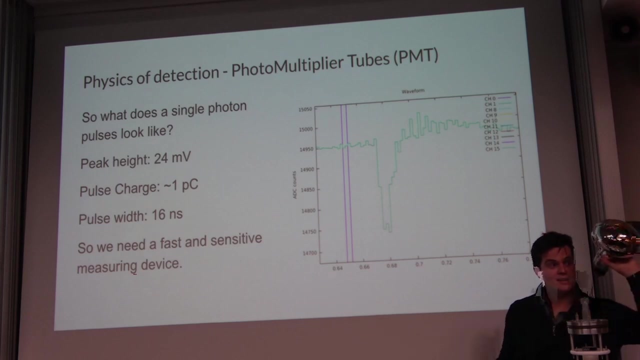 that we use. So what do one of these pulses look like if we have a single photon? So one electron's turned into millions of electrons. A million electrons still isn't a lot. So this is a pulse from a single photon. Actually, that one was recorded by exactly this PMT. 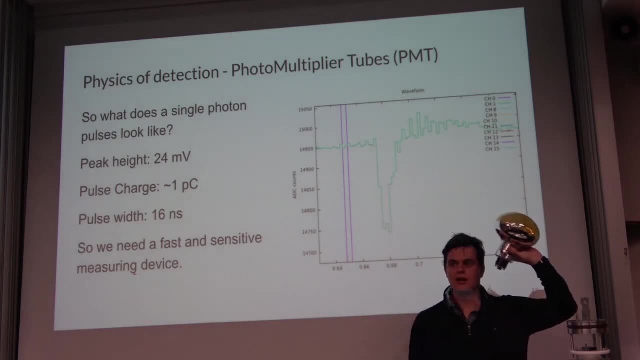 I have to be careful not to drop this on camera because I I will get in a lot of trouble if there's evidence of me dropping it because I was careless. But you can see, But you should work out what the photocathode's made of. 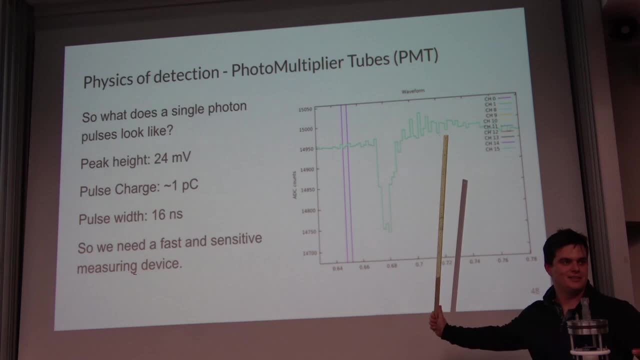 We'd have a great teaching demonstration, but this is probably. this is worth, like what I get paid in two months, So I'm not rushing to drop that on the ground. So this is what our pulse looks like in green. You can see it's flat. 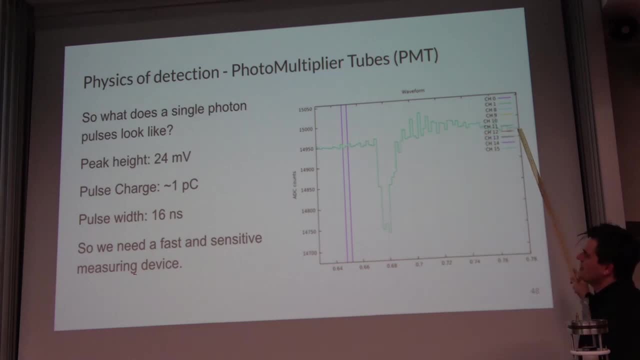 We get a big spike and it's back. But to give you an idea of what this pulse is, the height of this pulse is only 24 millivolts And the width of the pulse from here to here is only 16 nanoseconds. 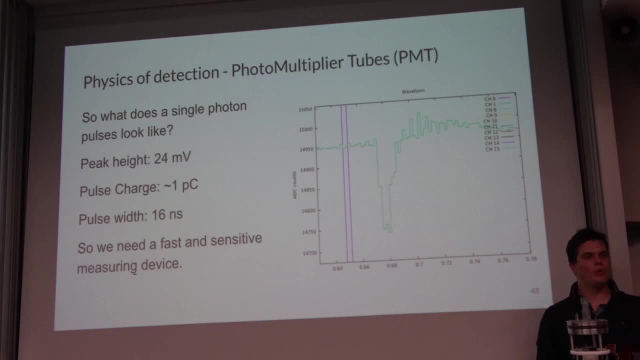 So it's still a tiny pulse. It's just a lot bigger than one single electron. This one has a charge of a picocoulomb, So that's one times 10 to the minus 12. So that's about 10 million electrons. 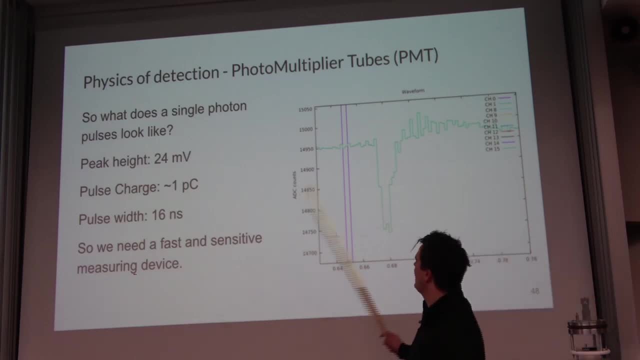 So we've turned one electron into 10 million electrons and it's still really hard to see. So whenever we measure these things, we need really fast and really sensitive detectors. And we do have those, but it's not easy by any stretch of the imagination. 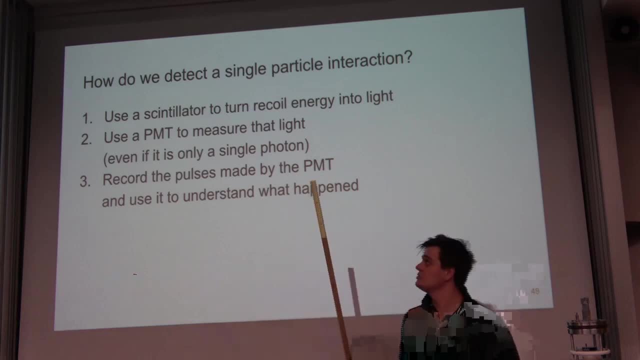 So I guess, as a summary of how we detect a single particle interaction, so we start by using a scintillator to turn our recoil into a light, into photons. We then use a detector like a PMT to measure that scintillation light. 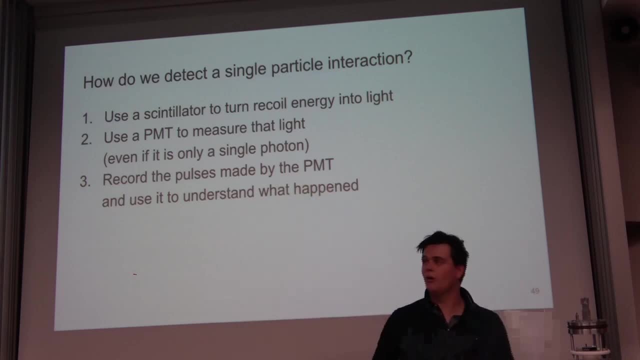 And then, finally, we can record these pulses, like we had on the screen before, and use that to then understand what happened. So from that we can figure out the energy, how often it happens and potentially based on the shape of that waveform. 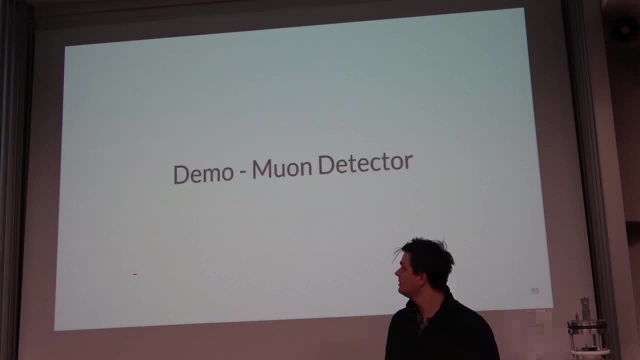 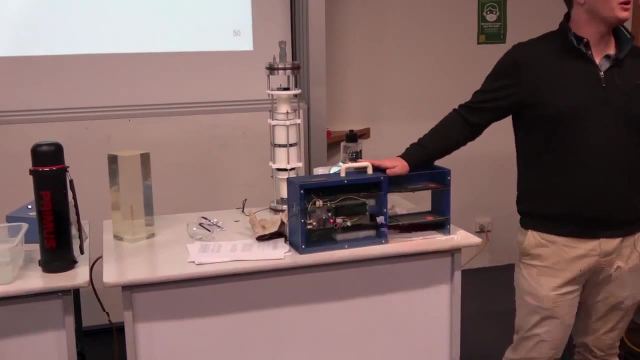 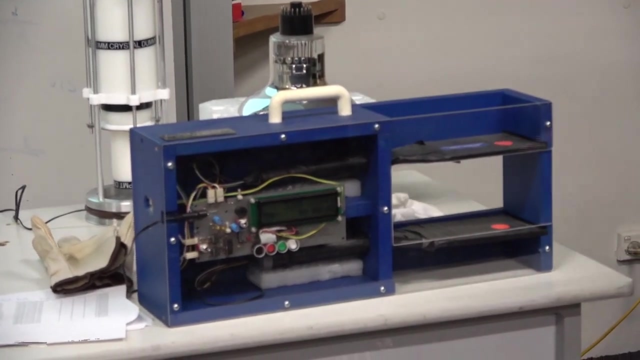 what type of particle caused the interaction. So I have another demo here. This is our muon detector. So, as I said, a muon is just a heavier electron And they're produced in the upper atmosphere from cosmic rays. So there are muons passing through us the whole time. 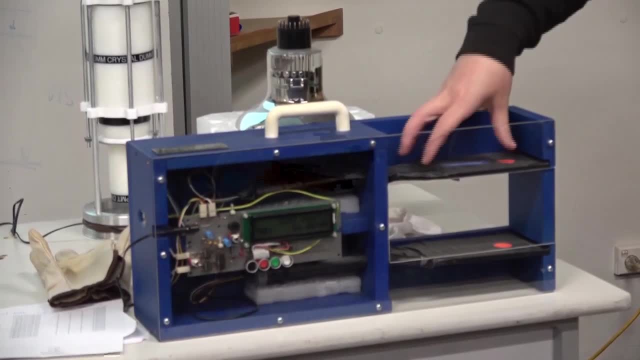 And what this detector is is. it's exactly the same as the one that I just showed you is. it's exactly the same thing. We have a scintillator here that's coupled to a PMT Now, unfortunately, because it's very sensitive to light. 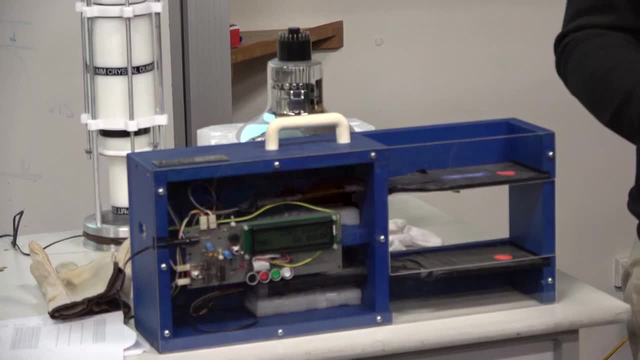 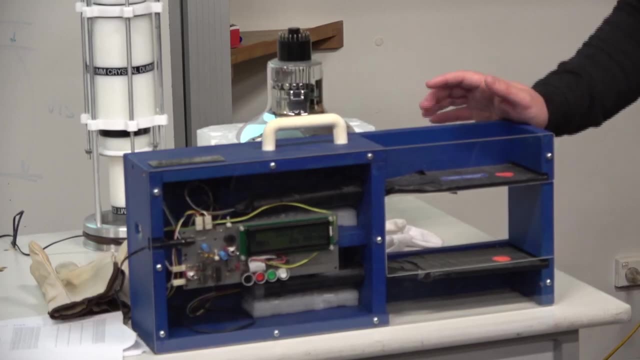 when we actually use these detectors, they always have to be wrapped in a lot of things to make them light proof, So that's why the entire thing is covered in black duct tape, But every time you hear one of those beeps, that's a muon- passing through these scintillators. 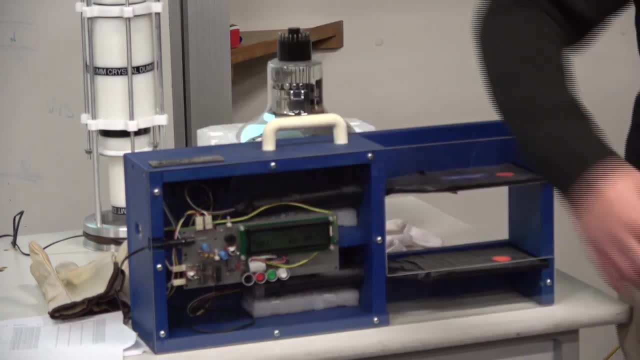 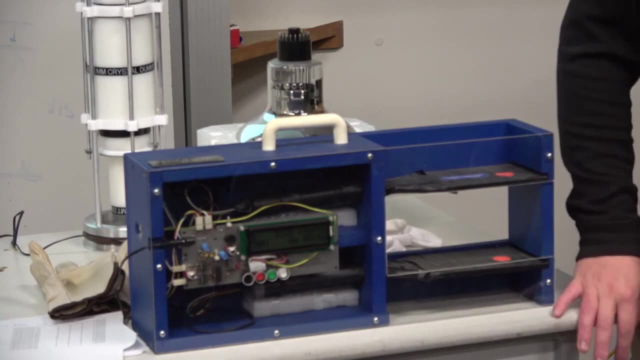 giving off light, which is then collected and turned into an electric signal. So this is also the background I was talking about at the start. Remember how I said we had to observe one count in a day? These are all the counts that are becoming our background. 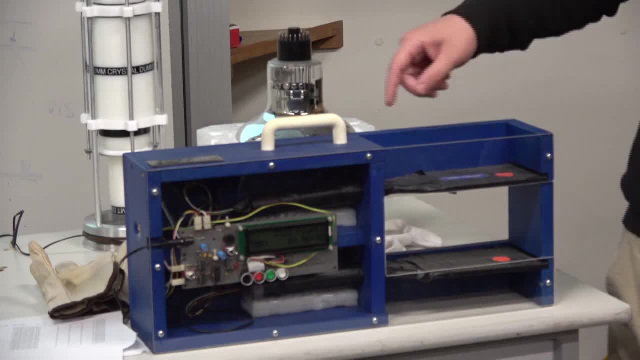 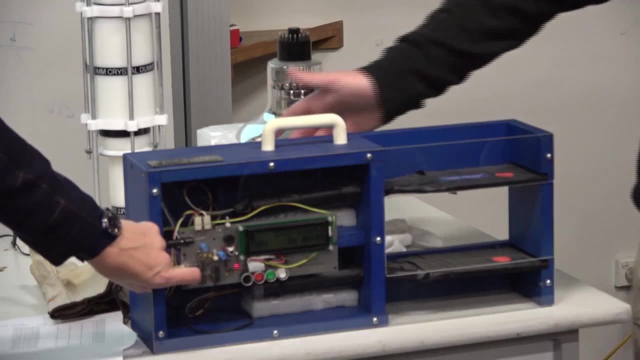 Yeah, So it's one count a day versus oh, it's just going quiet for a second. Turn it on to the coincidence setting: Oh, we can, And this was what would happen if you had. like, this is all the noise that you really get. 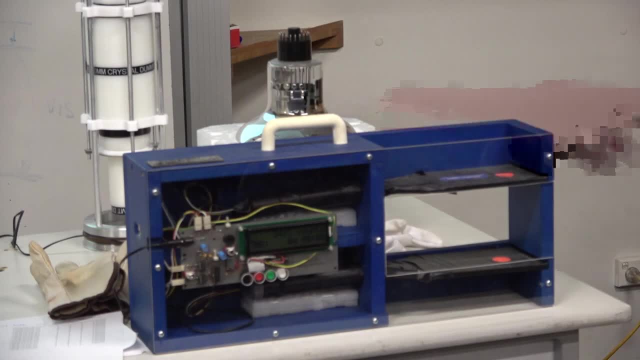 So that very rare pulsing was when we were already doing some work to try and get rid of some of the background. This is going to get a very, very annoying if we keep listening to it, but this just gives you an idea of why it's very hard. 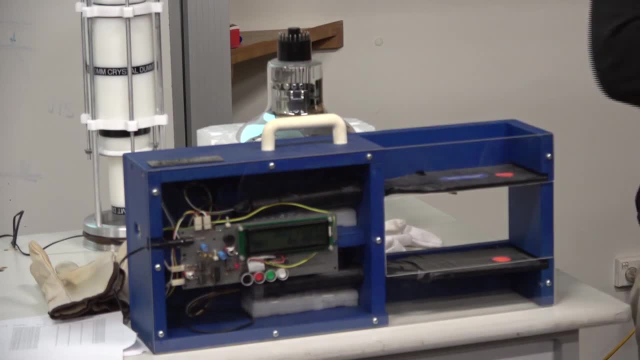 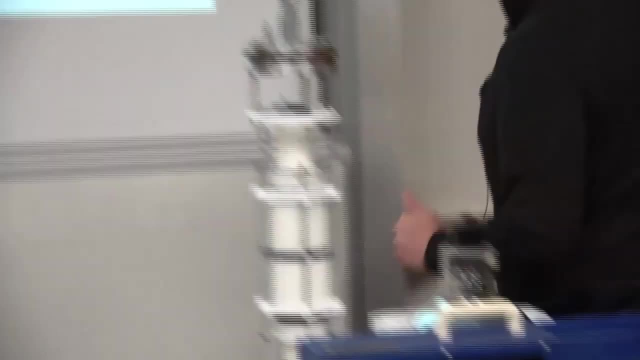 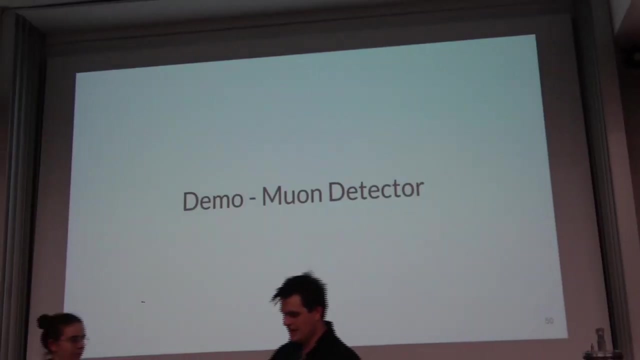 to look for dark matter, because we're looking for something very rare when there's a lot of other stuff going on to start with. Yeah, So I'll hand you back to Maddie for a couple of slides, If that's, I guess. are there any questions about that? 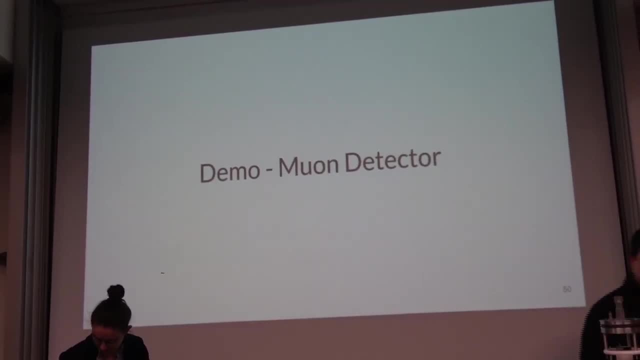 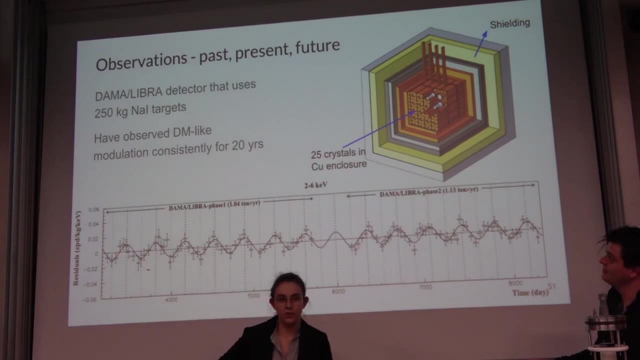 No, Okay, All right. So, finally, we promised to tell you guys about the status of some of the actual searches that are going on, So the big one that we've been talking about quite a bit, apart from SABR, is another one that uses sodium iodide. 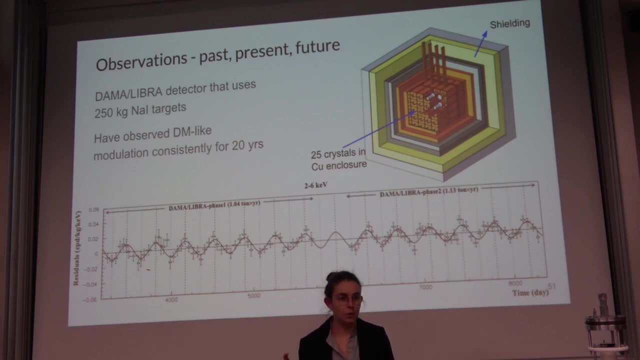 crystal, which is why they're so important, And that's called Dama Libra, which uses 250 kilograms of sodium iodide. There's a picture of the detector just here, So you basically have this cube that has all of those crystals. 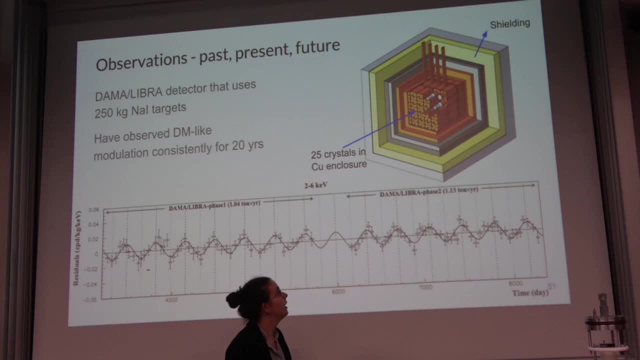 inside copper enclosures that look just like that one over there, And then it's placed inside a whole bunch of plastic and steel shielding. Now what's cool about this detector is they've actually observed exactly the signal we expect from dark matter. So remember how I said we expected it to be changing. 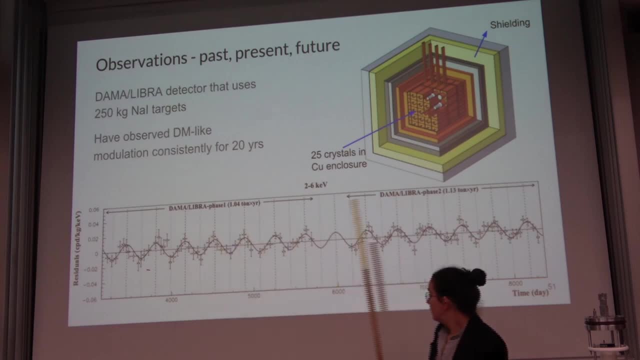 throughout the year. This is their data And you can see that it almost perfectly fits that exact same cosine curve that came up when I had my little gif before, And they've been collecting data like this for 20 years, So I'm pretty sure that's longer than most of you. 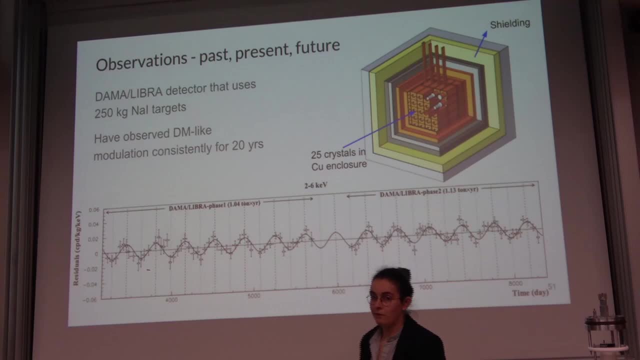 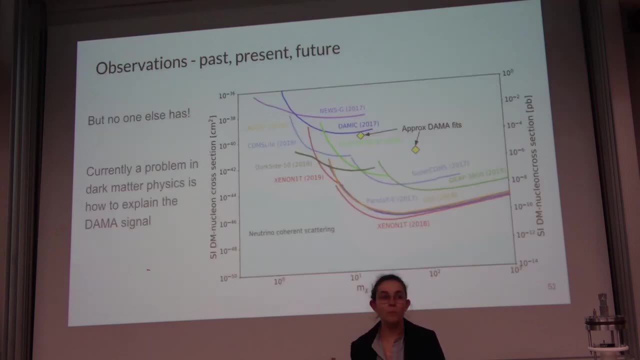 who have been walking around the planet. Okay, So this seems like very, very strong evidence of dark matter within the galaxy. There is, however, and unfortunately, a but Nobody else has been able to see it, So this is an exclusion plot, for- and it's pretty common. 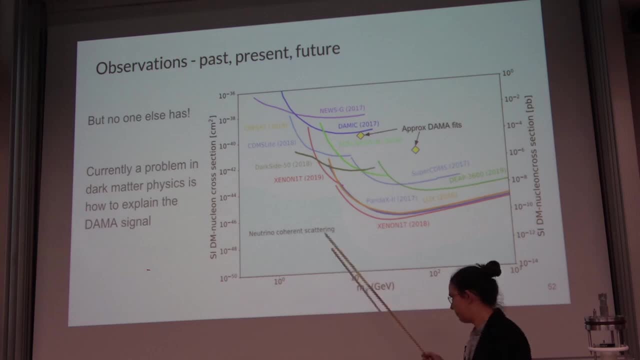 when you're in the field of dark matter And I'll just kind of walk you through what it is. So remember I said before the two things we care about are the mass and the cross-section, so how likely it is to interact. 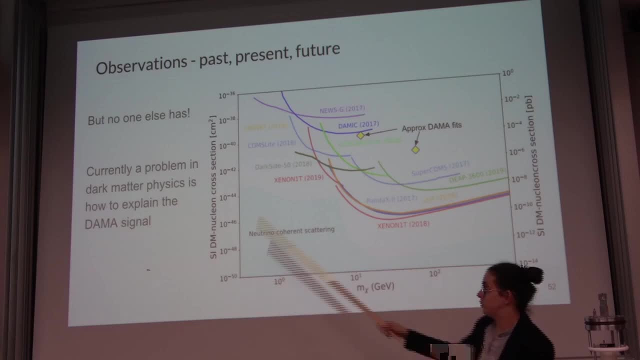 So on the x-axis here we have a mass and on the y we have the cross-section. So basically, what this plot is telling you is you can pick a point and say: okay, my dark matter is going to have a mass of 100 GeV. 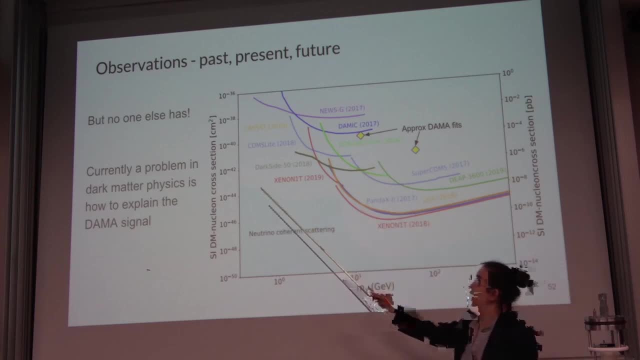 and a cross-section of 10 to the negative 42 centimeters squared. So that's going to be about here. I think Any experiment that has a line below that point is able to observe that particular dark matter model. So basically, you construct these lines. 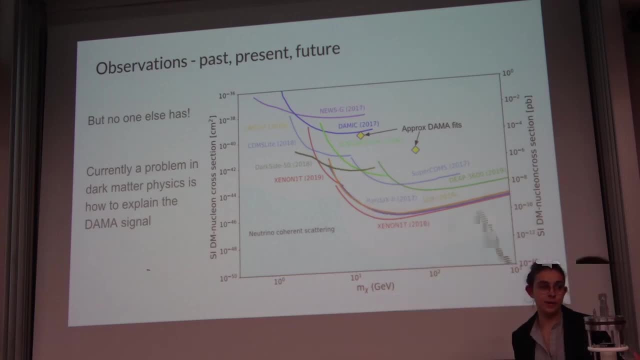 for each experiment and then that experiment says: okay, if I didn't see anything, there's no way that dark matter exists in this space here, However, the signal that DAMA has seen, which I just said was really good and looked like dark matter. 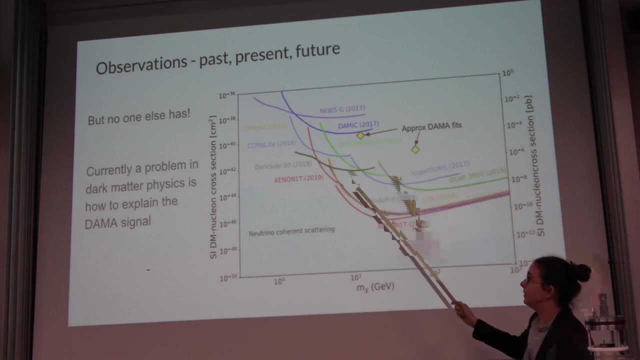 lives in one of these two spots, which is canceled out by null results from pretty much every single experiment that's being conducted since then. So this is a really big problem in dark matter physics. We don't know how we can explain the DAMA signal. 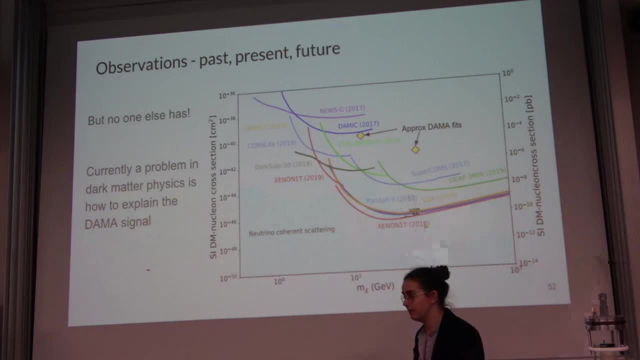 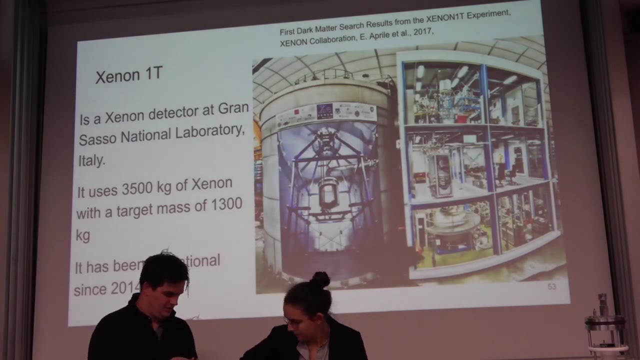 so that it's consistent with null results from all of these other experiments. I think Bill is now going to take you through exactly what these experiments are. So the first thing is I'm eventually going to tell you about SABR, which is the experiment we work on. 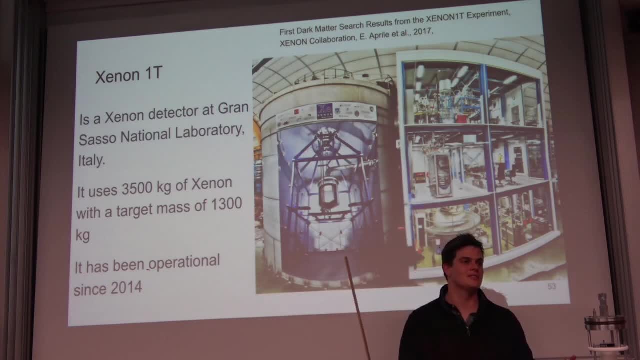 But I thought I'd tell you what the current best experiment in the world is for not finding dark matter. So it's called xenon one-ton and because physicists are very creative, you can guess what it uses for its target: It's xenon. 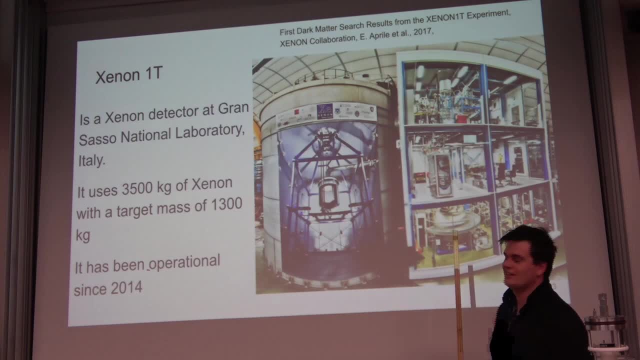 So this is a giant tank. Wait, wait, wait. How much xenon do they use, though, Bill? They use about one ton Shocking. I know We're great at naming things. If you like puns, this is the field for you. 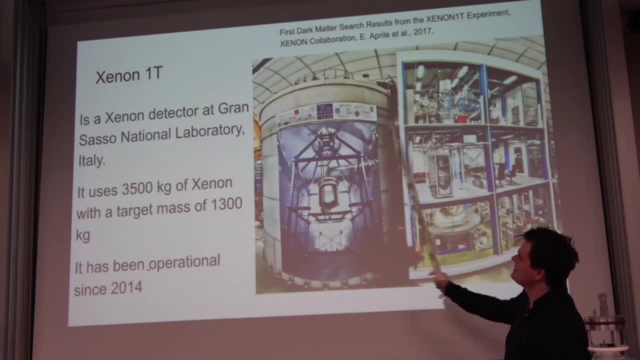 Physics that helps too. So it's a giant tank and it's located in an underground lab called the Gran Sasso National Laboratory. So in a very movie villain style, this is literally under the highest mountain in Italy. You enter it through a rolling door. 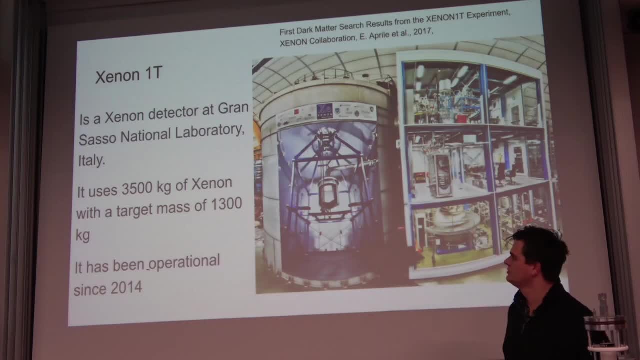 and they've got giant caverns and they use it for good, not evil, we're told. So this entire experiment is what it takes to be the best in the world at this, and in the very center- they have this picture drawn on that- there's this tiny little tank, and that's the actual center of the experiment. 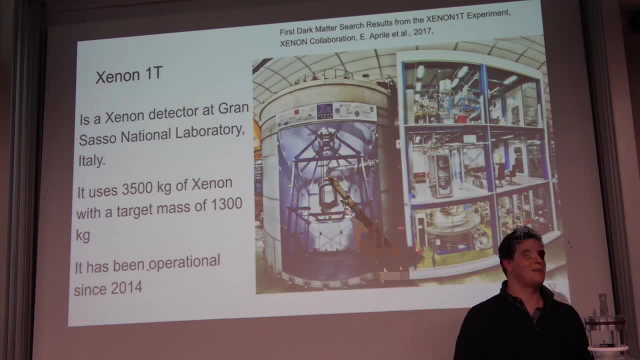 everything else is designed to find things that aren't dark matter, so they can make sure it's not in their signal. so again, it has nearly four tons of xenon, but, as the name suggests, it only really uses a just over one ton for its actual measurements. so not only is there this giant, 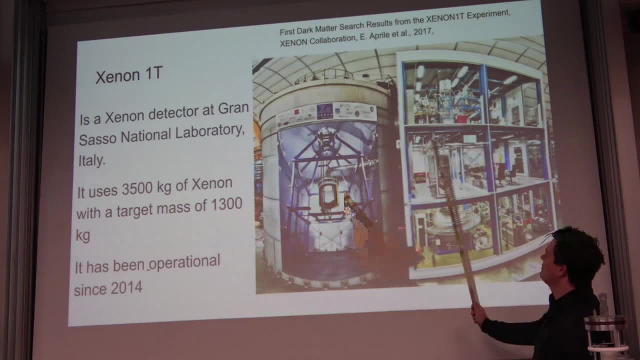 tank from all these universes that runs it. they have a three-story building that they use to run the experiment, so that has everything from computers and chemical labs to a break room and a control room and this has been running for a few years. if we go to the next slide, you can see. 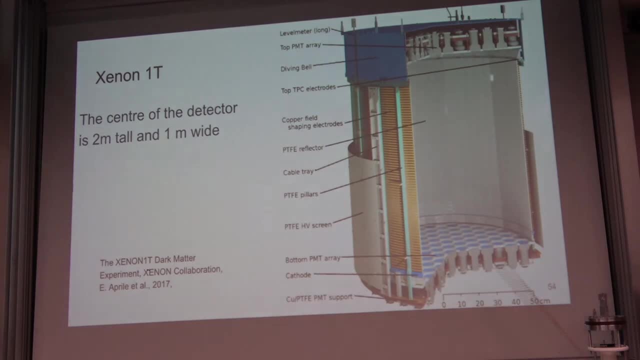 the very center of the experiment and this is a scintillation detector. so this entire space in here is going to be filled by liquid xenon, which is a scintillator and what you know. they've got PMTs at each end to read out the scintillation. 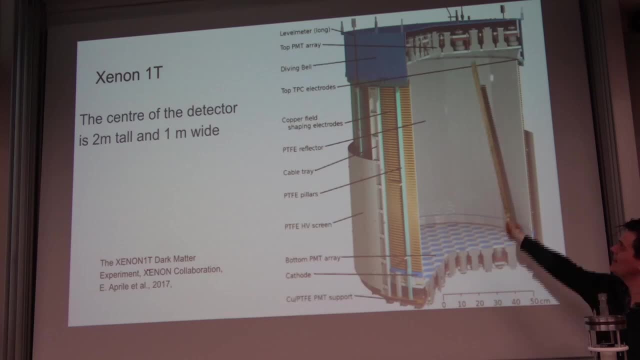 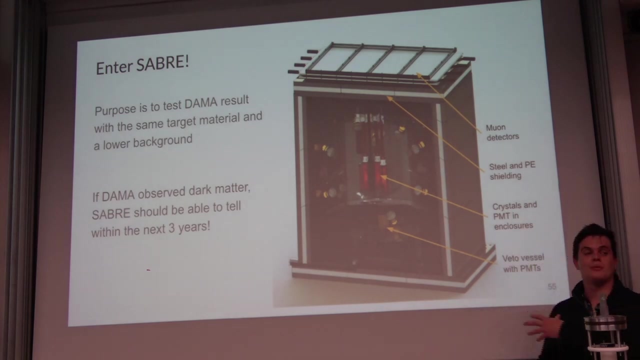 line, and this is the size of a person in height and basically the person if they held their arms out. yeah, so this is what it takes to be the best in the world, but then, if you're happy, for me, it is: what about the darma signal? so we are on sabre, which is an experiment that is being built to 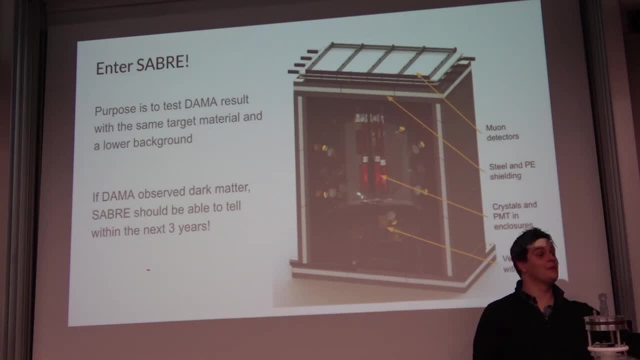 test the darma signal because if, if another experiment replicates the results, we can be pretty sure that it might be something like dark matter. so the whole point is we're using the dark matter to test the dark matter and we're using the dark matter to test the dark matter. 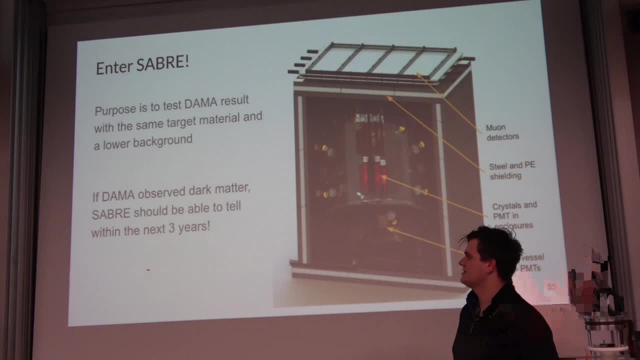 in the exact same material, which is sodium iodide, to test it. and, importantly, if the darma result is real, sabre should be able to find it within three years of operating underground, not three years in the next three years. oh, in the next three years. i'm not up to date with our current timeline. i. 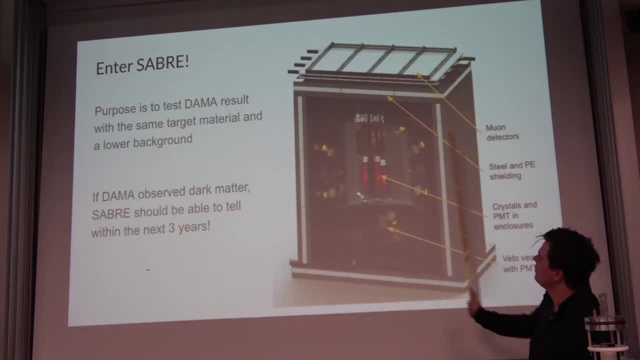 apologize. so just as a very quick overview of what sabre looks like, in the very center we have our sodium iodide detectors, once again in their big copper tubes, and we'll go through that in a minute. this is then surrounded by another uh detector which is filled with liquid scintillator and 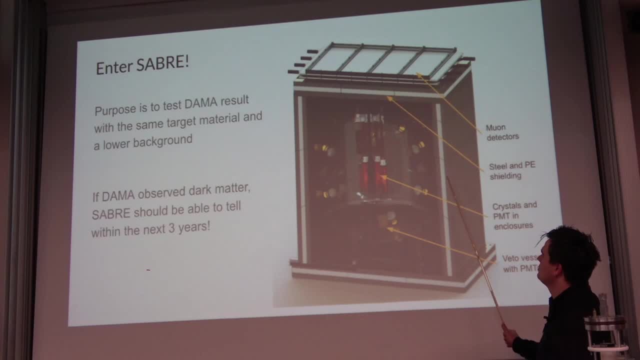 that's read out and we'll go through that again. and then, finally, it's shielded with copper- i'm sorry, with steel- all around it to block out radioactive particles, and we even have a muon detector on top, just like this one, except about a hundred times the size anyway. so if we go to 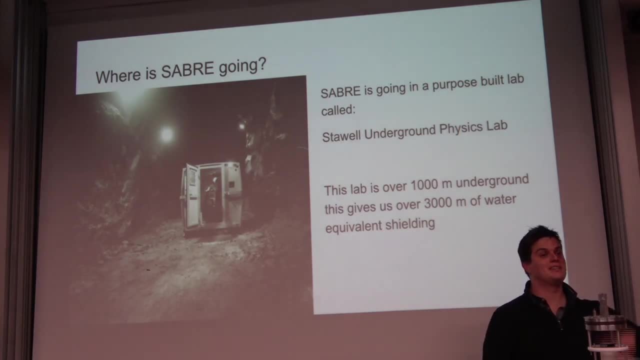 the next slide. where's sabre going? again, we're going deep underground, so we're going. sabre's being built in an old gold mine installed in regional victoria. um, this is the photo of where the lab will be. we won't actually be working in this space. it's not very big. our detectors, 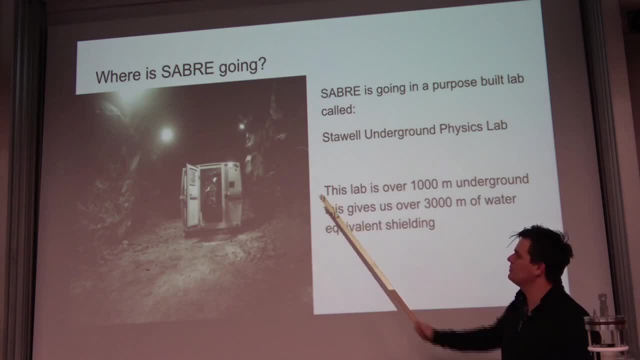 three meters by three meters by three meters. they're building a lab here right now, so we don't have a photo of it, but that's going to be built very soon. so by being over a kilometer underground we get nearly three kilometers of effect of what we. we measure our shielding in terms of water. 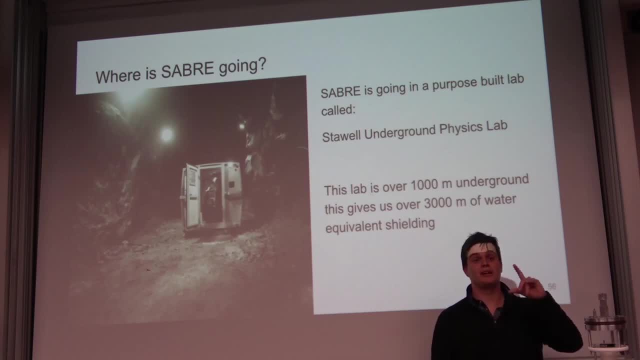 so by going a kilometer underground we've effectively got three kilometers of water on top of our experiment. that helps block out the muons, like we saw before. so instead of having them going that fast, as we were hearing it, the rate's much lower, so we can actually observe dark matter. 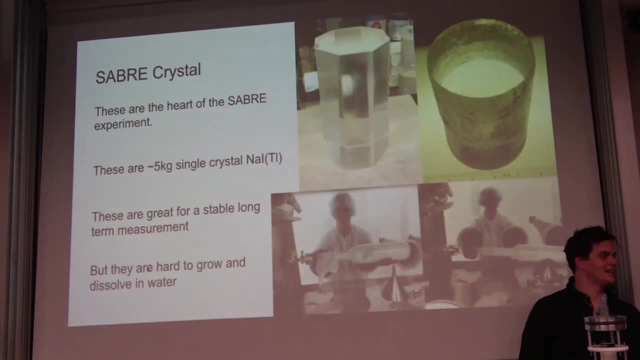 so on. to the like, the main part of the experiment, which for sabre, which is our crystals, um so we sabre- is using sodium iodide, like dharma, and we're using these big five kilogram single crystal bits of sodium iodide. so by single crystal here i mean it's grown so that it's one. 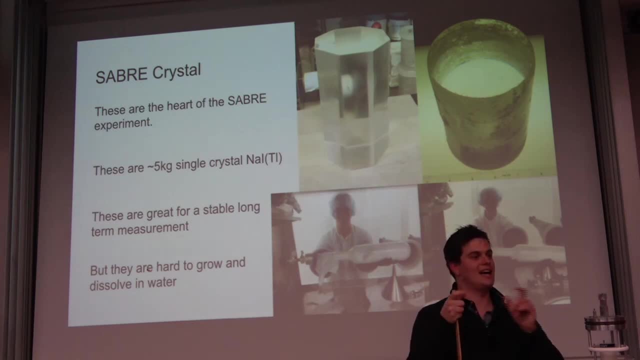 continuous lattice of sodium and iodine atoms together, so these things take months to grow and there's a lot of very, very sensitive handling um. so they're great for a long-term measurement because they're solid, but one of the reasons we have to be so careful is because it dissolves in. 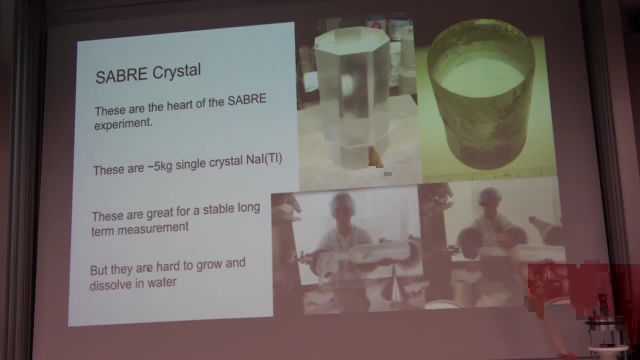 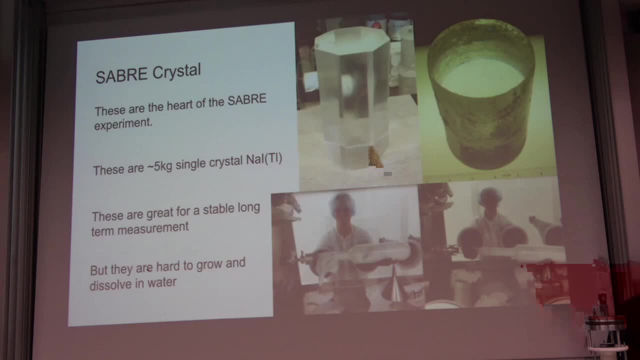 these crystals has to happen in a clean room, in a glove box, so we dress up basically like clowns to put on three pairs of gloves to finally be allowed to handle something. so in this case, this is the powder that ends up being used to produce these crystals. but this is how sensitive. 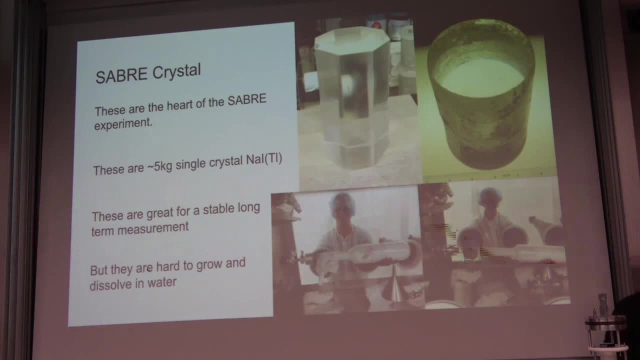 these experiments are that we have to do all this work to keep it pure, because, again, maddie was talking about one count per day, per kilogram. when you're at that level, everything is too radioactive. people are too radioactive. there's more potassium in. there's enough potassium in bananas to just. 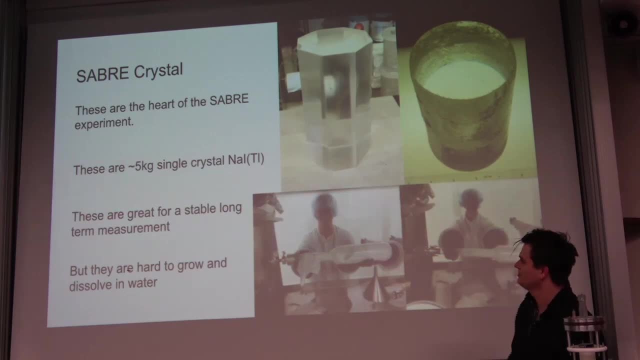 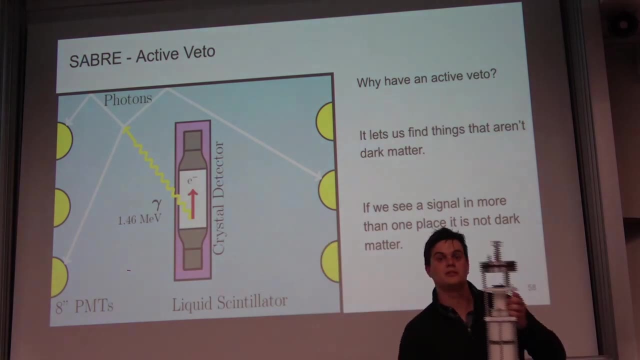 completely ruin our experiment if we left one in there with it. yeah, so our crystal. sorry, actually, i should have just before we're there. our crystal actually will get placed in this. this is a mock-up of its little enclosure and you can see, here we have our dummy crystal and then the two pmts that 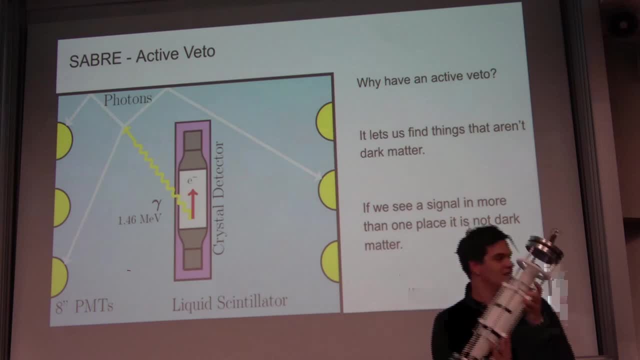 get paired with it. on either side this thing goes in a copper tube which then goes in our active veto, and the whole reason we have an active veto is that dark matter interacts very rarely, so it should only really interact once in our entire detector. so if we see something interact multiple times in multiple places, we can be pretty sure it's. 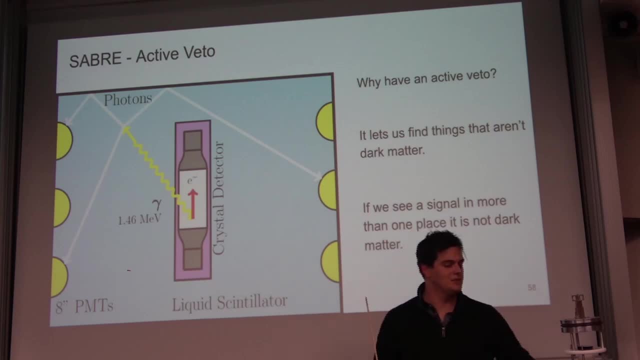 not dark matter, and that's why we have a giant tank of liquid scintillator that's covered with these pmts, these big hot um, these big ones that can see single photons, and this is it, doing exactly what it does. so we've talked about potassium a lot, because that's the thing that most looks like. 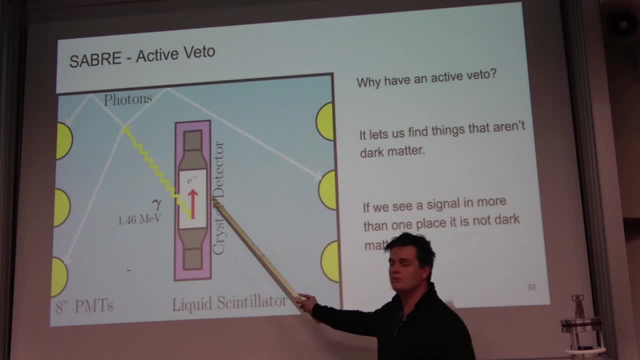 dark matter. if you have a potassium decay inside the crystal, we might think it's dark matter, unless we could also see this gamma ray that's produced and if it goes out, it interacts in our liquid scintillator. it produces scintillation light. we see it and we know that it's not. 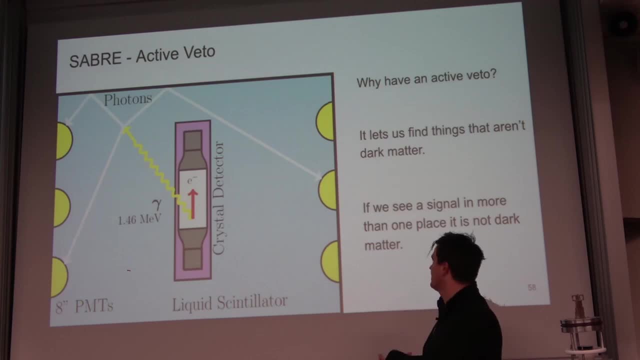 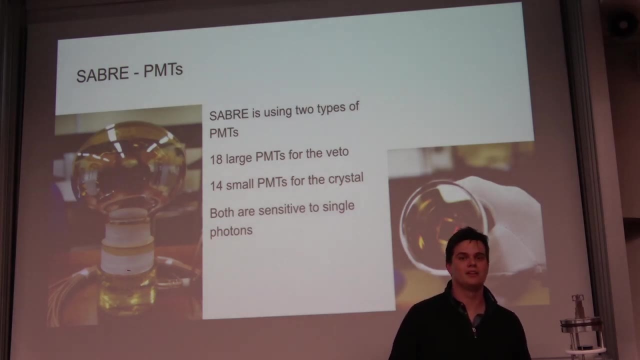 dark matter. we know that it was a different decay. okay, so again, i've told you. i go on and on about pmts. it's what i work on. i'm sorry, but i'm not really sorry. so we have our two different pmts. we have the big one for the veto and the much, much smaller one. so these are made to see single. 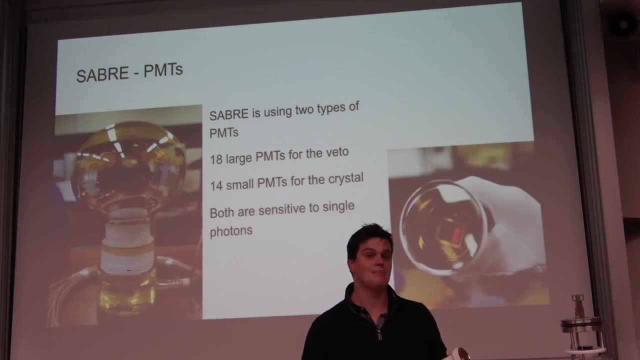 photons. because of that they are quite expensive and they're also handmade in japan. so the this one is like hand-blown, nicely blown glass and, yeah, i quite like them they are. they do look very nice. um, i guess if you're in person you can come up and have a look if you have questions about. 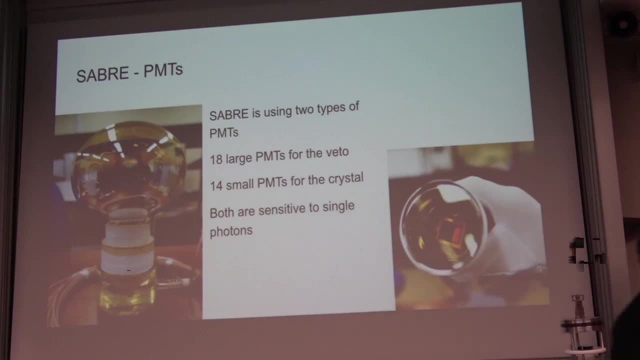 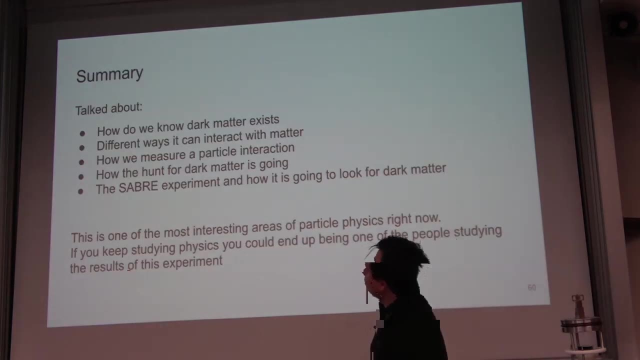 them, i'm happy to bring them up to the camera. you can also just not be as interested in them as i am, that's also okay. so i guess, to summarize what i've done today, we've talked about how we know dark matter exists, what evidence we have for it, the different ways that it can interact with matter and how we measure. 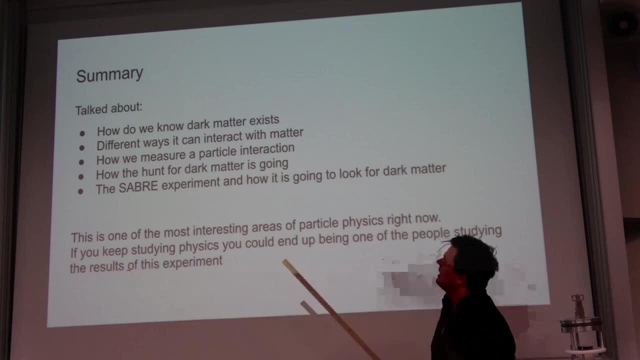 a particle interaction. i've gone on and on about that, haven't i? and then we have just how the hunt for dark matter is going. we have a result that looks pretty good, a bunch of results that say no, it's not. and then we have a result that looks pretty good, a bunch of results that say 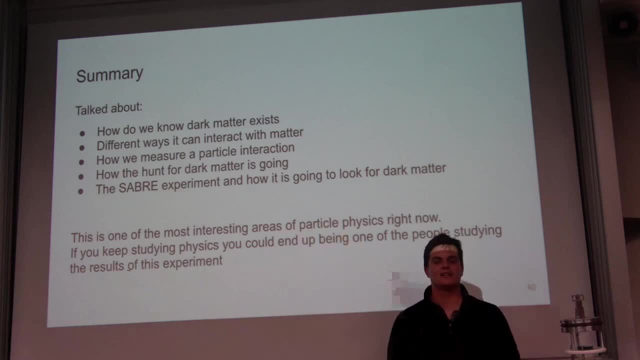 no, it's not. and then, finally, what the saber experiment is and what it's going to look like. so i just guess, to conclude, if this really interests you, dark matter is one of the things that interests physicists at the moment. it's one of the most compelling areas to work on in particle. 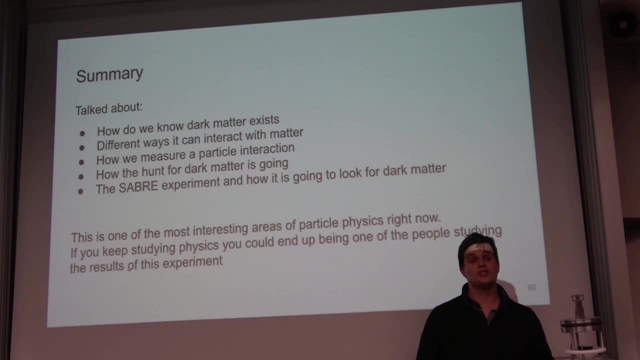 physics, and if you actually keep studying physics, there's a good chance you could be one of the people that helps us find the results from this experiment right. maddie said three years to get the first results. this will probably be going for five years, which is right about the time if you're. 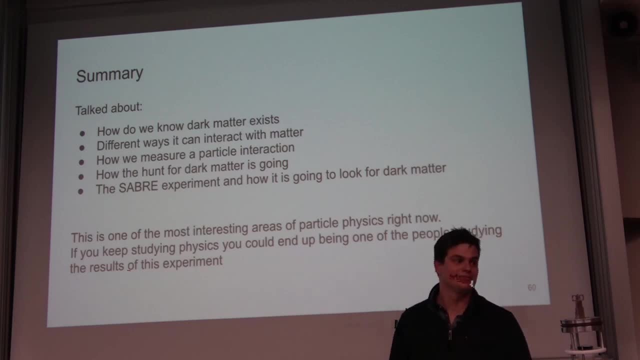 interested. you might be here doing a research project. so, yeah, you could be the ones telling us the answer to this. yeah, yeah, i think that's everything now. there's 55 questions on the chat. um, so i'll take question one from ben ben james. what was your question again, ben? 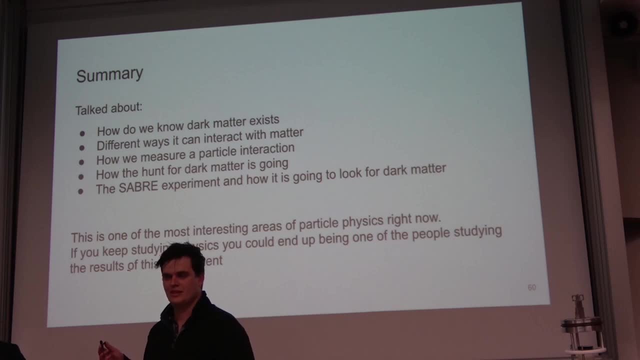 i'm not, ben hadn't asked a question, but i just thought if i'd asked ben to ask some questions, oh, you got me excited there, hey, actually. um, all right, dorothy nixon. all right, so the dharma results wiggle up and down, you know. 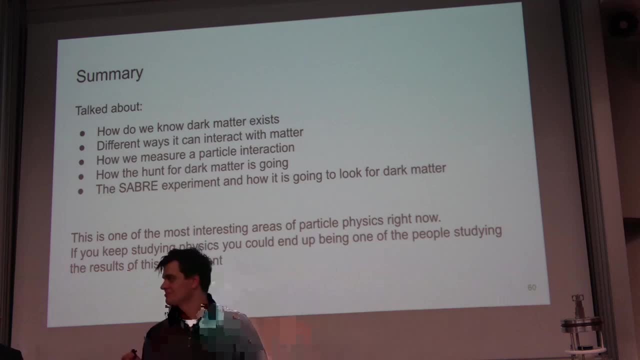 and they look like to expect yours to wiggle up and down the same way. i mean, isn't one in one hemisphere or the other. i'll hand this over to the expert on what labor should look like. yeah, in the same way that bill's spent the last. 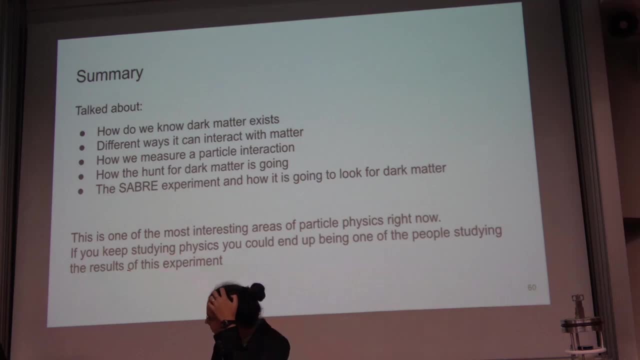 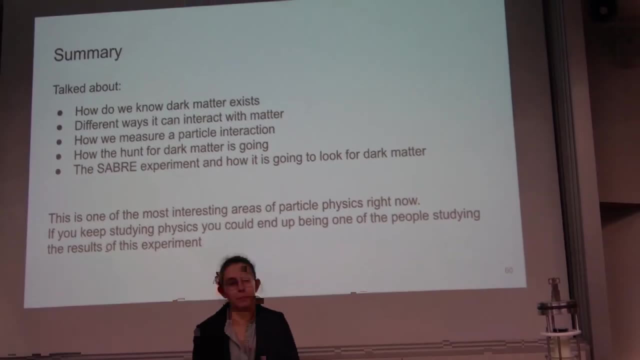 yeah, in the same way that bill's spent the last five years now almost let's not count how many years i've spent in a basement looking at pmts. yeah, i've been doing the same thing, the same thing four floors up, uh, trying to work out what. 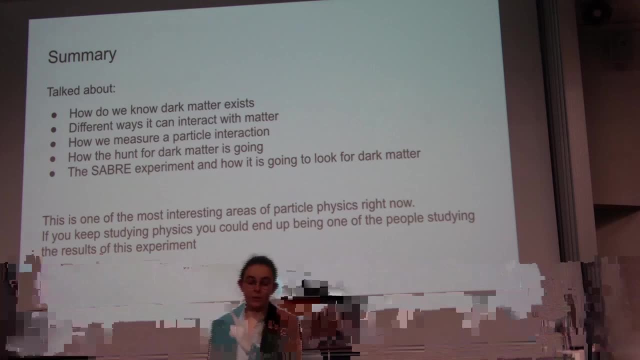 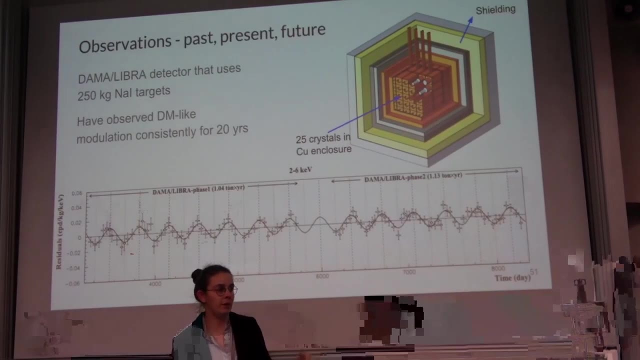 we're actually going to see in the pmt. so, rogers white, right, one of the really cool things about saber and, in particular, supple, is that we're in the southern hemisphere. all of those other detectors we're talking about are in the northern hemisphere. so remember, i said that we expect it. 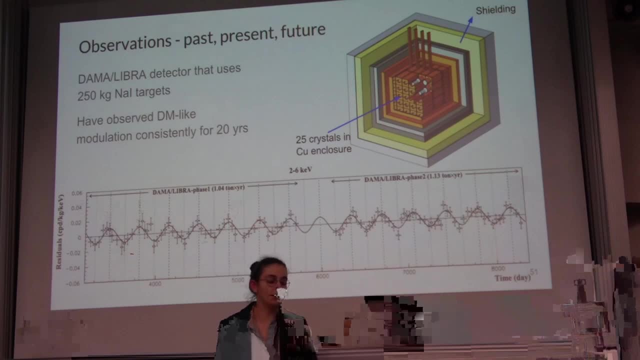 to be modulating or changing throughout the year. because the earth is going to be modulating around the sun, we can also have a lot of changes because of the seasons, right? so as one side of the earth is further away from the sun than the other, one of the things that we expect to change with 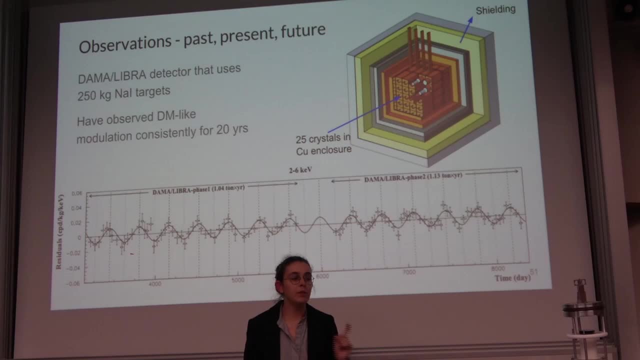 the seasons is the muon rate. so in the northern hemisphere, the number of muons that you expect to see has the same kind of look and feel as dark matter, so a lot of people have thought that this could be due to muons and not due to dark matter. however, in the southern hemisphere, 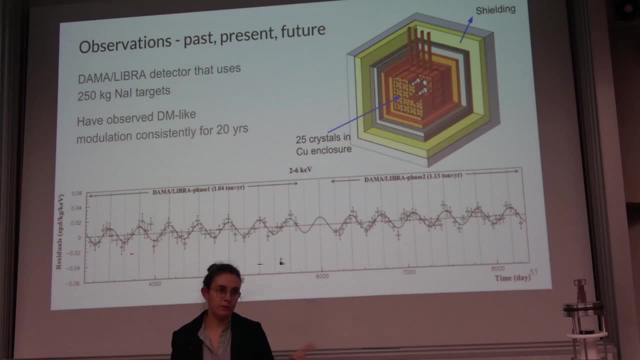 they're opposite. dark matter stays the same, but the muon shifts back to the northern hemisphere by six months. so if we see something in saber that looks like this but just shifted, we know that it's not dark matter. if we see something that looks exactly like this, then we know that it probably is. 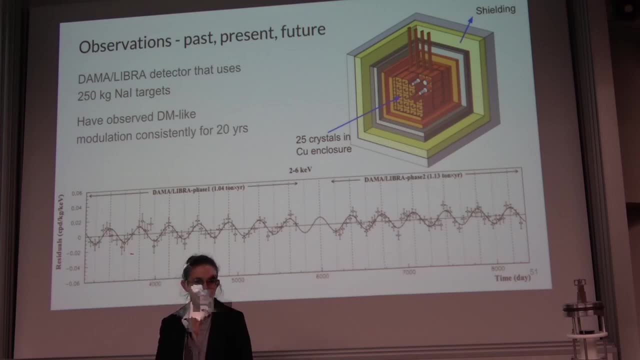 jacinta. oh, we need mike. i mean, we could get a person who spent four years of muons to do this, but are you happy? so, uh, i mean, it has to do with the way that the earth is tilted on its axis, right? so, all right, so i'll give you the microphone. 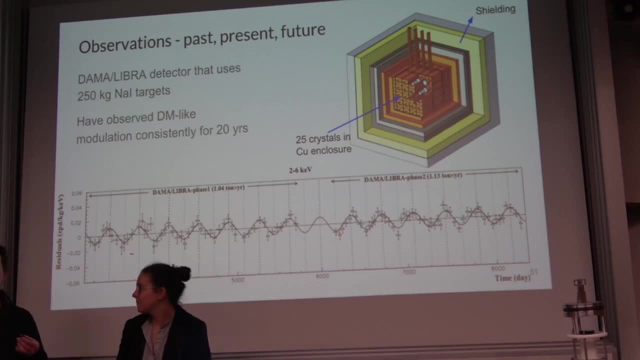 actually let me just pass it out. um, so it's because muons are produced in the upper atmosphere, so one of the things that affects them is the pressure up there. if you're doing chemistry is the same time as doing physics, you know the ideal gas flow, right? 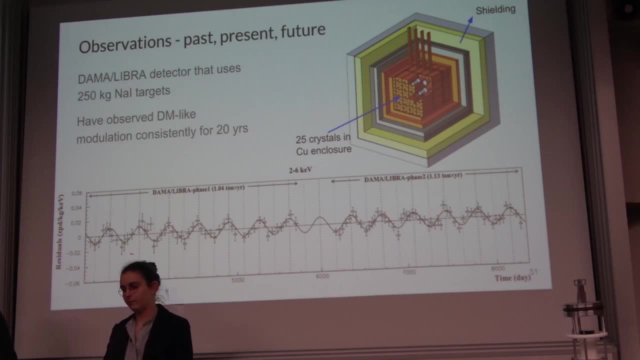 so if you change the temperature you'll change the pressure. that's true in the atmosphere as well. so in summer, which is what it is in the northern hemisphere, in july it's hotter, there's less air pressure. so the muons, the production rate, will change. so the point is, the muons change in summer. because where they're produced has different conditions. they're produced in a different part of the atmosphere, so you get more of them. so one of the things is the muon rate doesn't just fluctuate with temperature. whenever you have a thunderstorm come through all of the 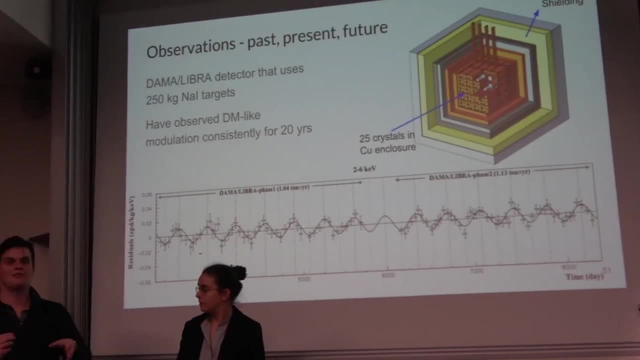 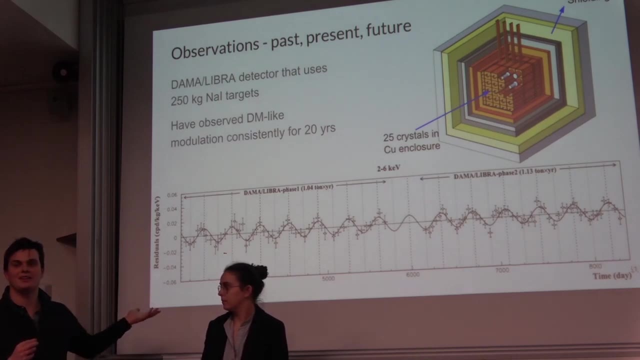 experiments that look for muons see the rate change, because you have a giant change in air pressure when a thunderstorm comes through. so that's why muons peak in summer when the app, when it's hotter in the atmosphere. i guess does that answer the. i'm hoping that answers the question that was asked. 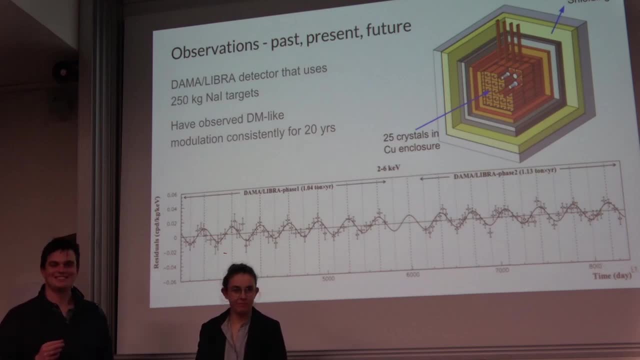 i didn't answer something else. we've clearly made everybody else experts. now they don't have any more questions. job is done. how far underground? one kilometer? yeah, a kilometer, but because you have to drive in, it takes about 30 kilometers of driving to get there. you just gotta go straight there like thunder beds. 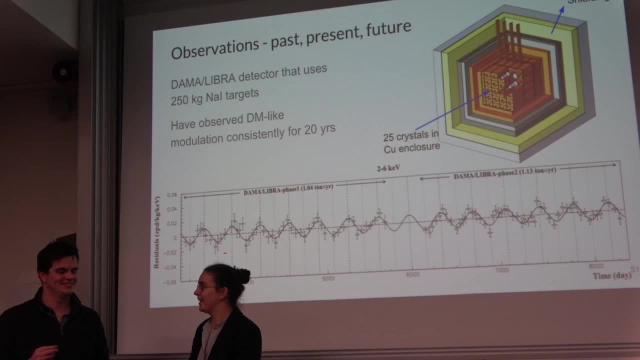 oh, i wish we haven't actually been yet. they had an official visit uh last week, week before, but they took the important people like politicians and stuff like that so soon. i personally can't wait to go see it, although in person we've got the air conditioning system, because apparently 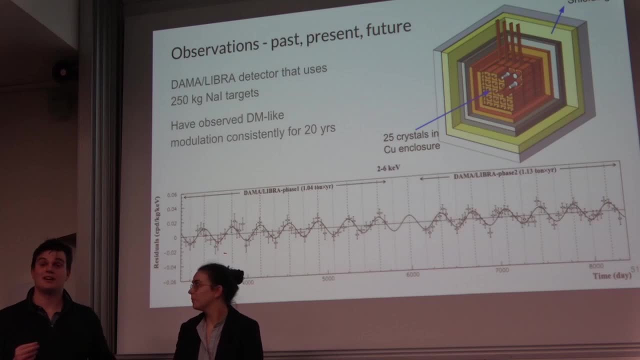 it's like almost 40 degrees down there, yeah, and you can see the most important thing about the air And because I was, you remember when we were talking about the clean rooms that we had to wear the plastic clown suits Because it's under a mine. you have to wear your proper high-vis. 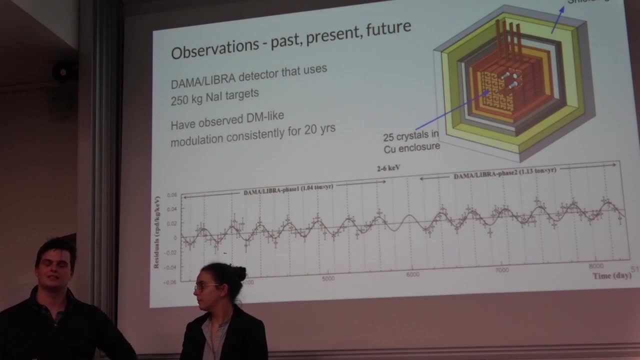 like mining overalls And then when you get there, you have to put your plastic clown suit over your mining overalls. So it's going to be unbearably hot down there. But please do physics. You don't just have to work in uncomfortable places. You can do cool things like visit the 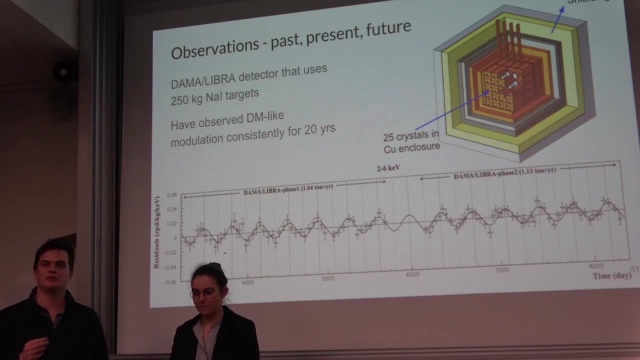 not evil underground lab in Italy where they do cool things under a mountain? Yeah, Yeah, What happens when the radiation contaminates the crystals? Good question, That's an excellent question. Maybe repeat it, Yeah, Okay. So the question was: what happens when the radiation contaminates the crystals? I guess, Yeah, I'm happy to take. 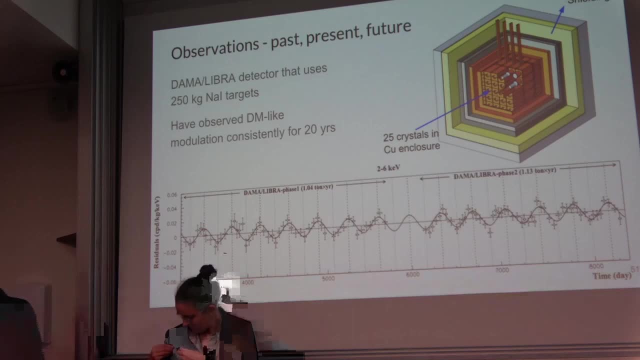 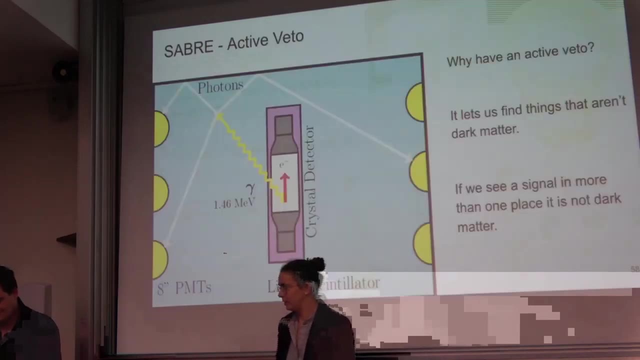 that one. This is the banana question. Yeah, The banana question. Do you want to get the active veto one up again, Just because that's got a picture of the? Yeah. So one of the things that I didn't mention about dark matter is that we kind of know 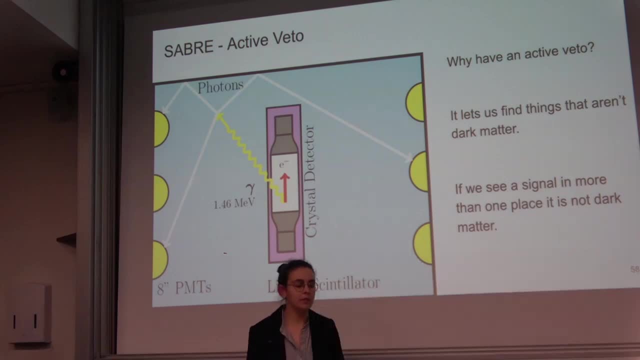 approximately how much energy it should have. So we expect it to be within around one to six keV. The problem with radiation is there are a lot of different radioactive processes that happen that have decay products at exactly that energy. So if you have them in the crystal like this, 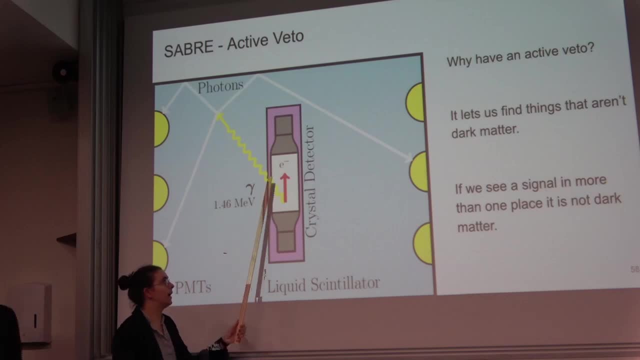 if we didn't have this liquid veto here, our radioactive decay would create, you know, an oscillation event and detection in our PMT and it would look almost the same as dark matter. So potassium in particular, which, as Bill said, we talk about a lot and we worry about a lot, 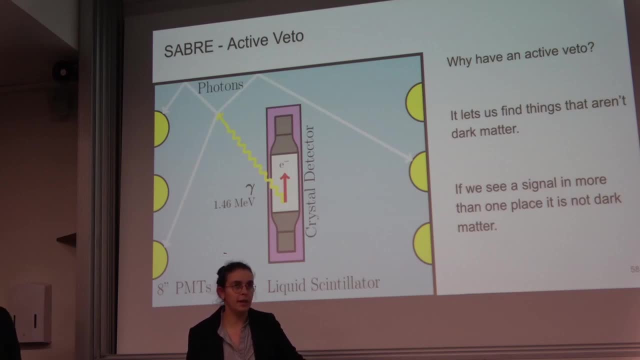 has a decay process that gives us a 3.2 electron, which is 3.2 keV electron, which is this guy here, and then our 1.46 meV gamma ray. Now this is problematic both because, as I just said, 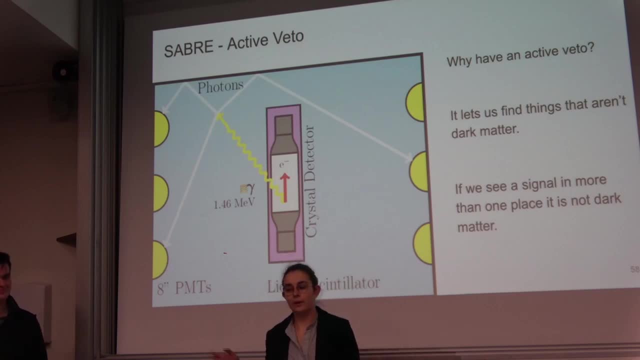 it's right where we expect dark matter to be. But also, I don't know if you have the periodic table kind of set up in your head, but potassium is right underneath sodium, So chemically the two are very, very similar. 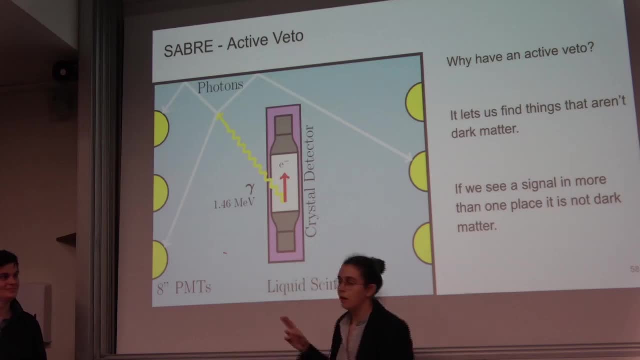 and it's quite easy for potassium to make its way into our ultra pure crystals. Now Roger said that this is the banana question. Part of that is because a lot of the way we measure radioactivity is in terms of bananas. So Bill said we can't have any bananas in the lab because 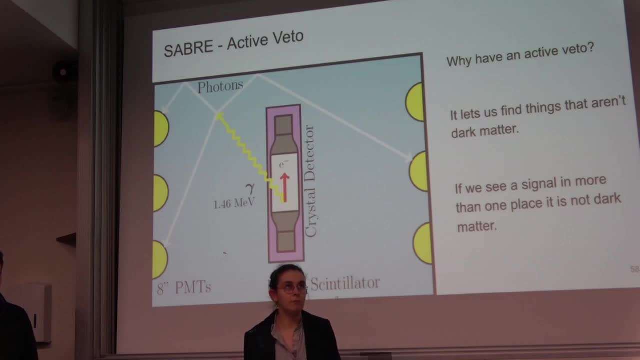 they're too radioactive. They're actually about 10 times too radioactive. So we have to grow these crystals so that they have 10 times less potassium than a banana does, because otherwise we would have our detector being overwhelmed by these kinds of radioactive events. 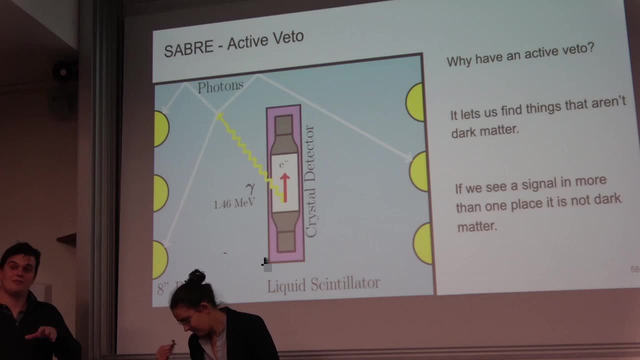 So I guess, just as Maggie was said at the very start, remember looking for a needle in the hay stack. If we have other radiation there, that's just basically adding more hay to our stack as well. That's the same size as the needles we're looking for. Yeah, Searching for a needle in a 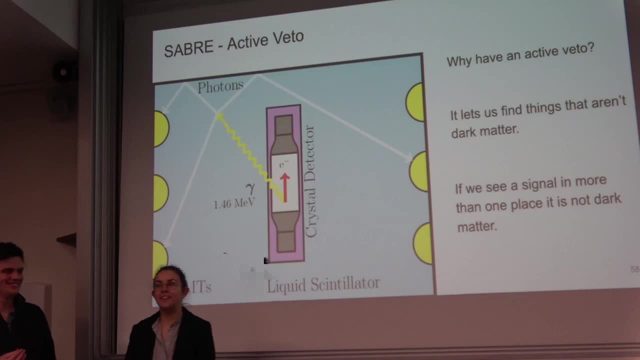 needle stack might be a more appropriate example. Yeah, because if it's a needle in a hay stack, it's a more appropriate example. So I guess, just as Maggie was saying, if we have other radiation there, that's just basically adding more hay to our stack as well. That's the same size as the needles we're looking for. 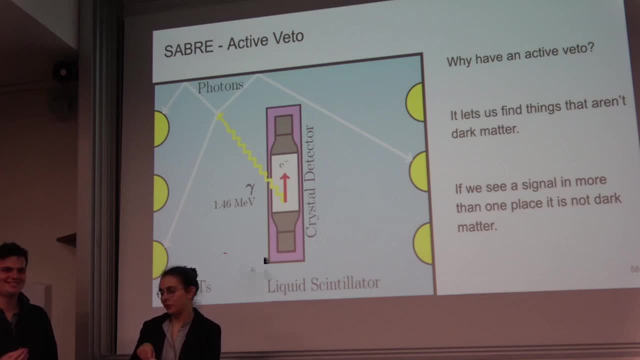 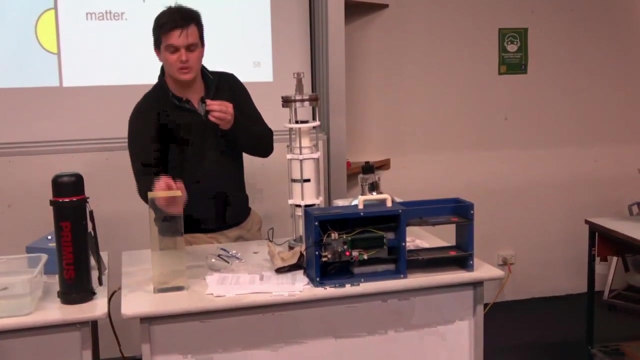 stack. you just put a big magnet nearby and then turn on a leaf load. I wish it was science. What are the exact materials that are used in the detector to detect materials In here? Okay, So the exact material. it is really a smaller sheet of plastic, almost exactly like this, but just cut much thinner. 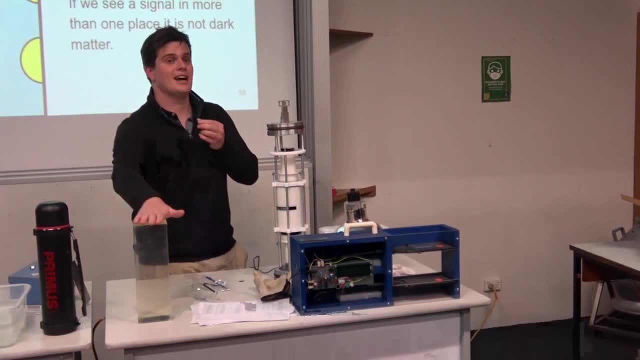 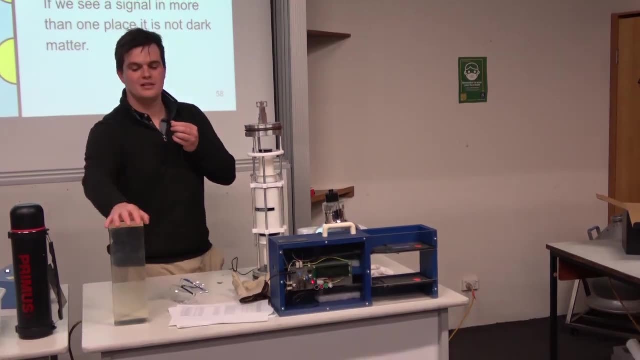 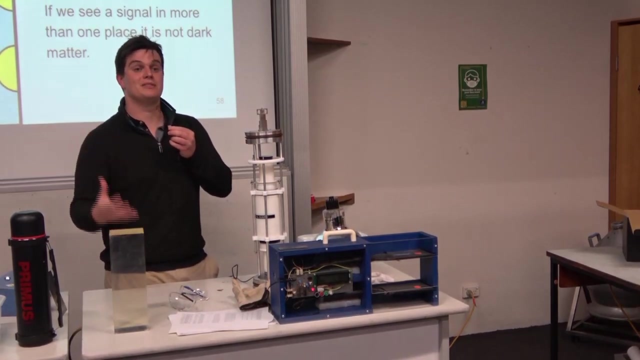 So people are always very funny about saying what the exact material is here, because it's hard to believe There's not a lot of buyers for it. but people do sell this. So typically it's a very long chain plastic with a few very rare elements- few rare elements- mixed in. 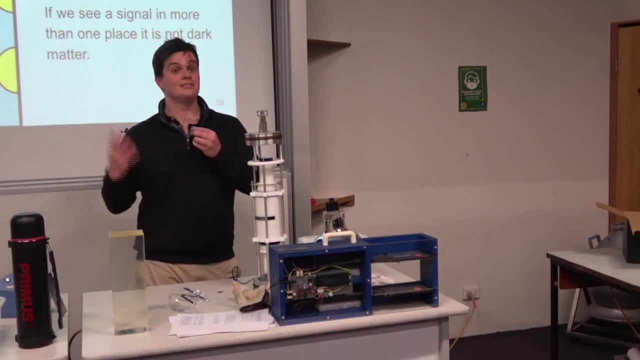 So for the most part it's plastic. for our liquid scintillator It's actually. it's called linear alkyl benzene, which just means it's a really long Chain of hydrocarbons with a benzene ring at one end. 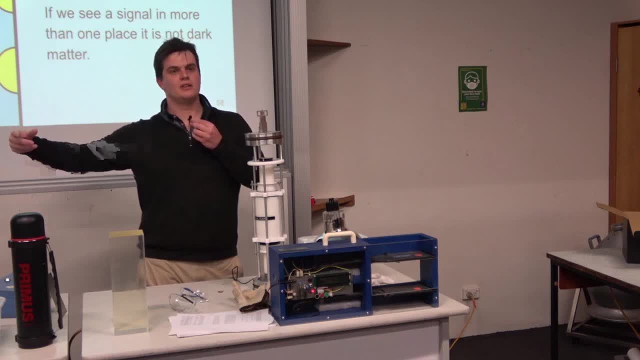 So it has the consistency of dish soap. So we have a 35,000 liter tank of dish soap arriving in about three weeks. Yeah, there's a scale to some of these things, But yeah, so inside here It's just a bit of plastic exactly like this. 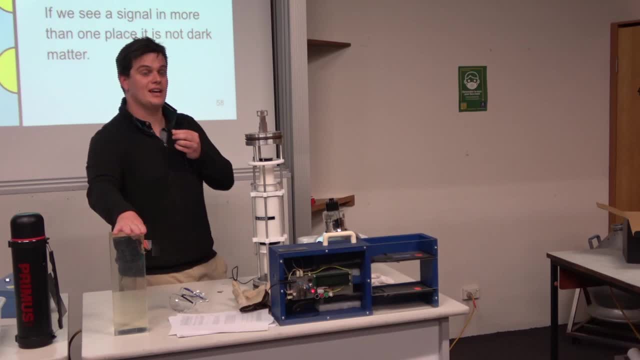 I can't tell you exactly what it is chemically, because they don't tell us what it is chemically. So how does it help to detect? So it works because it converts. when a muon passes through, it'll create, it'll knock a bunch of electrons loose in this. 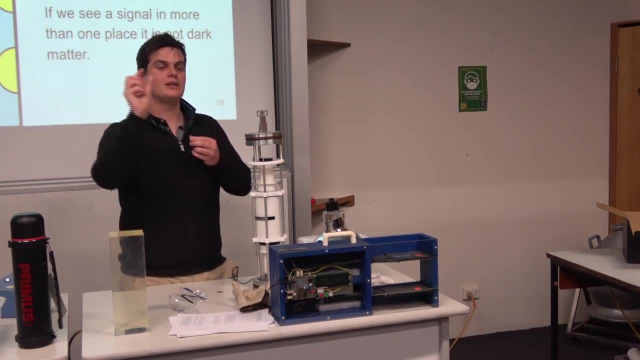 Right. And when those electrons are knocked loose, when they recombine with the space where they used to be, that will release some energy, And that energy is going to look like light, will be released as light, And then we can measure that. So that's why these detectors here. 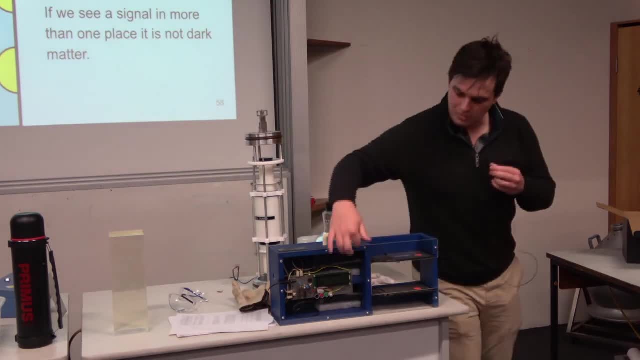 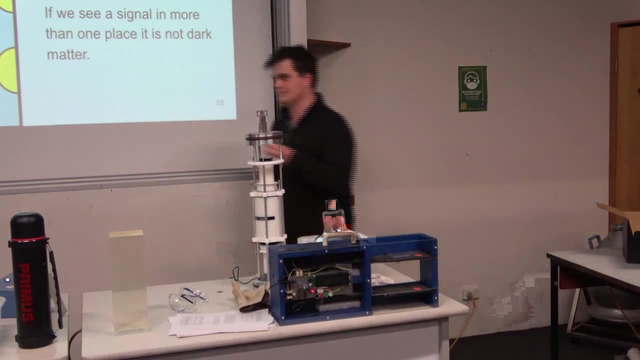 It's a bit of scintillator And then there's a very small PMT Under all this black tape here, So it's not a lot of light, which is the other thing. So it is pretty much the same as this. 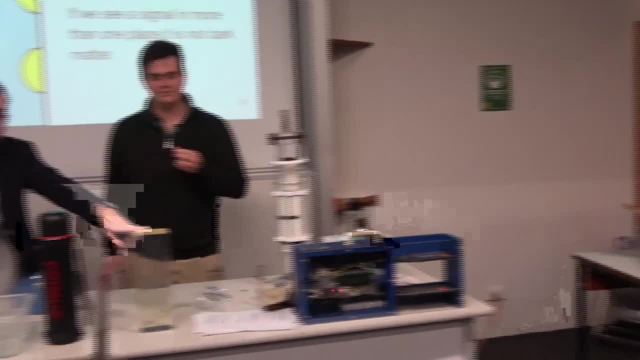 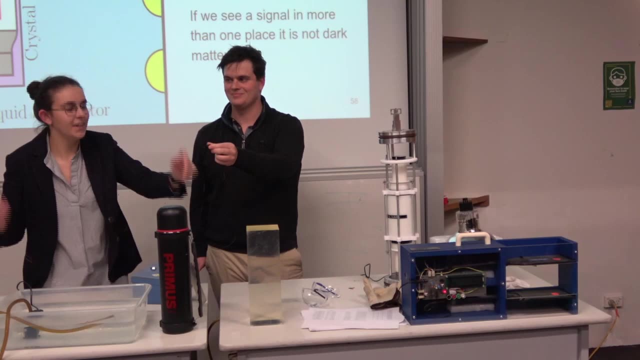 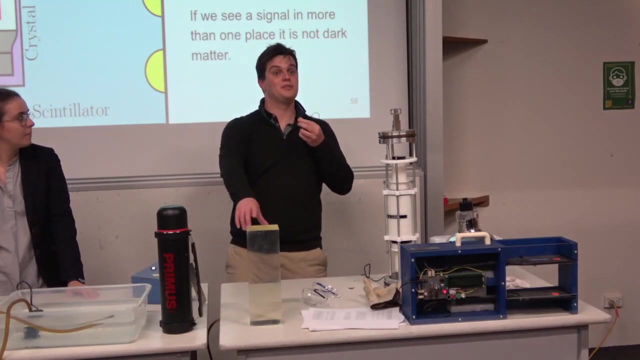 But the reason we don't see any muons moving through the sky is because the light that they're producing is microscopic- Nanoscopic, Yes, Compared to the light that's just from the general room by itself. So yeah, I guess, to see these things you have to put it inside not just one dark box, but two. 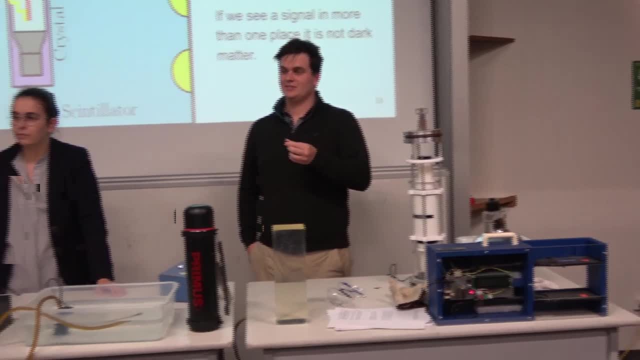 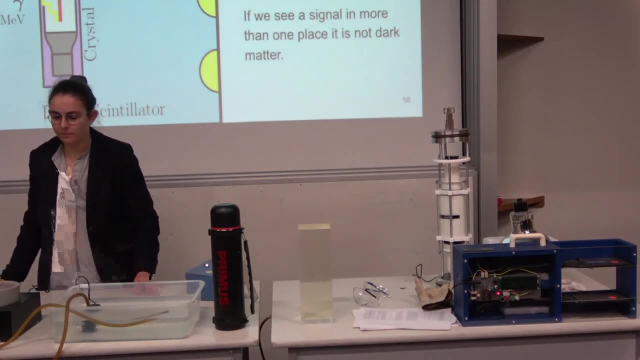 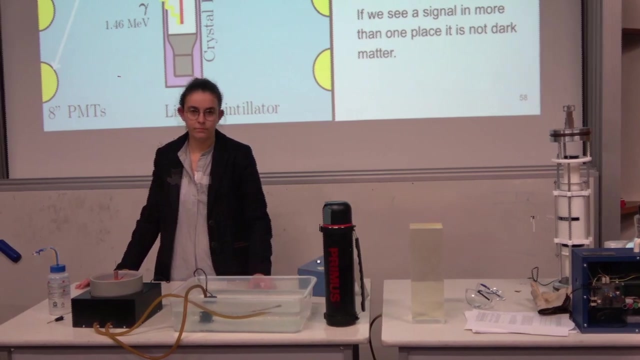 It's a beautiful thing, If I could. If we took that lump of plastic out into the bright sun, you would see an amazing purple glow in it And that's the actual scintillation of particles actually going through that. So we can't see that very much here. 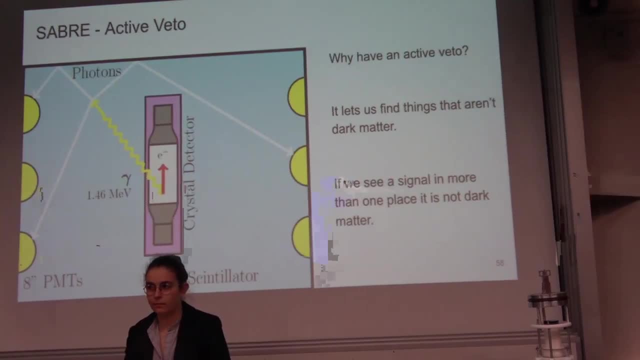 And then the black magic of what they do with the loading of these crystals is that often the glowing is not at an area that's sensitive by, say, those photomultipliers. So they put some other little dopants into there so that when the ultraviolet light is produced, it then in your level of physics you guys do, they do fluorescence still. 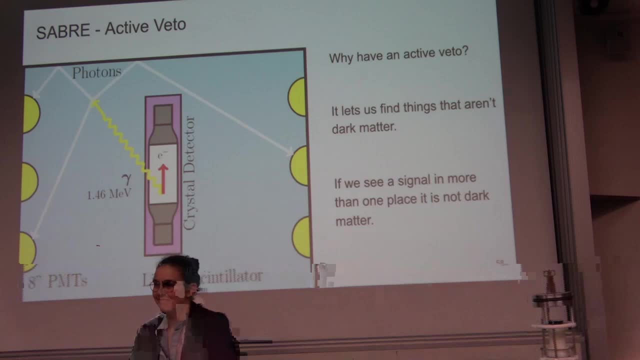 Well, we did that last week. Yeah, perfect, Okay, Okay, So, perfect. So the charged particle that comes through will liberate electrons. Those electrons lose their energy, And it's called scintillation, And it's called scintillation process. 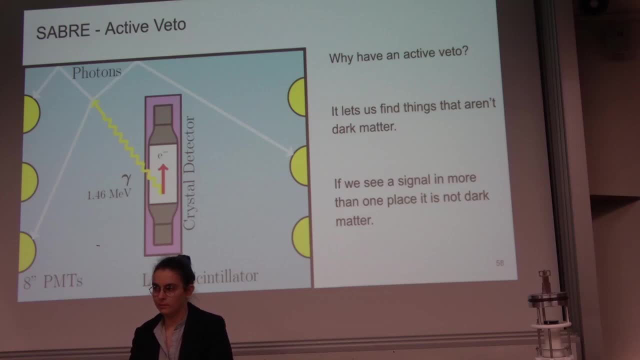 That then will often produce a color of the light that can't be seen, But then the dopant will actually absorb that light and then re-emit it fluorescently, probably towards the blue end of the spectrum or sometimes greenish, And then the photomultiplier on the front of that photo tube. that's what I was asking. 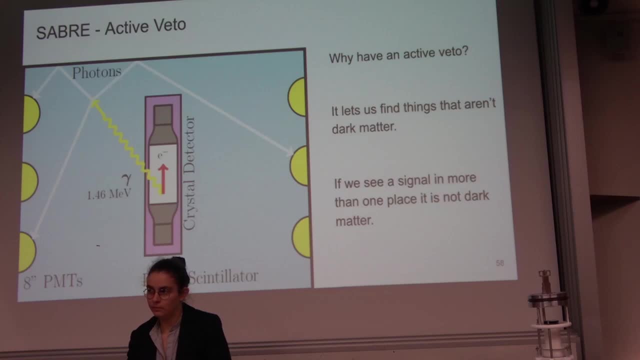 I don't know what. it's not cesium. obviously those ones. Is it The photo tube? The photo tube, The photocathode? It's not cesium, is it? Or is it cesium? It's not cesium. 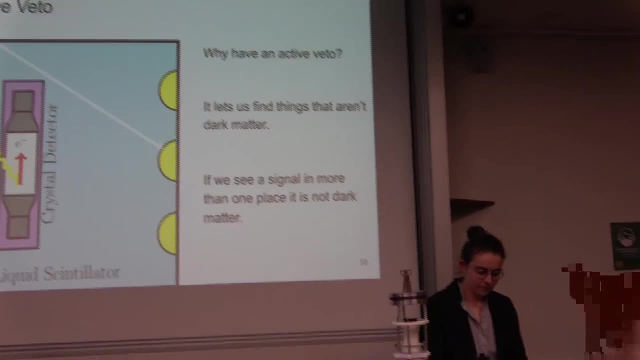 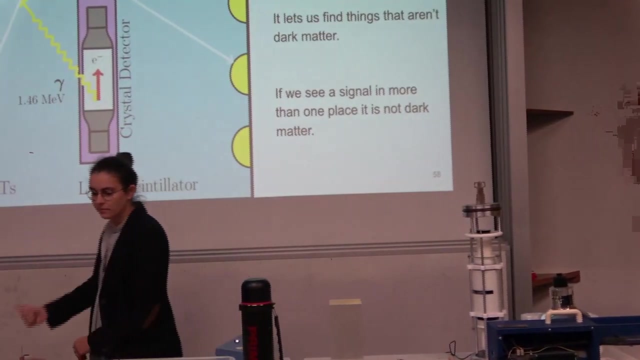 It's not cesium And it's a company secret. All right, Hamamatsu secret, Hamamatsu, bloody secret. We also have to be careful that they're not regular. Yeah, No, But see what will then happen. this is physics that you guys know. 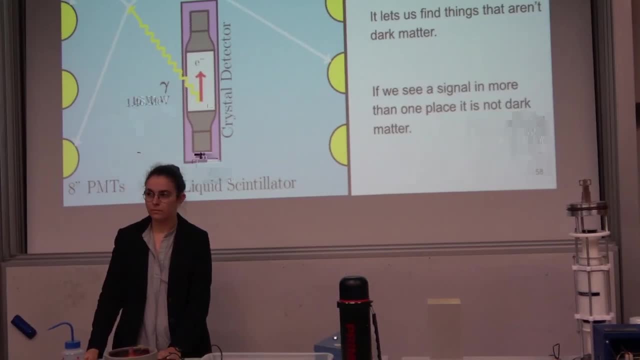 So now you've got a visible photon that goes through the front of that glass thing and liberates an electron from photoelectric effect- All the physics that you guys already have studied or will study at year 12.. Yeah, So there's the chain of events as Bill and Maddie described. it is the important thing. 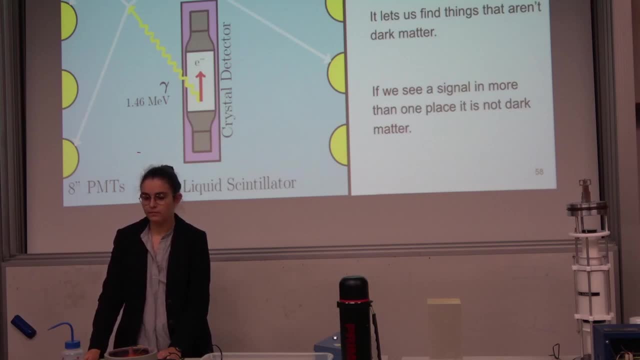 that you have some unknown particle that interacts in this crystalline structure, excites that structure, produces light. that light then travels into the photomultiplier, liberates an electron. that electron is then accelerated and then you get a pulse from that. 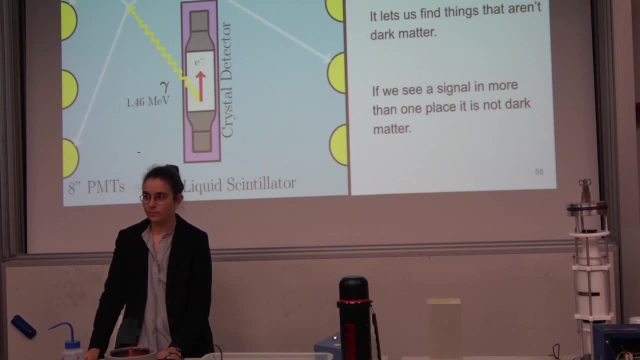 And all you have to do is study year 12 physics and then you'll be ready here at first year to go and play downstairs in that lab. They're beautiful devices And you know, the other thing is often in physics you think, oh, I got it invented last week. 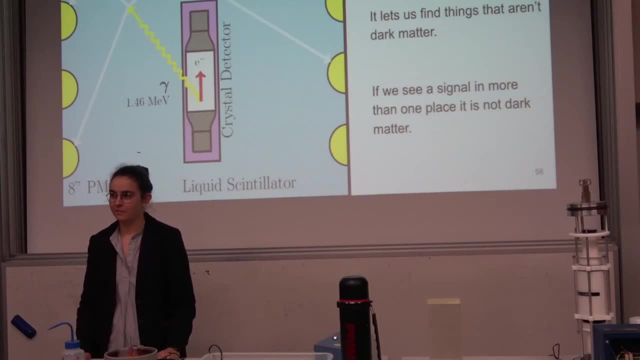 No, no, no, no, no. The sodium iodide: do you guys know when it was invented? Well, we read a bunch of papers when we were trying to grow really pure ones that came from the 1950s and 60s. 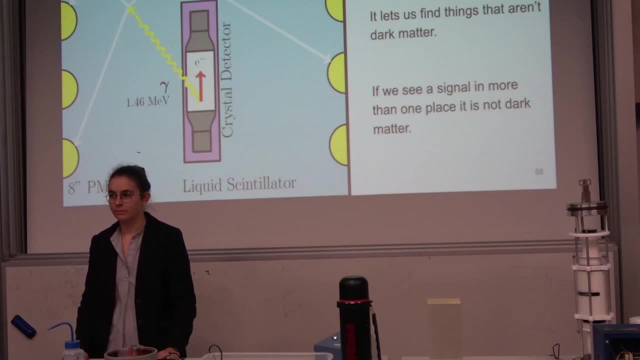 Correct: 1956, early 1950s, late 1940s, early 1950s. Yeah, So this is what's going to save the world. So the big advance we had since the 1950s and the reason they couldn't do this. 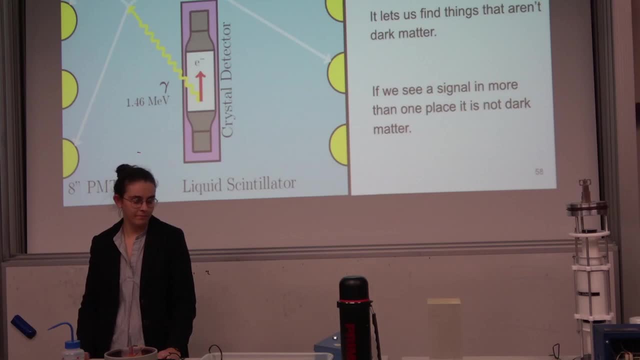 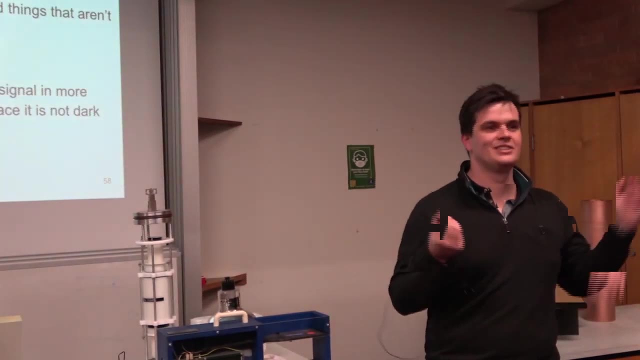 is that we have the electronics to measure it much better. So that's why I could actually show you the plot. they had there Previous experiments. they just went: oh, there's a pulse. Yeah, they could maybe measure the size of the pulse. 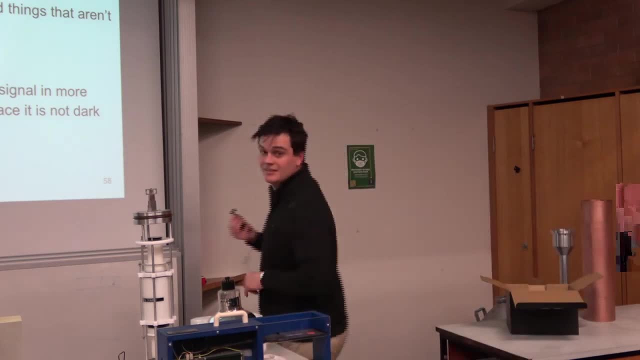 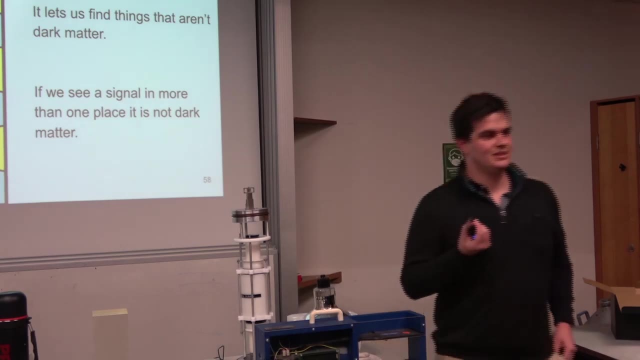 if they had a really good experiment. That was about it. That's right, 16 nanoseconds would have been unheard of. Yes, there was another question. Yeah, So you said dark matter didn't interact with electromagnetic force. Does it interact with weak force? 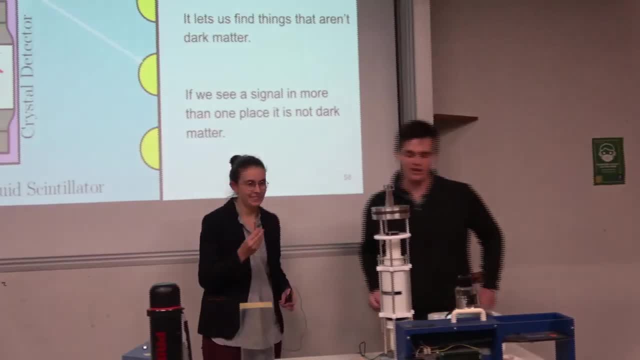 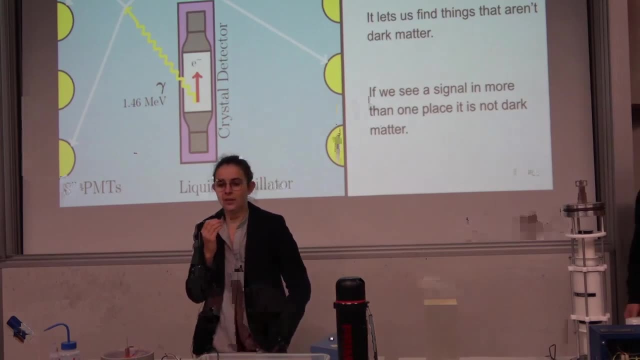 Again. hand you back to our dark matter interaction expert. Someone's been doing their homework, Yep. So the question for anybody playing along at home was: I said before that dark matter doesn't interact with the electromagnetic force, but does it interact with the weak force? 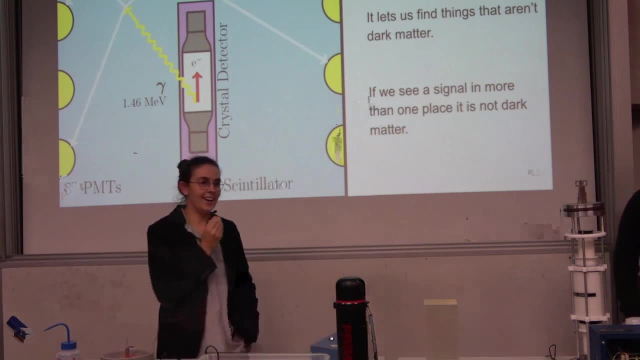 The answer is God. yes, I hope it does. The whole point of this experiment is: there has to be some way for dark matter and regular matter to talk to each other. Okay, Because we know that it doesn't interact with the electromagnetic force. 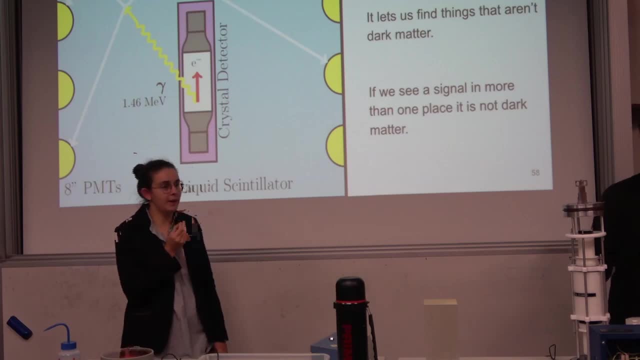 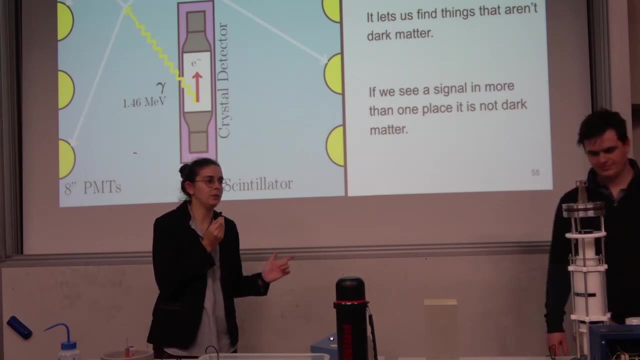 the one that we think of next is the weak, So we basically have to hope there's some kind of particle that can talk to the weak force, mediators that can then talk to dark matter and talk to the regular matter and allow them to actually have this scattering event. 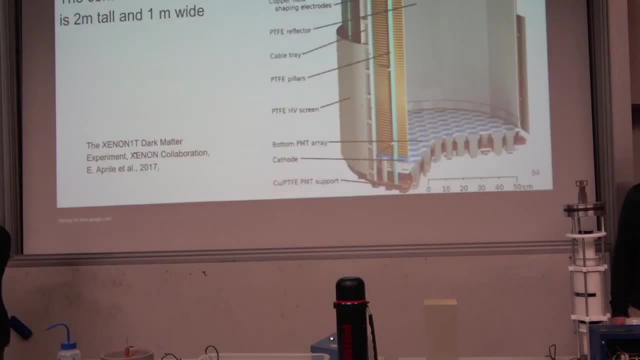 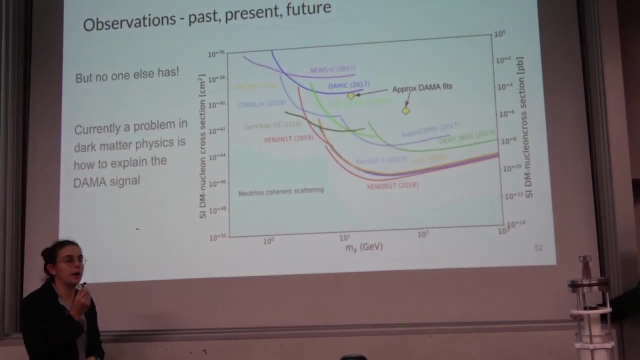 So the plot that I had up before of the cross-section here, and remember how I said that we think we know what, approximately what cross-sections we have. Part of the reason it's called a WIMP is because we think that it's weakly interacting. 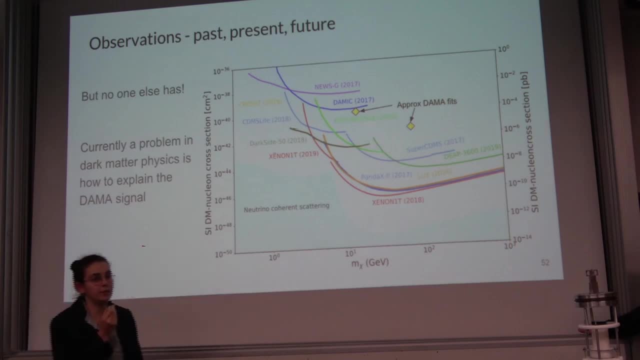 which means that it has a cross-section of around 10 to the negative 40 centimeters squared. So long answer short, I hope. I hope it interacts with the weak force And if it doesn't, would we see it? Not in this way. 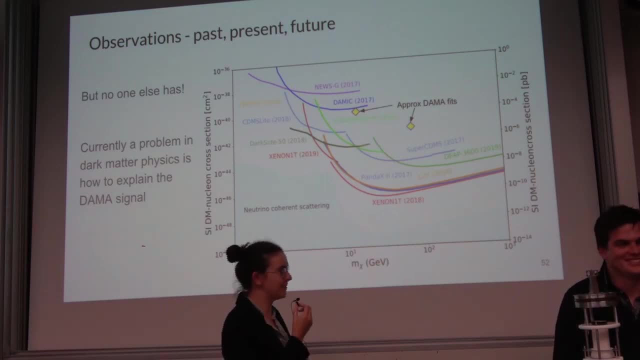 Yeah, now I'm panicking that I've banked my career on the weak force interaction. I think I've done it before. I think I've done it before And I'm not sure what it is, But I don't know. 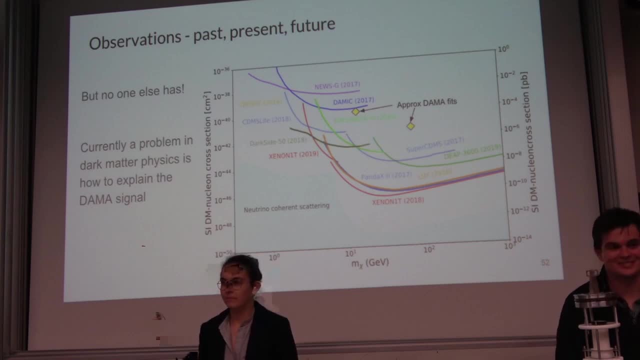 I'm not sure what the real thing is. I'm not sure what the real thing is, But there is nothing that I've done that's not used to it. There is nothing that I've done that's not used to it, And I'm sure that I can do it. 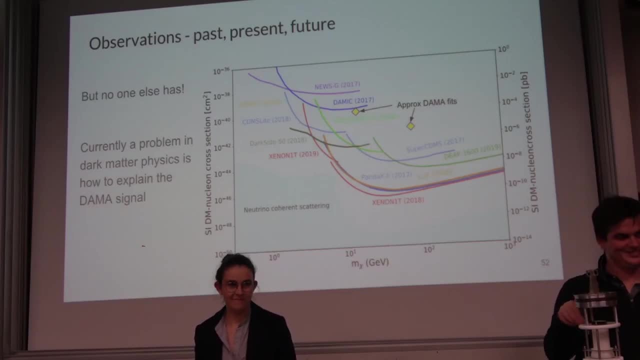 And I'm sure that I can do it. I'm sure that I can do it. That's really good, Maddie, I can yell, People can hear me. So, Maddie and Bill, thank you for a great talk. Thank you for those of you who came tonight. 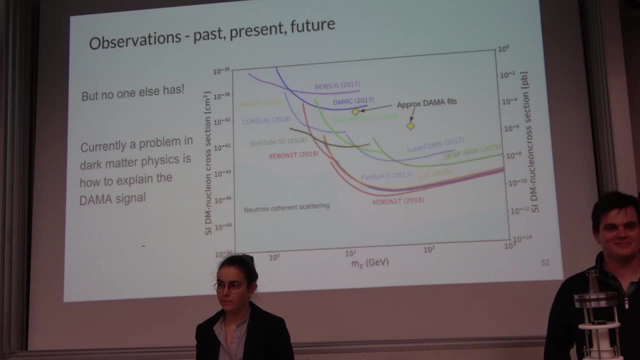 I think, Shuri, you win, coming the furthest from Frankston. Yeah, That's fantastic. Thank you for coming. thank our two speakers once again for coming tonight, and also a very special thank you to Steve, who is absolutely always there to set up any debate with me or anything else like that. so thank you, Steve, and good night everyone. 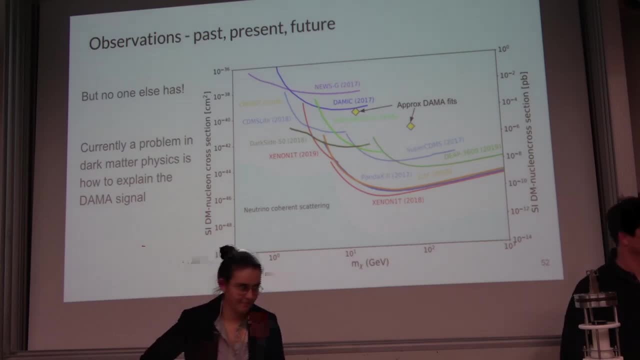 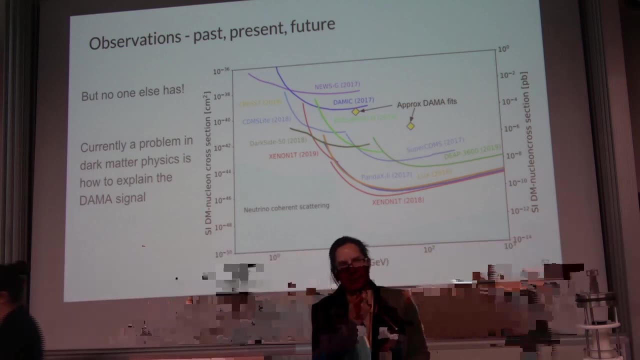 I was also going to say just really quickly that in two weeks time- thanks, in two weeks time- we've got a very special guest coming all the way from the University of Wollongong and she is talking about how we are going to combat radiation so we can get astronauts to Mars. okay, so she works on how we protect our astronauts and hopefully getting them to Mars. so she's making it all the way down from Wollongong, so I'd love for you to have as many people. 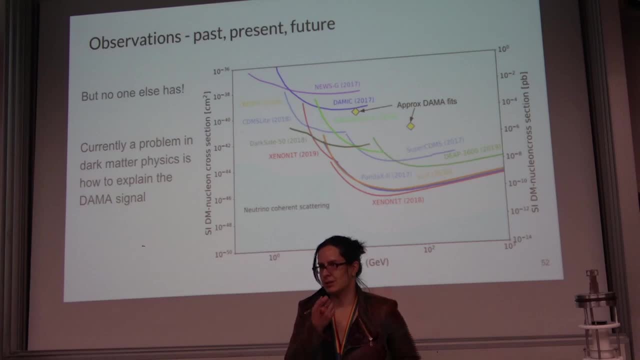 well, I don't think she's necessarily going to Mars, but she's just designing the suits so that we can get to Mars. so, please, please, come along, And it'd be great to have a full theatre, or, you know, lots of people come along, so if you can make it, that'd be great. 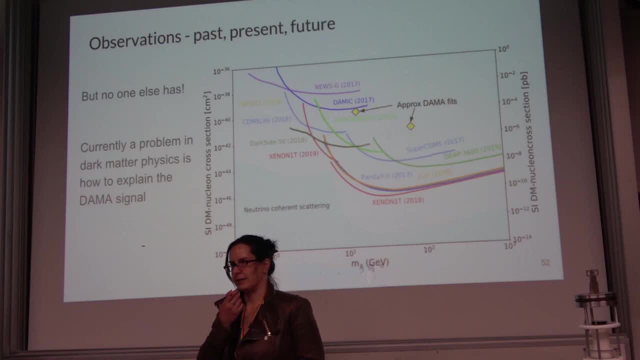 And they'll be up on the website. It is already up on the website, yes, and you can register now. Yeah, Cool, Ah, hang on, whoa, whoa, whoa. Ben James, Ben's got a question. 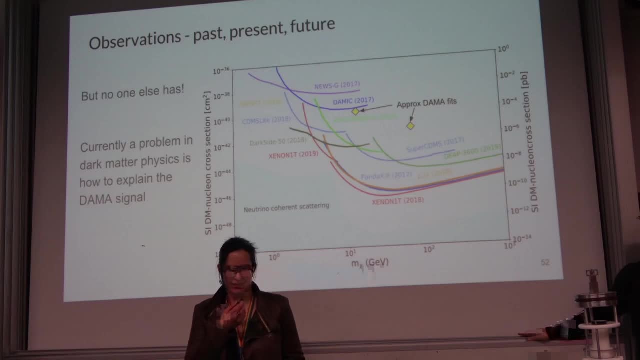